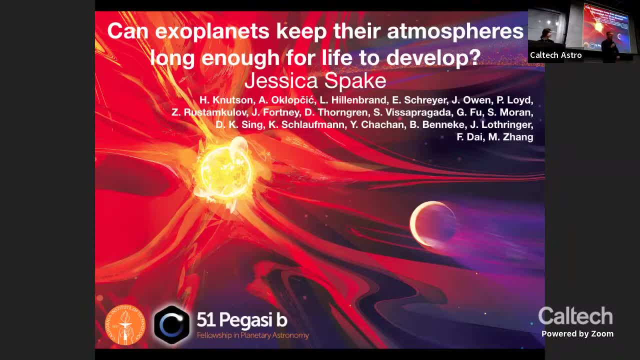 And he's going to talk about instruments like the LIGO instrument that occurred a few years ago and was awarded the Nobel Prize. So he'll talk something about, he'll give a presentation something about black holes, And then we have another series of events called Astronomy on Tap that take place at a bar in Old Town, Pasadena, once a month on a Monday night. 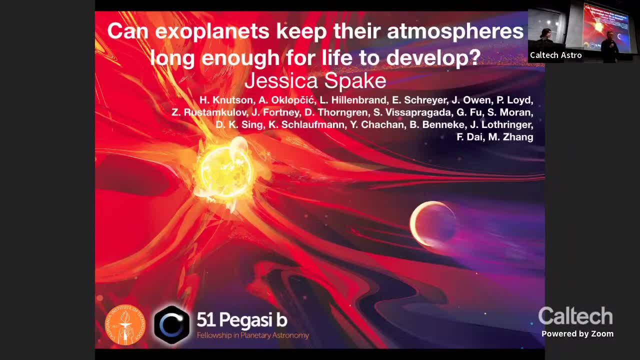 Our next one. I need to check the date. The next one? oh no, I don't need to check the date. I know the date: March 13th, Monday March 13th, so just two and a half weeks from now. 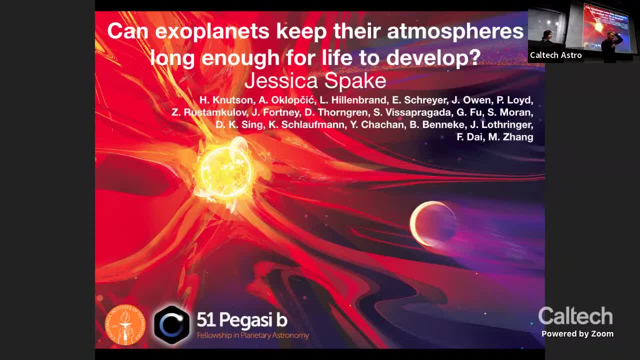 I forget the presentation topics, but I'll put out a poster about that, probably this weekend, So follow our social media or our YouTube page. No, it won't be on YouTube, So just on social media. I'm trying to make these occur live streamed on YouTube as well, but but haven't yet been successful on that front. 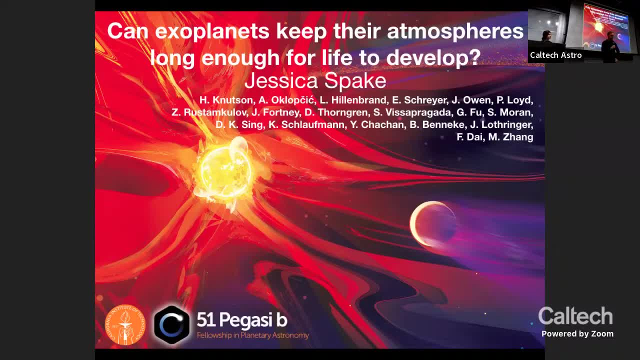 Welcome everyone. I think those are the bulk of my announcements. We obviously aren't going to be doing any stargazing tonight because of the torrential rain that we're encountering here in Southern California. We just, unfortunately, optical telescopes like the ones like the one in the corner, that will do a little demo of how it interacts, since we can't do a real demo outside. 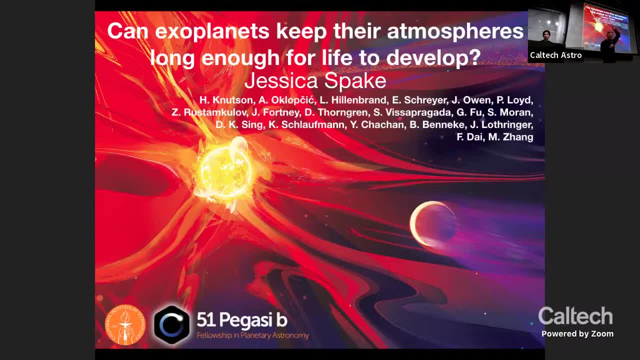 But we don't have telescopes that are capable of piercing through the clouds. You can look through clouds if you're using radio telescopes- certain wavelengths of radio waves, You aren't affected by atmospheric conditions, but that's not what we're looking at with our eyes tonight. 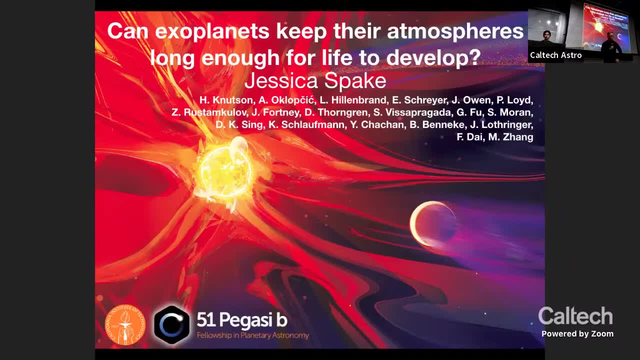 So So no observing tonight. OK, I think those are my my announcements, so I'd like to introduce our speaker. Our speaker is Dr Jessica Spake. She started in the UK. She went to Imperial College in London for her undergraduate before doing her PhD at University of Exeter and has been a Pegasi 51B fellow here at Caltech for the last few years. 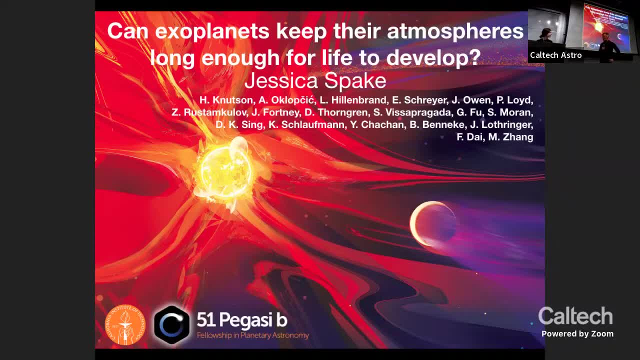 And tonight she's going to talk about Something I'm very interested in, which is how long atmospheres can remain around exoplanets and if they're there long enough for life to actually develop. So please welcome our speaker, Dr Jessica Spake. 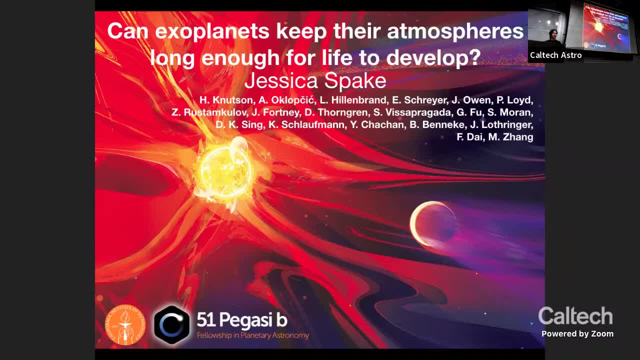 Thanks, Cameron. Thanks also everyone for bearing the torrential downpour that's occurring today. I really appreciate you being here. I don't have enough room on this slide to acknowledge everybody that I work with, but please bear in mind that all of this stuff 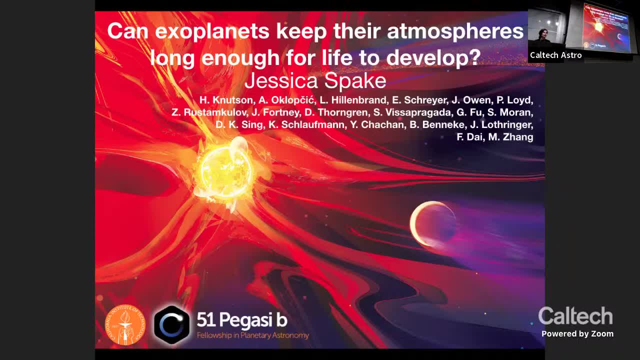 I'm about to talk to you about today. It's all done by huge teams of scientists. We never really do this work alone. There's never really one person that solves all the answers. So thank you to all my colleagues who helped me out with this. 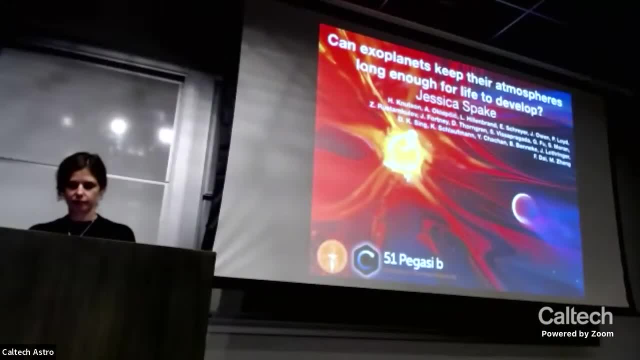 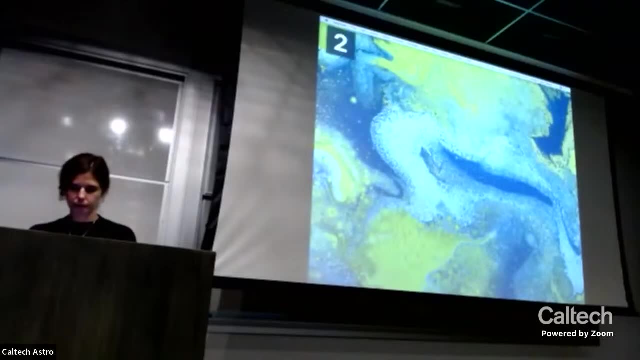 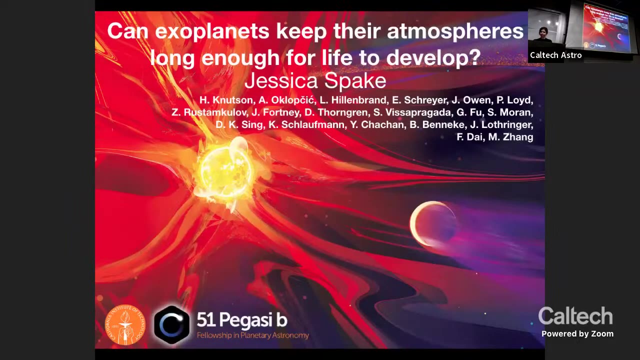 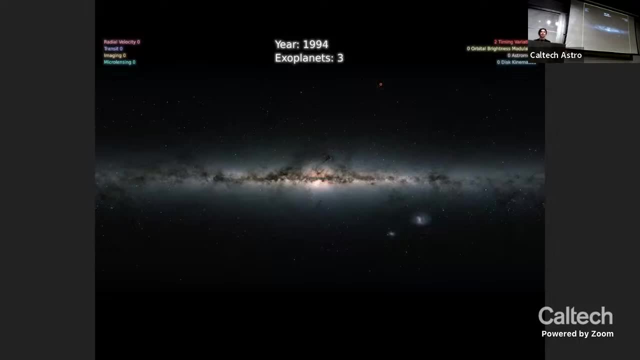 OK, OK, OK, Great. So I'd like to start By relaxing for a minute And giving us time to enjoy the sound of exoplanet discovery. The American Pronunciation Guide Presents ''How to Pronounce Exoplanets''. 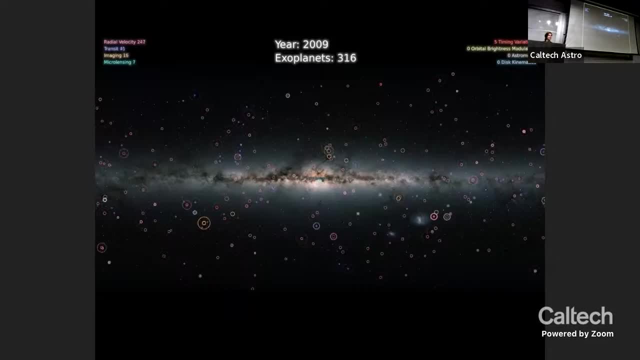 Out there orbiting around nearly every star in the galaxy are exoplanets. Exo means outside. These are planets outside of our solar system, And we found over five thousands of these orbiting around other stars, And we're pretty sure that most of the stars you see have at least one or two planets orbiting them. 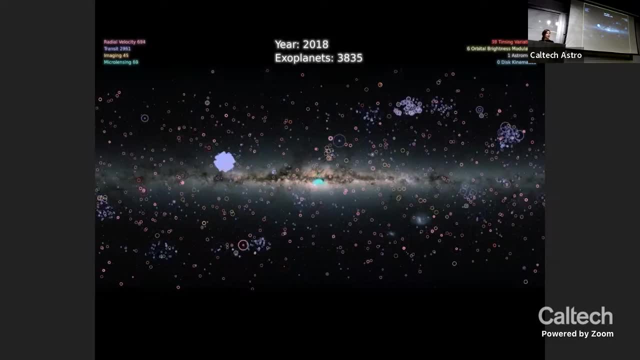 We find them with telescopes like Kepler, which focused on that purple patch of sky. you see, there And in this video, the tone of the sound you hear tells you how fast a planet orbits around its host star, and the size of the dot tells you the size of the planet. 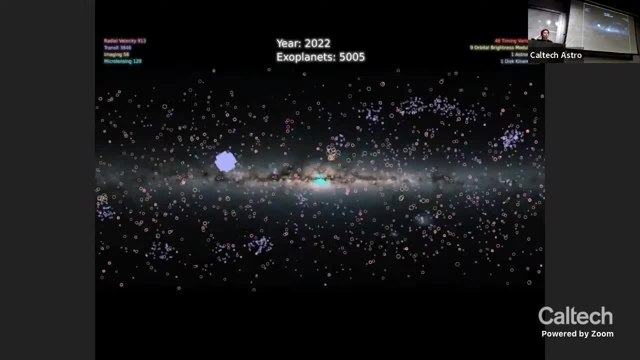 But for most planets that we found, that's pretty much all the information that we have. But the size of the planet and the length of its orbit doesn't tell you much about the story of an individual planet. It doesn't tell you what it's made of and it doesn't tell you whether that planet is habitable or if it ever has been habitable. 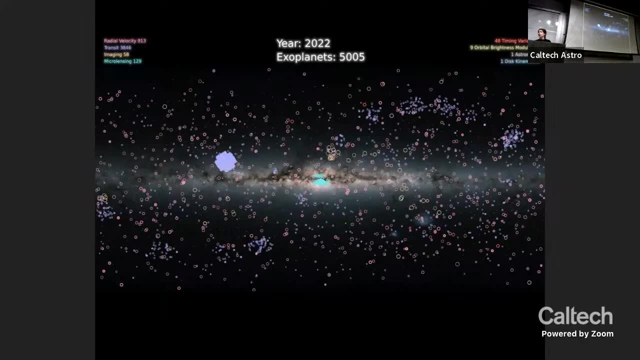 And for that we need to know the story of each of these planets. I can't Hello people online, So we're trying to piece together the story of exoplanets And we want to know if there ever has been, or if there will be, another place where life exists out there. 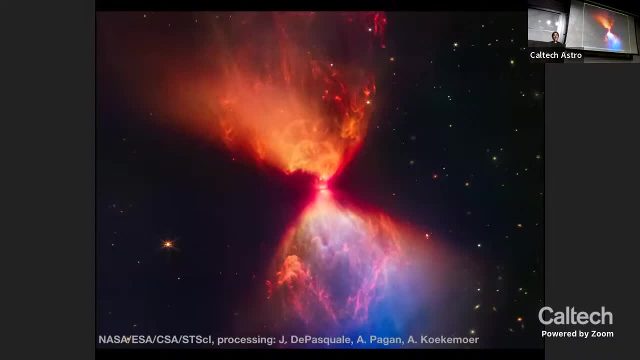 Planets start life in a disk around a young star, And this is a very violent place. In this image of a young star, the star is in the center of this hour: a glass of gas and dust, And that's what's lighting it all up. 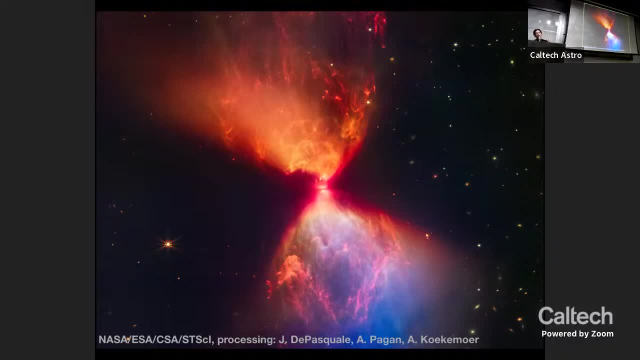 But right across the center you can see a dark band And this is an edge-on view of a protoplanetary disk And this is where planets are formed And right now we're trying to understand around which kind of stars and in which kinds of protoplanetary disks. 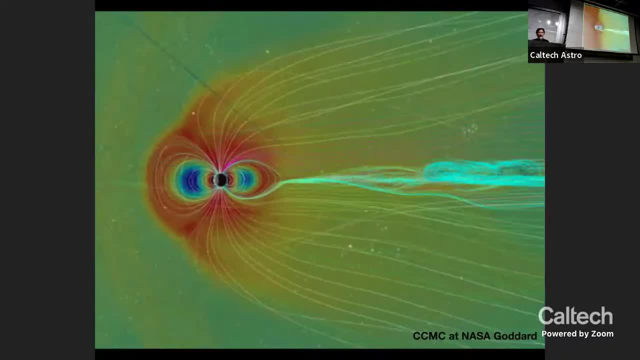 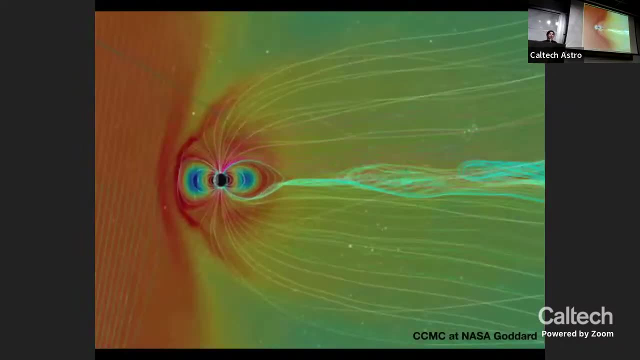 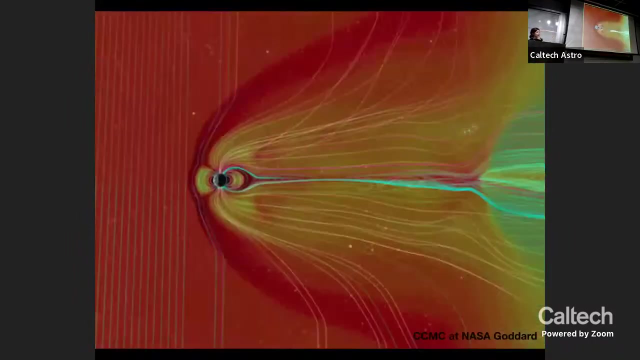 do, which kind of planets form, And once they are born, we need to know the rest of the stories, Especially because, even for older planets, space can be a violent place still, Especially for the atmospheres of these planets, And that's because this acts as the interface between the planet and the rest of space. 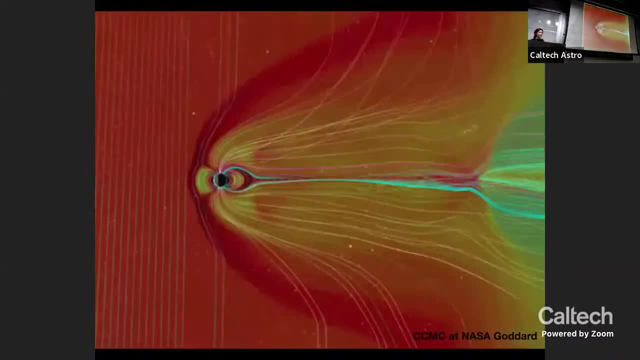 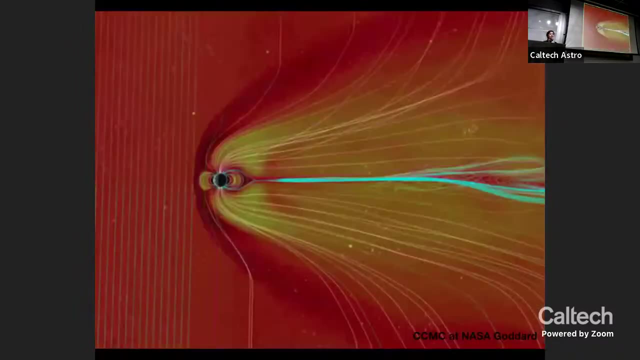 Now atmospheres are affected by magnetic fields. They can be affected by giant impacts, like the one that formed the moon around the Earth, And they're also impacted by the star. Now the star can emit these very strong winds and very strong radiation. 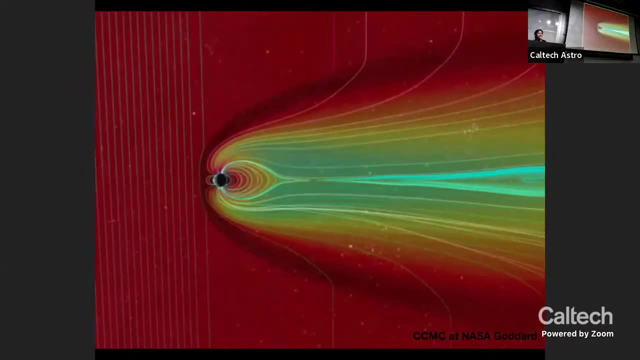 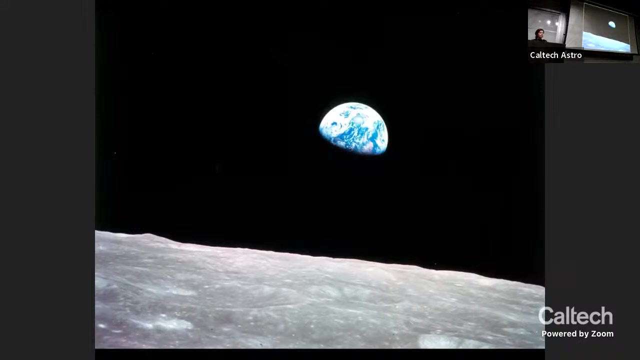 And this can escape the atmosphere into space. And this is what I'm interested in. I want to know how long can planets hold on to these atmospheres in these pretty tough environments? The Earth is a beautiful blue color because of our atmosphere. The atmosphere gives us enough pressure at the Earth's surface. 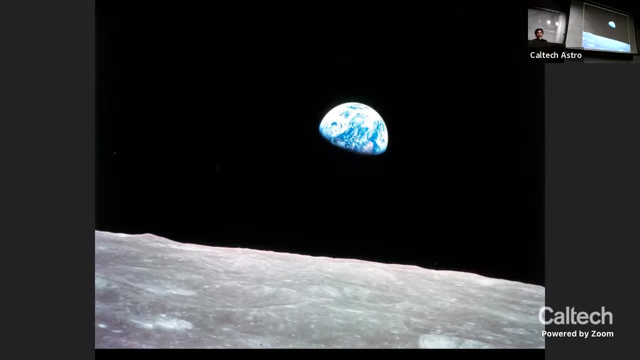 to maintain liquid water oceans. If you compare this to the bare rock of the moon at the bottom of this photo, which is airless now, this moon is the same average distance away from the sun and yet it's completely lifeless. There's no water on the surface. 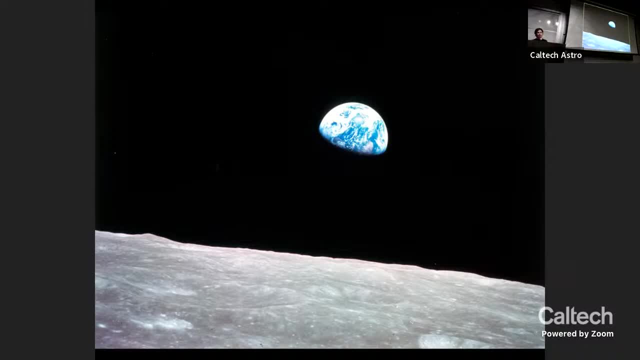 Some people consider this the most influential photo ever taken, First shot of the Earth rise on the surface of the moon, taken by the Apollo astronauts in 1969.. I struggle to express how moving I find this image. I love the contrast between the Earth and the bare rock. 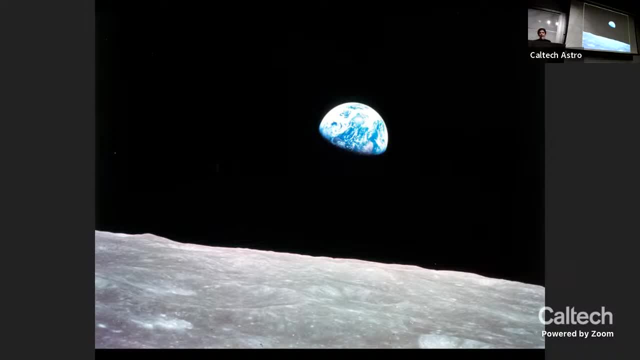 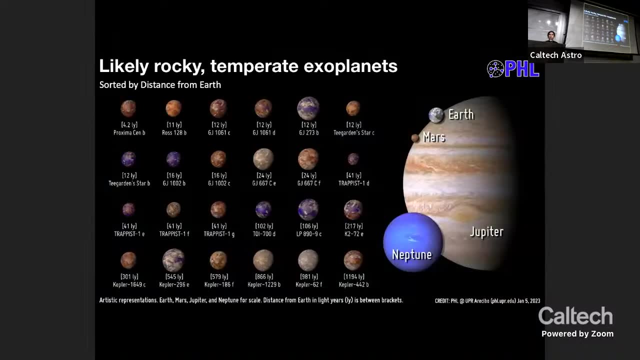 Our home looks very inviting but also very fragile. We don't know if there's anywhere else in the universe that's this beautiful. But since the end of the last millennium we've made some pretty extraordinary discoveries. So in 1991, the year I was born, 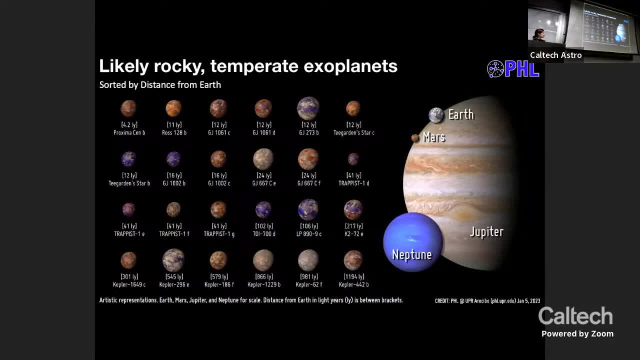 we didn't know of the existence of any exoplanets, But now we have over 5,000.. I'm really just getting started, because we think there really is a planet around every star in the galaxy. So here are some artists' impressions of some of the exoplanets. 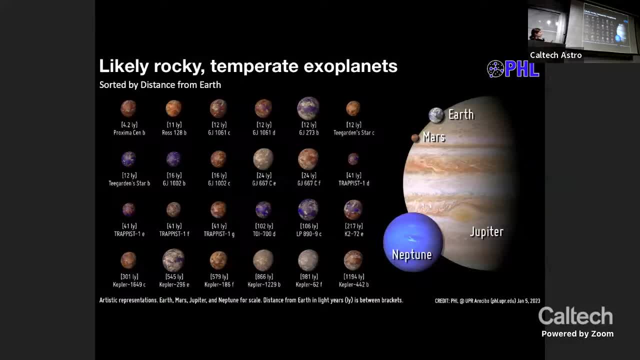 that you might be most interested in. Now. these are not real images, and I'll explain why in a little bit, But there are around 20 or so planets that are just about the right size to be rocky and they're just about the right distance between them and their host stars. 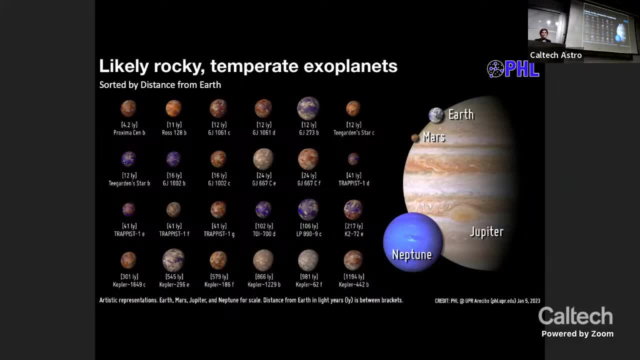 But if these planets do have atmospheres, maybe there might be liquid water on the surface of these planets, so maybe there might be life there. So the exact number of these so-called habitable planets varies depending on who you ask, But importantly, you can see the role of these planets. 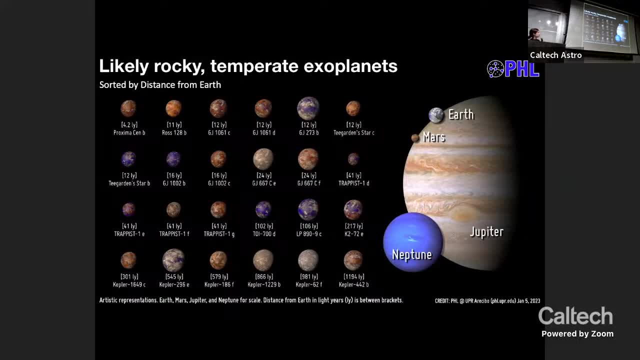 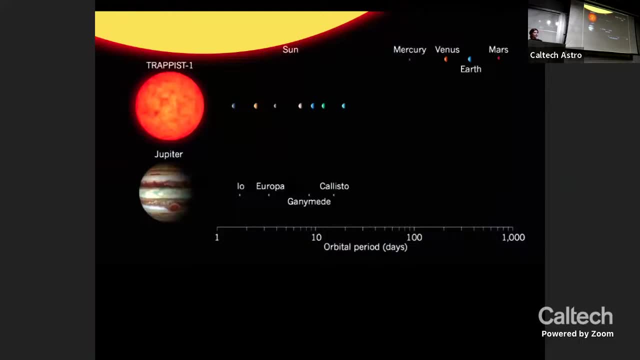 and they're all about the same size of Earth, so that's much smaller than the planets Jupiter and Neptune. However, every single one of those planets orbits a star unlike our own. They all orbit small, cool red stars. We call them M dwarfs. 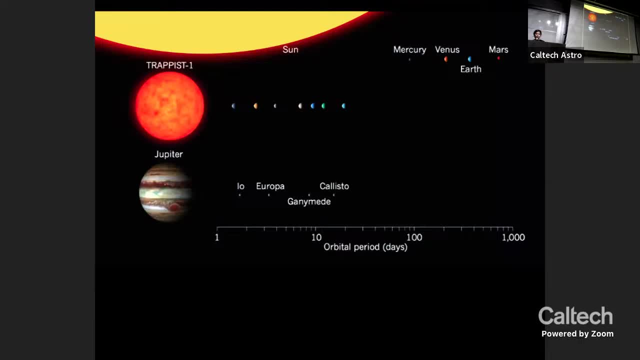 So they are much smaller, much cooler, much more red than our yellow sun. The famous TRAPPIST system, which is shown here, hosts seven Earth-sized planets, four of which are in that gallery I just showed because they might be about the right temperature. 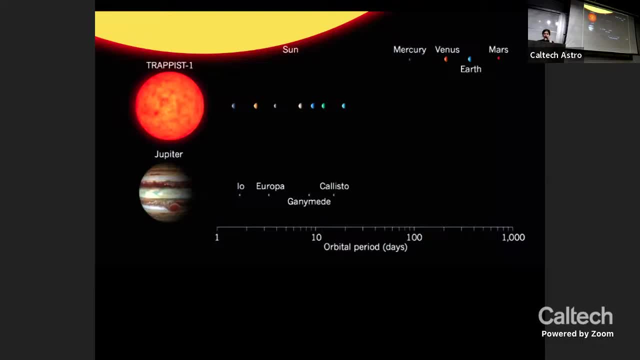 for liquid water to exist on their surface if they have atmospheres. Now, the star in this system is way smaller than the sun. You can see the size comparison here. It's actually not that much bigger than our planet Jupiter. So as yet we've never found an Earth-sized planet. 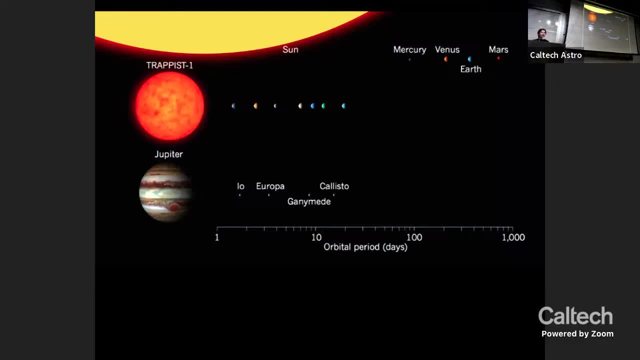 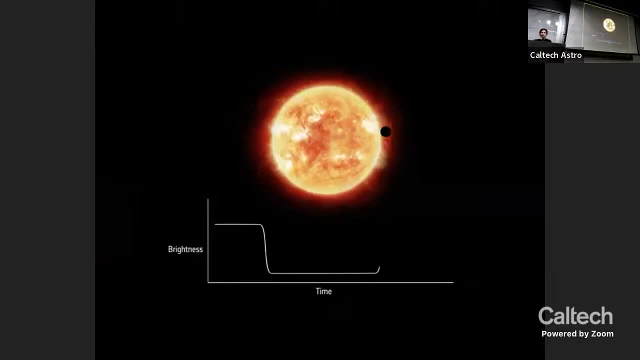 that orbits in a period of about one year around a sun-like star. and that's because this is really hard to do And that's because of our detection methods. So taking a direct image of an exoplanet is like trying to take a picture of a pea. 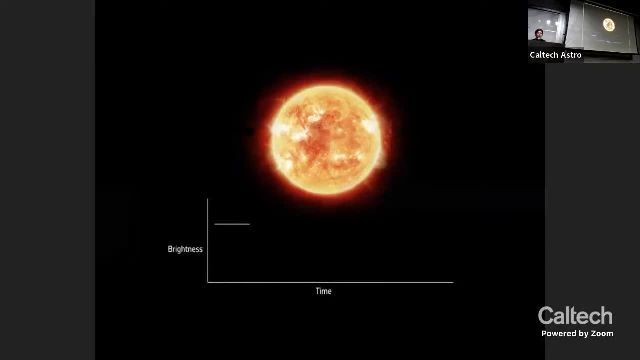 held right next to a flashlight from a mile away. So right now we mostly use indirect methods, like the transit method. So this works by if the orbit of the planet is aligned just right, such that the planet passes in front of its star once she orbits. 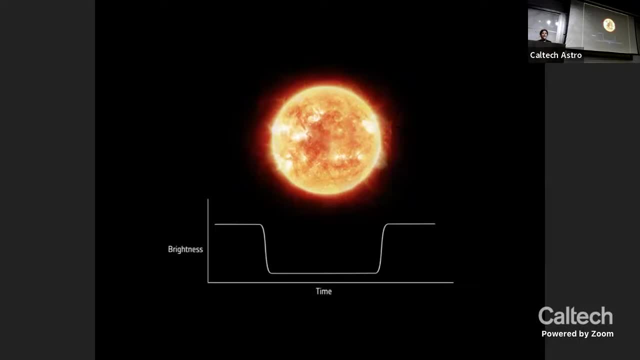 we can use our telescopes to measure that dip in the brightness. Now, when we measure the brightness over time, we call that a light curve. So these dips in that light curve here, if they appear very regularly, can indicate the presence of a planet. 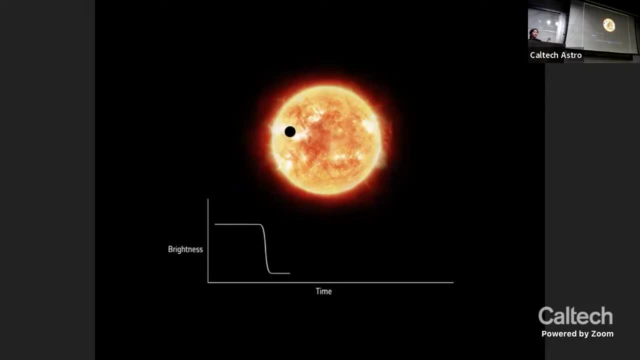 And the size of that dip is proportional to the relative size of the planet and the star. So you can imagine that if you have the same size planet but a much smaller star, that transit depth actually gets a lot bigger and it's much easier to detect. 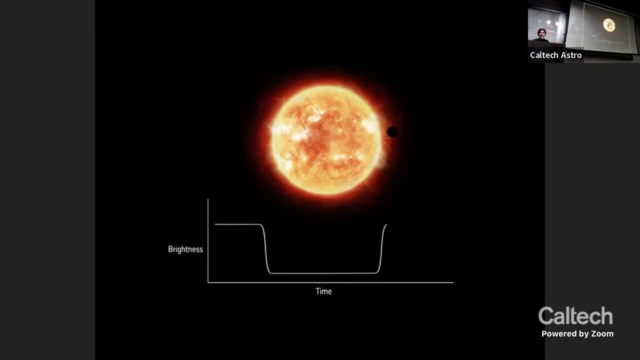 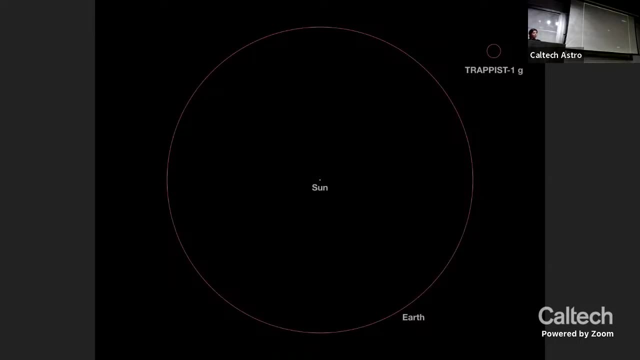 So that's why- part of the reason why we've been able to find small planets and small stars, And that's not the only reason For a smaller, cooler star. if you want to be in the habitable zone, you need to get much closer. 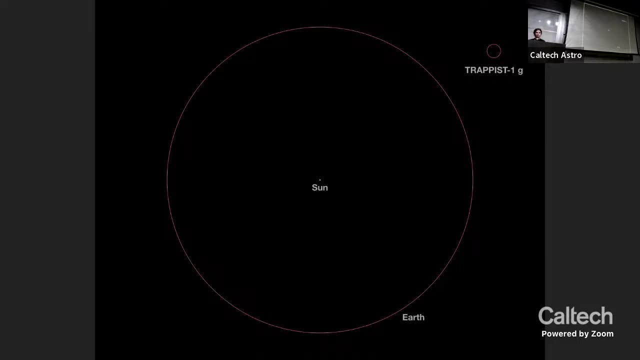 So here's the orbit in the upper right of this slide here And that shows the distance of the outer Trappist planet, Trappist-1 g h. So this is right outside the habitable zone of Trappist-1.. 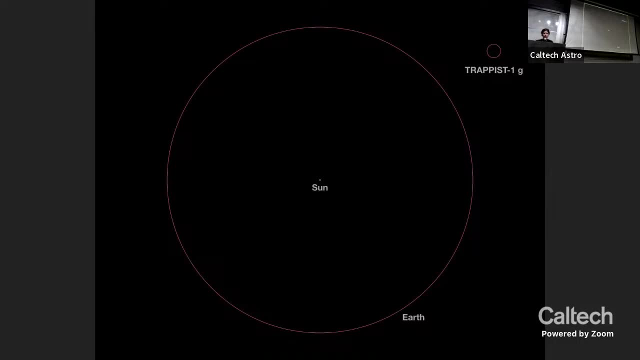 And you compare that to the size of the orbit of the Earth, It's much smaller. So for the transit technique the orbit needs to be aligned just right that you pass in front of the star Now it's way more likely that you're going to be aligned just right. 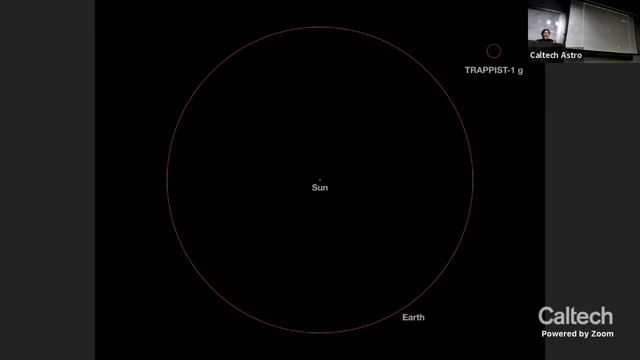 to do that if your orbit is much smaller. Also, these orbits take like a few days to complete, which is much shorter than the 365 days that you would need to stare at a Sun-like star to observe a truly Earth-like planet. And not only that, but M-dwarfs. 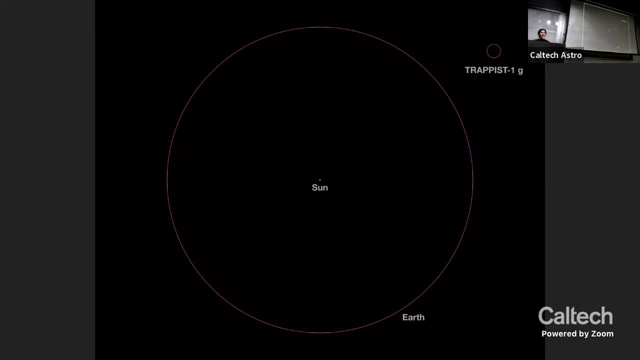 these tiny small stars. they are way more common in the galaxy than Sun-like stars. About 70% of the stars in the galaxy are these small red, M-dwarf stars. So this is why it is way easier to find warm, rocky planets around those small stars. 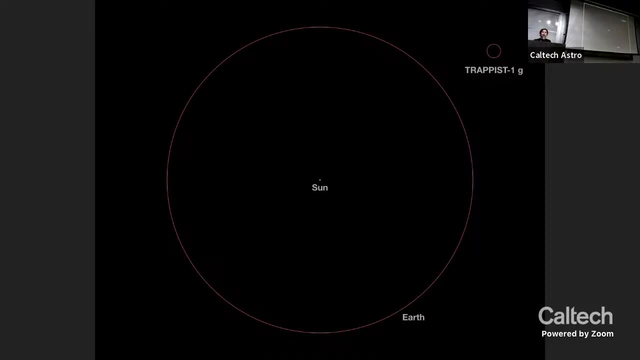 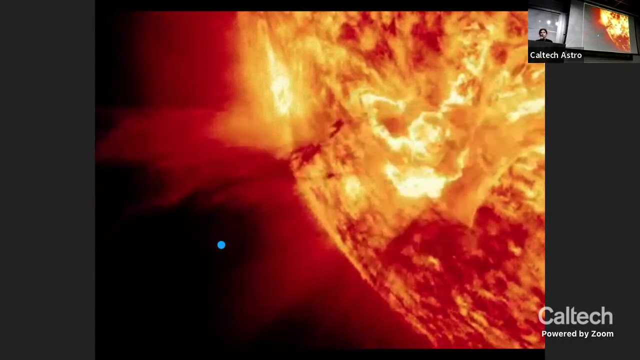 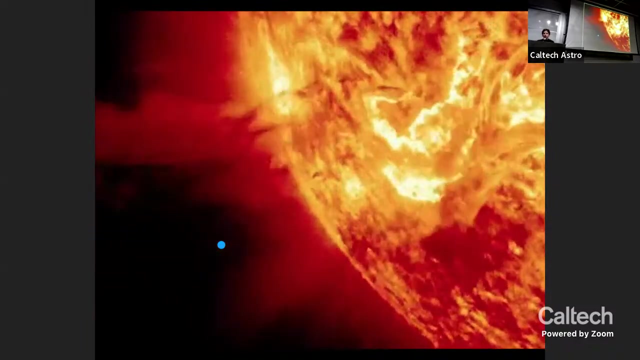 So the question is: is this the best place to look for life in the universe? if they are so easy to find and if they're so common, It might not be. This massive explosion that you see on the surface of the Sun is a coronal mass ejection. 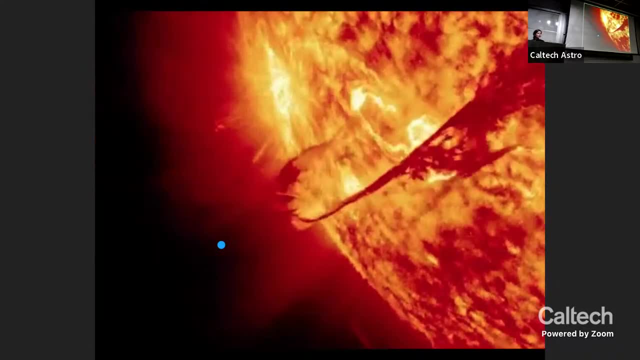 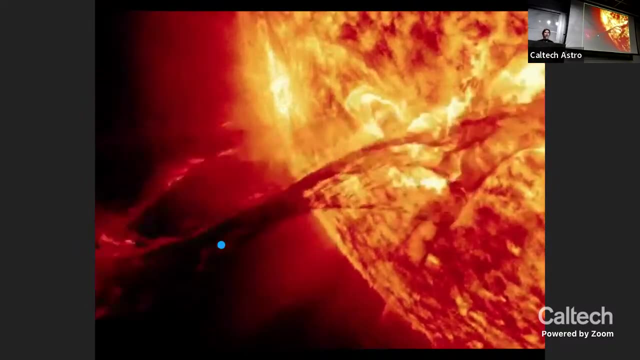 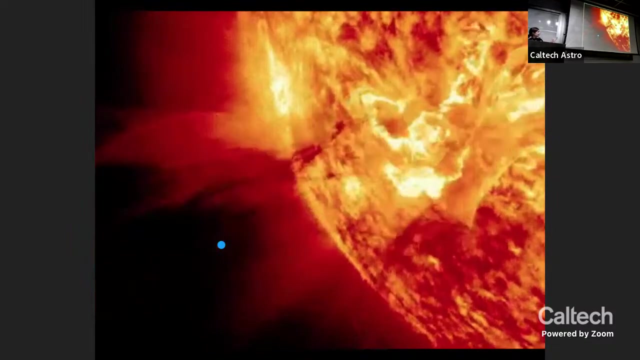 It's a huge explosion of matter and is often associated with giant flares, massive increases in the brightness of the star and lots of high-energy radiation comes streaming off the star. You can see I've put the Earth perspective in this plot here. 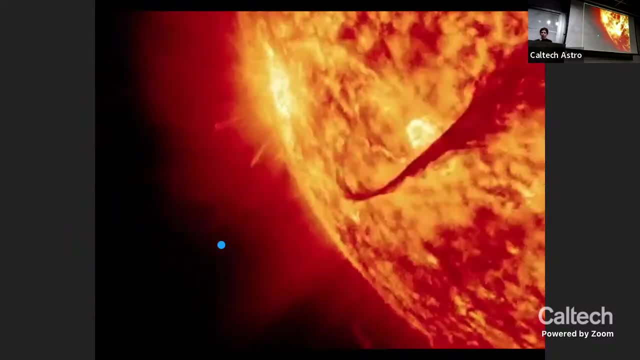 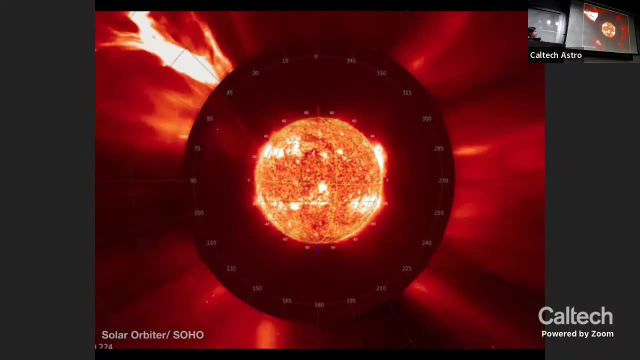 It's a tiny blue dot, way smaller than this huge explosion, And if we zoom out a bit, we can also see other dangers too. So around the edge of this video, here is a giant halo of material that you can see, and this is called the solar wind. 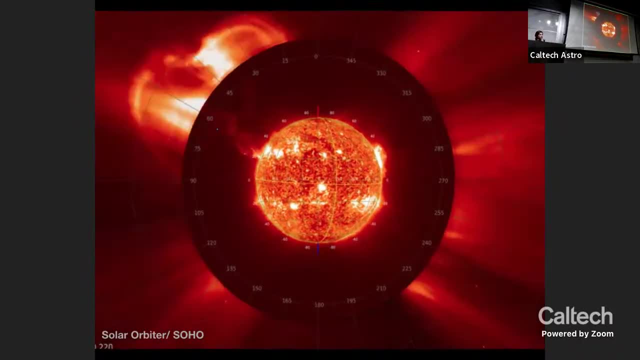 And it's basically very high-energy particles streaming out of the Sun. Now our Earth's atmosphere is protected by a magnetic field from this solar wind, But if this wind was a bit stronger, or maybe the Earth was a bit closer to the Sun, 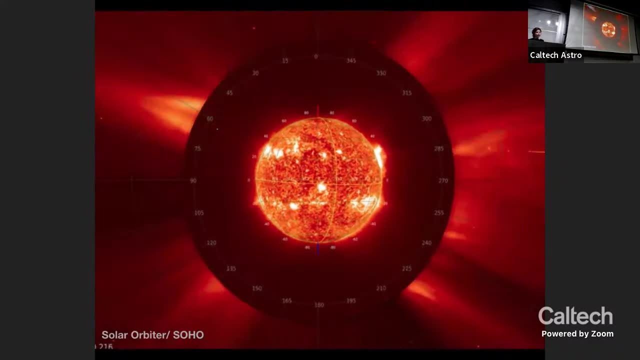 that magnetic field might not be enough. If you're in the habitable zone of an M dwarf, you are much closer to the star, much closer to this stellar wind. Now we have measured a few, but it's really difficult to measure the stellar winds. 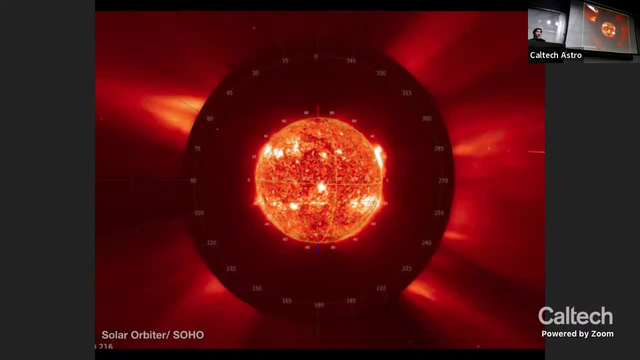 of any other stars other than the Sun. We have some measurements, but basically we're not sure how strong the stellar winds of M dwarf stars are compared to our Sun. Now these massive explosions which are often associated with big flares, they're a little bit easier to study. 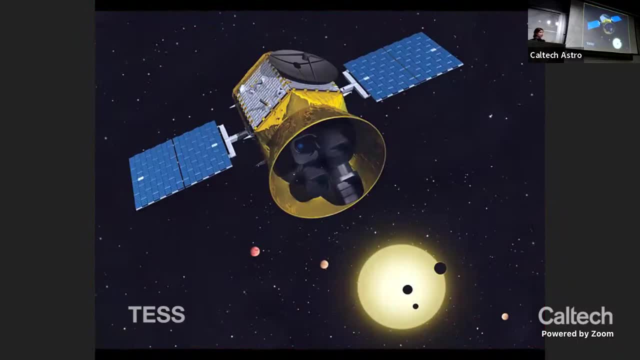 We have been able to do that for M dwarfs. There's a recent really cool space mission that we've been using to do that, called TESS. It's the Transiting Exoplanet Survey Satellite, And this was launched in 2018,. 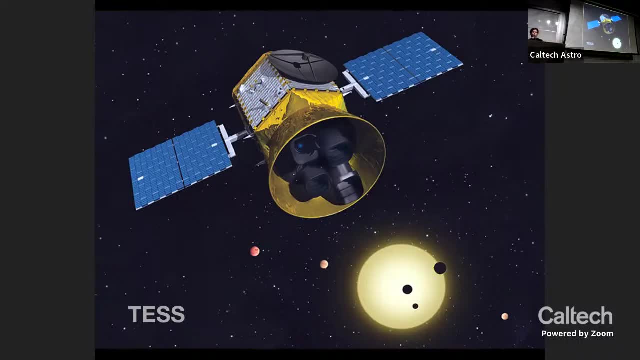 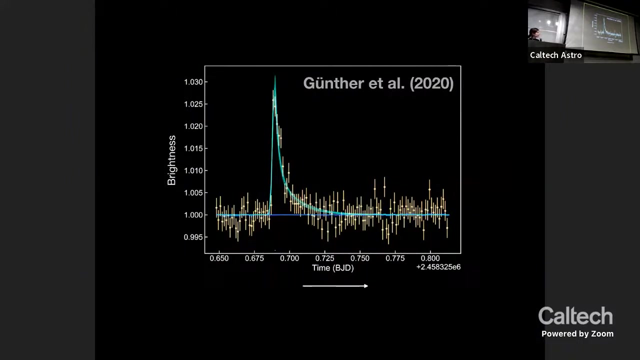 and it measures the light curves, those brightness-over-time plots of hundreds of thousands of stars, And they are searching for those tiny dips in those light curves that indicate the presence of planets. We can also use this to study the stars themselves And we can detect those massive flare events. 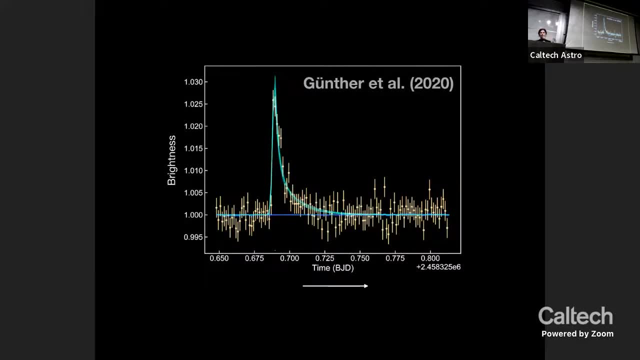 And they look like this in those light curves. So these are sudden increases in brightness in the light curve of the star. Time is going to the right And these signals indicate the release of a massive amount of high-energy radiation which may strip away a planet's atmosphere. 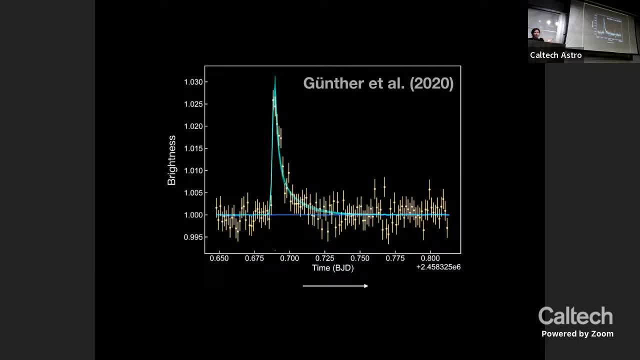 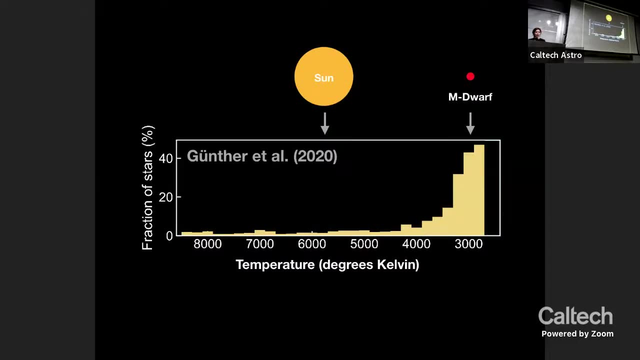 And this is from a neat study led by Max Gunther, where they searched the light curves of thousands of stars for different kinds of sizes and temperatures. So they counted the fraction of stars which showed detectable flares in two months of observations. 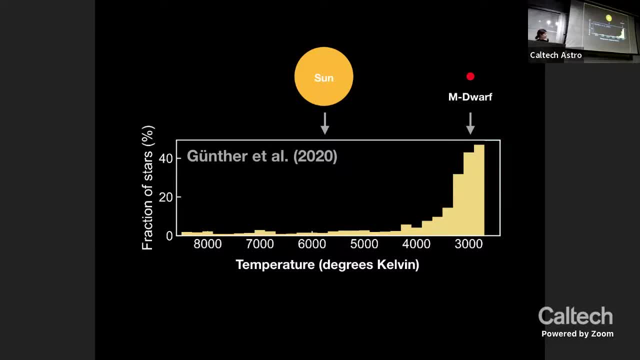 And so you can see the temperature of the star going along to the right. Cooler stars are to the right, And then this just shows you how many of those stars showed those observable giant flares in that time. And you can see the Sun is about 5,800 Kelvin. 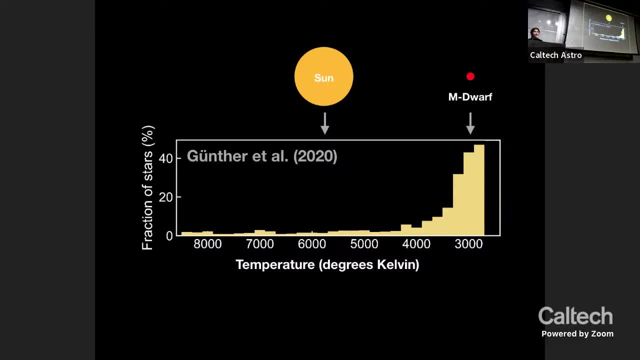 And those M dwarfs are much cooler- about 3,000 Kelvin, And the fraction of those stars which showed detectable flares shoots up when you go to these smaller stars. Not only are you closer to these flares when you're in a habitable zone around an M dwarf, 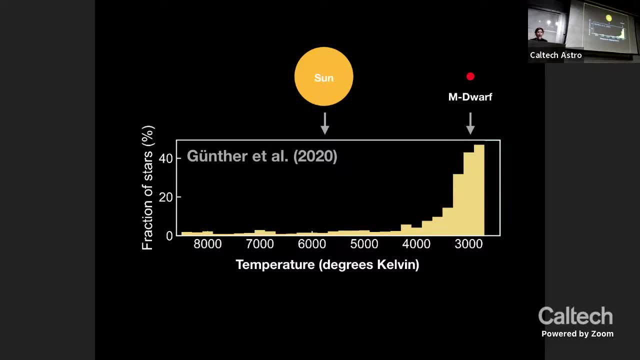 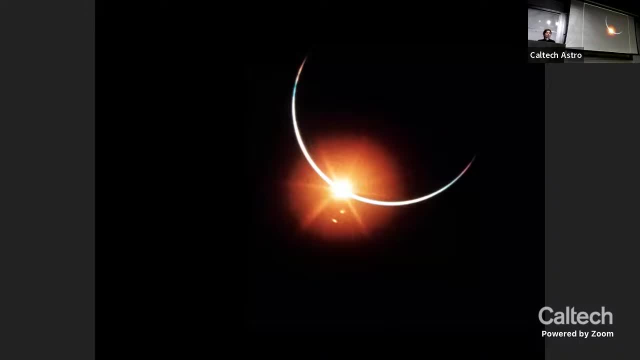 but these flares also happen way more often and they are also much more energetic. So what does that mean for our precious thin atmosphere around these rocky M dwarf planets? The honest answer is: we don't actually know yet, And that's because we've never been able to detect. 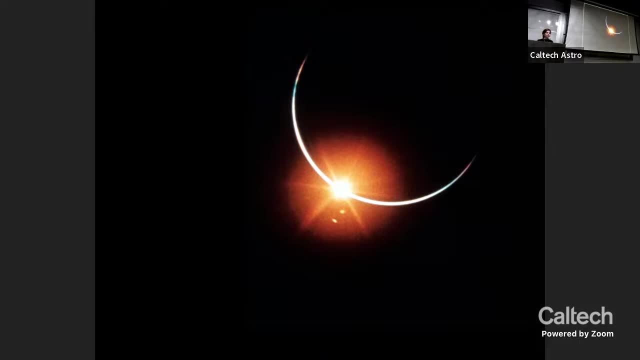 an atmosphere around a rocky planet, around another star. And this we don't know. if this is because that these planets, these atmospheres are so thin that we don't have the technology to observe them yet, or if it's because those flares 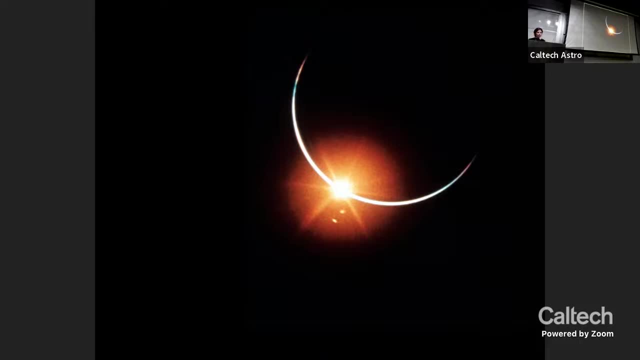 have stripped them all away, And so the way we study these planets is kind of shown in this picture here, And in it you can see just how thin the Earth's atmosphere is when it's backlit by the Sun, So the light doesn't pass through. 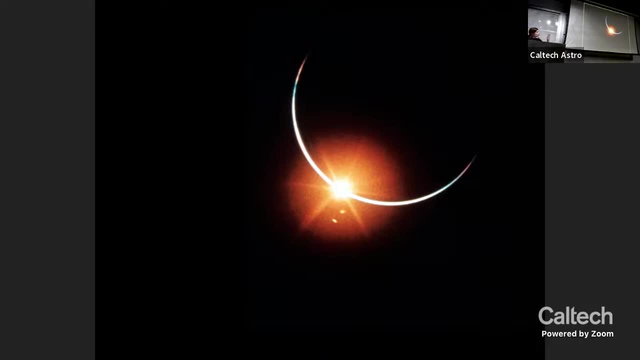 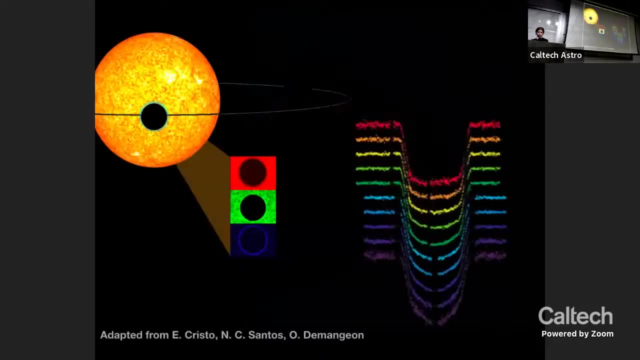 the main disk of the Earth, but a tiny amount of it streams through the slightly opaque atmosphere that we see, And this is how we study the atmospheres of planets around other stars. It's basically an extension of the transit technique, except this time. 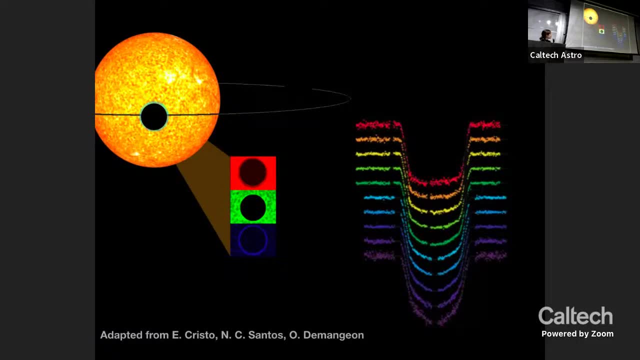 when we measure the light curves, we split up those light curves into different colours and we can look at those transit depths and they will change depending on the colour that we're using, And the reason is because there are specific gases in the planet's atmosphere. 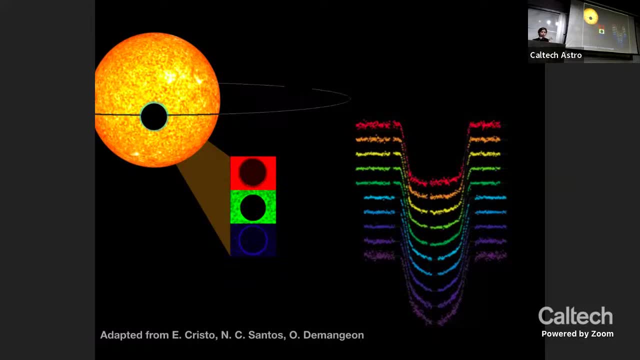 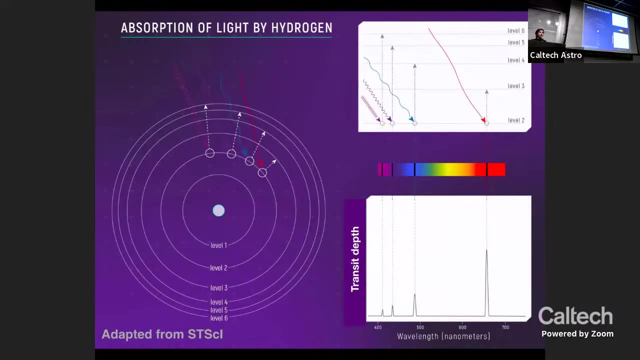 that will absorb very specific colours of light And they will make the transit depth look deeper, And that's because of the basic structure of atoms. So this is the only slide I have in here that includes atomic physics, Don't worry. So on the left side, 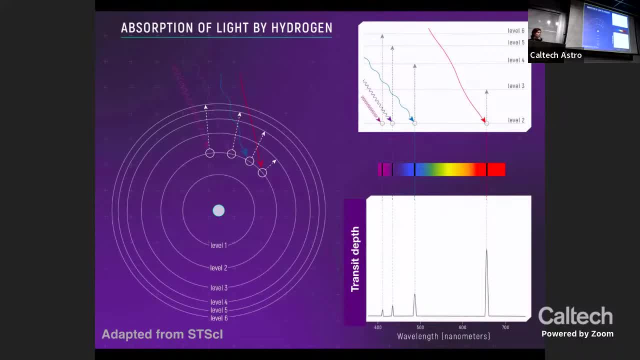 we have a cartoon of a hydrogen atom. So in the middle we have a nucleus And surrounding the nucleus are these shells of electrons. These are tiny, tiny particles buzzing around the middle of an atom. All of the hydrogen atoms look exactly the same. 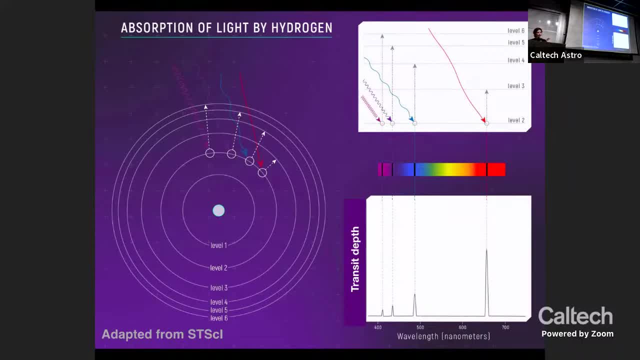 So these tiny electrons can sit in these exact shells, but nowhere else. They can't be anywhere in between them, But they can jump from shell to shell And they can do this by absorbing a very specific energy of light. And when you look at a rocket, 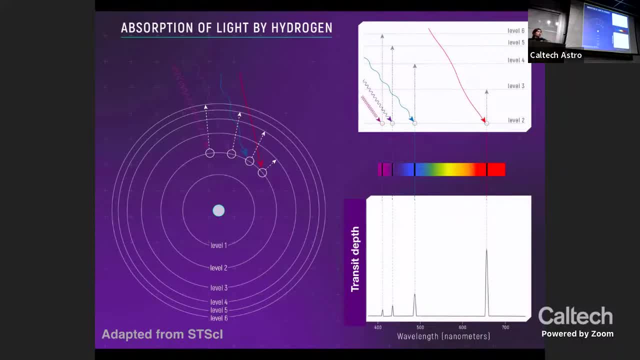 and when you look at a rainbow in the sky, that's light being sorted out into its different energies: Purple light to the left of this rainbow, you see here, that's higher energy light And as you decrease in energy, you move through the rainbow. 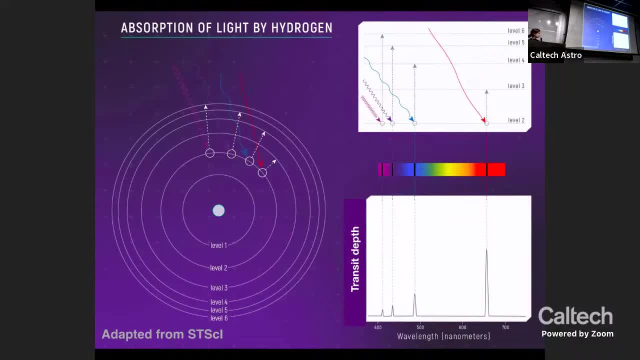 And that red on the right side. that's lower energy light And you can see there are several strong absorption lines of atomic hydrogen that correspond to these specific jumps that come out as these specific colours, And there are also different energies that we can't see with our eyes. 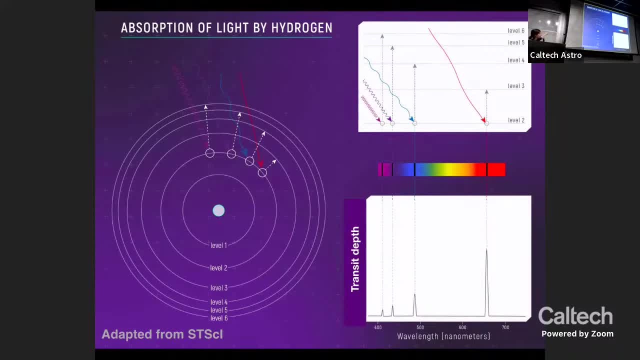 So if you would move further to the left of this rainbow, past the purple, you'd move into the ultraviolet light That's higher and higher energy, And if you move further into the red, you go into infrared. We can't see either of those with our eyes. 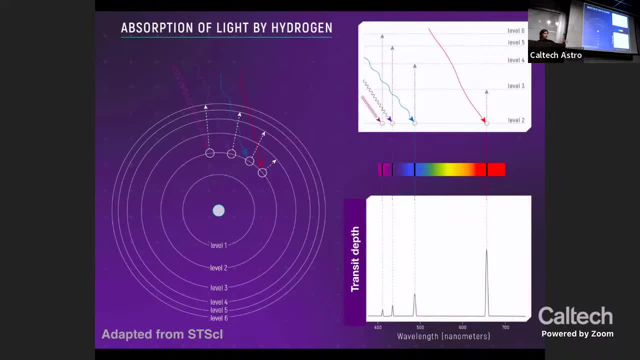 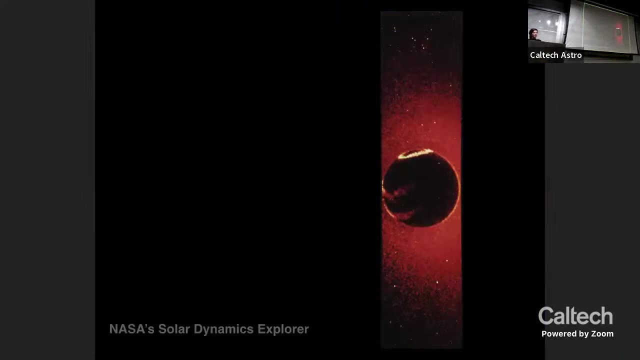 but we can see these visible lights of hydrogen, And so if you looked at the transit depth of a planet with a bunch of atomic hydrogen in its atmosphere, that planet would look way bigger. So we can look at these four specific lines. So let's take a look at the Earth. 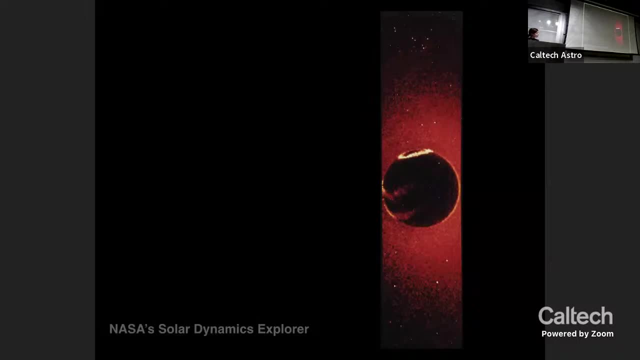 in ultraviolet light actually so not visible. We can't usually see this with our eyes, But in this new way of looking at the Earth, you can see that there is actually a massive cloud of hydrogen surrounding the Earth, And it extends up to 7,000 kilometres. 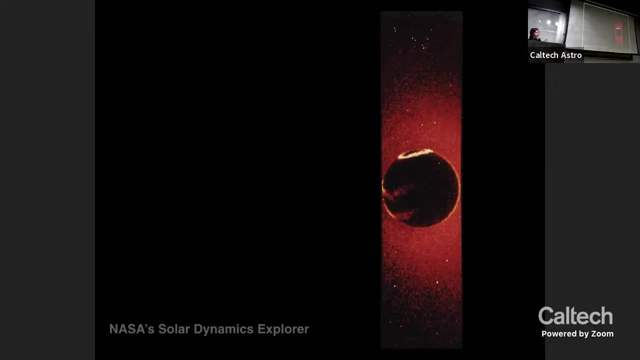 above the Earth's surface. So there's a very strong absorption line of hydrogen in the ultraviolet. It corresponds to that very lowest level. the jump from that very lowest level to the next level up, So this hydrogen which isn't really present, 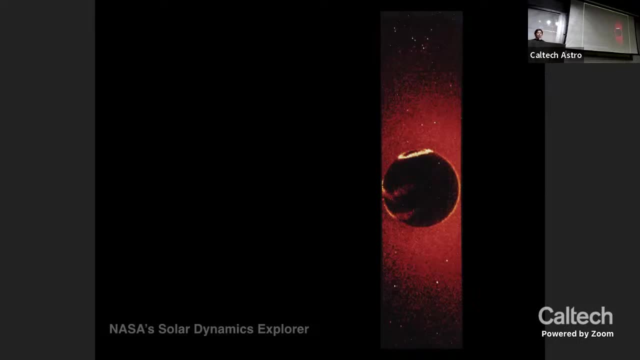 in the lower atmosphere of the Earth. it's too light, It kind of drifts all the way up. So this is trickling off at a rate of about 90 tonnes per day. So Earth is actually losing some of its atmosphere, but very slowly. 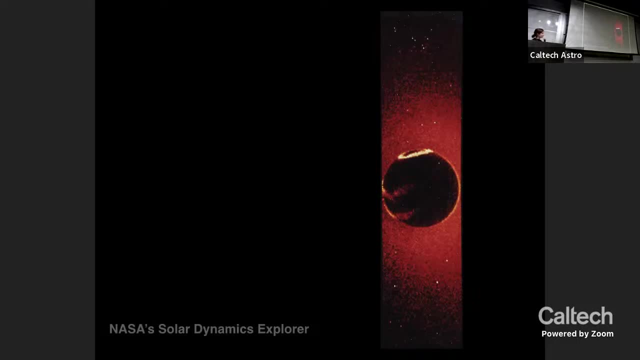 because there are five quadrillion tonnes of the Earth's atmosphere still left, so we shouldn't worry too much about it. So this is a region of a planet's atmosphere that I'm most interested in, because it's where we can see the escape actually happening. 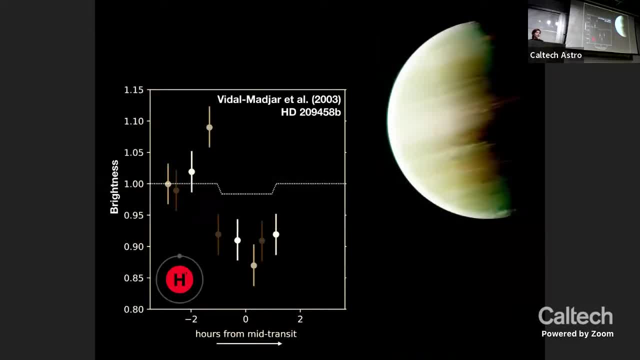 So the first planet with its escaping atmosphere to be detected was found using that line of hydrogen in the ultraviolet, And it was around this massive giant planet. It's a Jupiter-sized planet that orbits its host star. Its host star is like the sun. 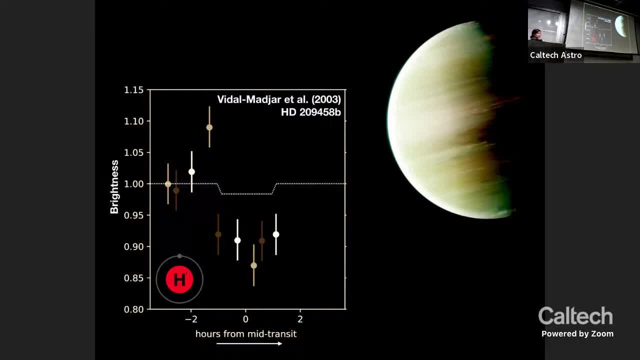 It's very hot And it orbits that once every few days. So it's a super hot planet about the size of Jupiter. So we call these hot Jupiters. So in the visible light you would expect this planet to be relatively small. 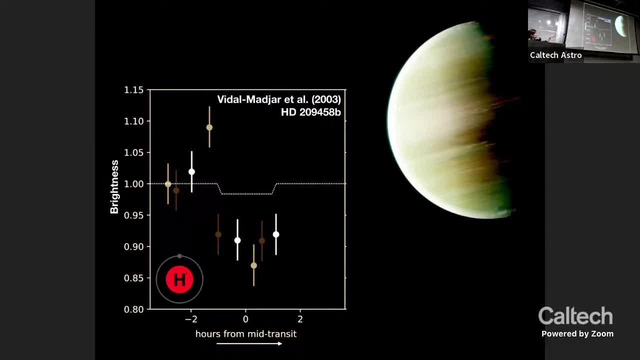 You can see the light curve of that by the white dotted line. We expect it to have a transit depth of about 2%. When you look in this very strong line of hydrogen in the UV, we see that actually the planet blocks out about 10% of the starlight. 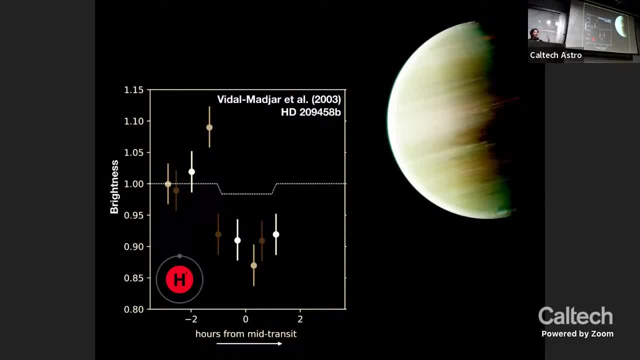 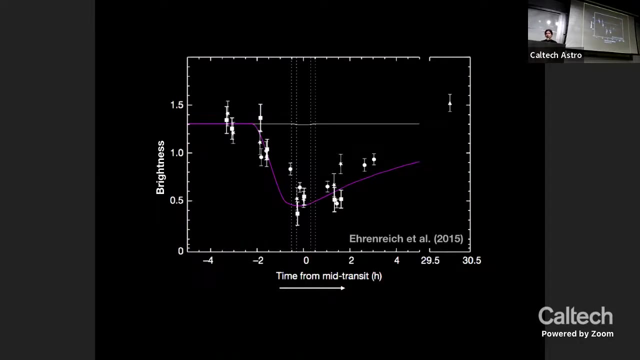 And so this means that this planet is surrounded by a massive shroud of hydrogen that is streaming off into space because it's being heated up and expanded by a lot of stellar radiation. And here's another transit light curve of another planet in that very same hydrogen line. 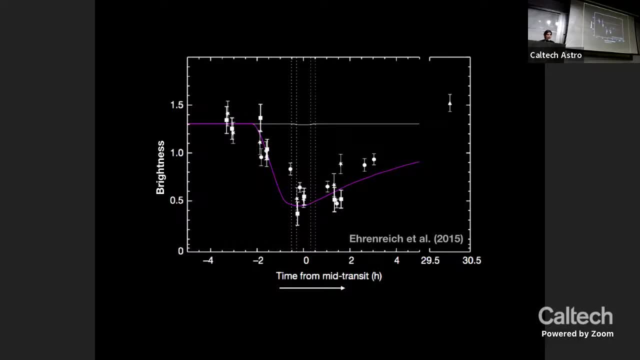 So the vertical dotted lines here tell you exactly when we expect the planet to start passing in front of the star and to finish passing in front of the star. But you can see that these white data points are what we actually measure And you can see that they start dipping. 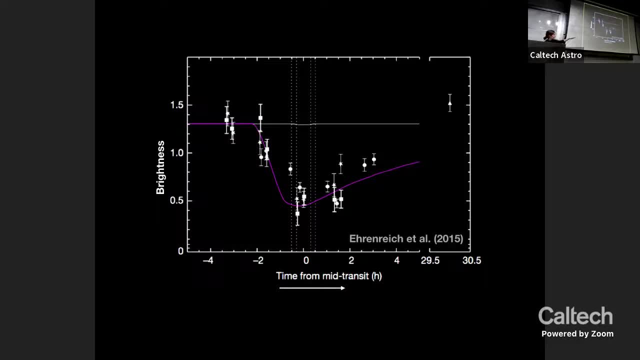 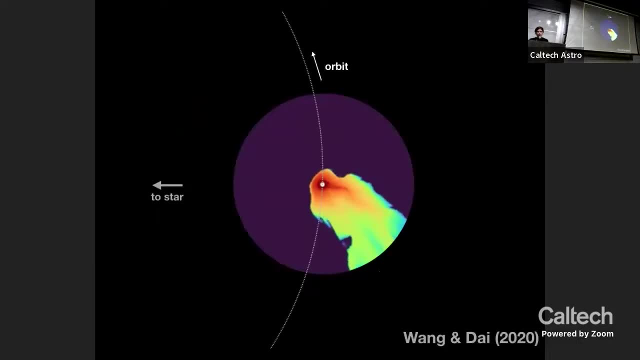 way before that line starts And they also carry on. They stay low way after. They don't go back up to that straight line, like we should expect, And what that means is that this planet is surrounded by a massive cometary-like tail of material. 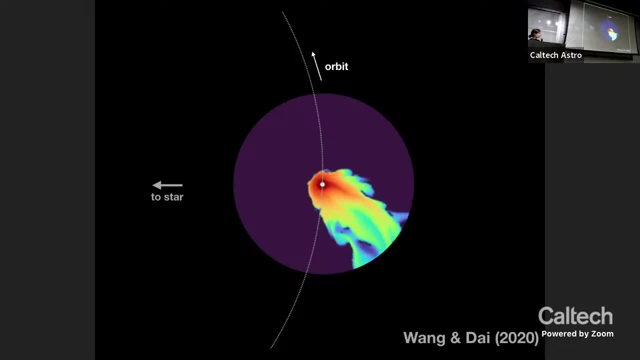 that is streaming away from the planet. So this is a top-down view of the system, And so the planet is orbiting around the star on that white dotted line, And the star is like over here off the left of the screen, And there is this really beautiful stream. 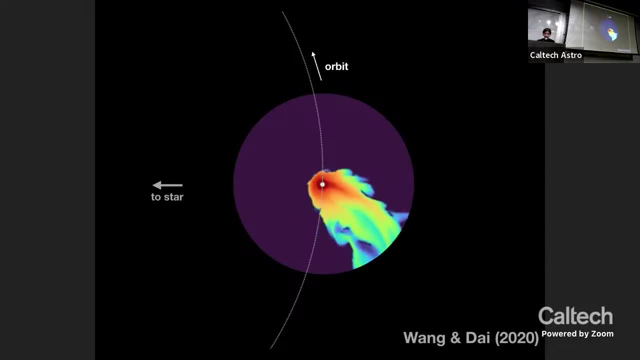 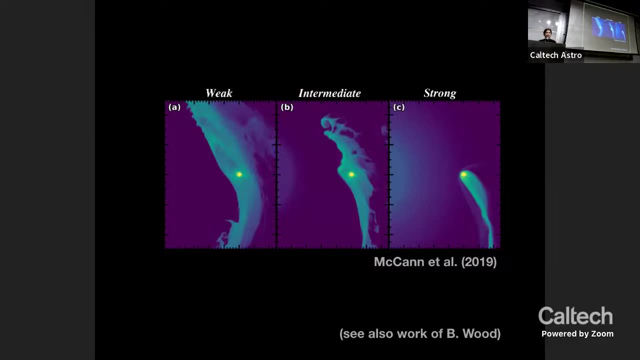 of material that's escaping off of the planet, And one reason I'm like really interested about studying these wispy tails trailing behind the planet is because of this really nice work led by John McCann a few years ago. So they show that when you increase. 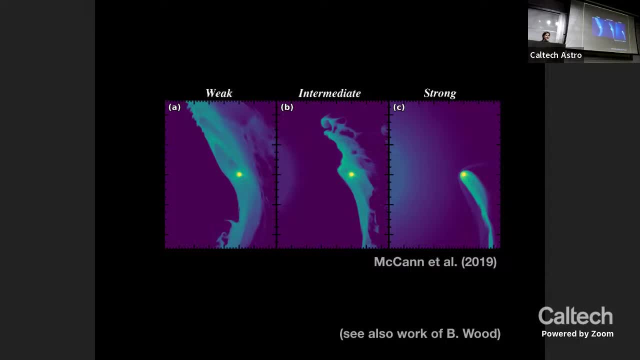 the strength of that stellar wind. that's that giant red halo surrounding the sun that we saw earlier. When you pump that up, you can carve out the material that's escaping from the planet into these tails, these very fast tails streaming behind the planet. 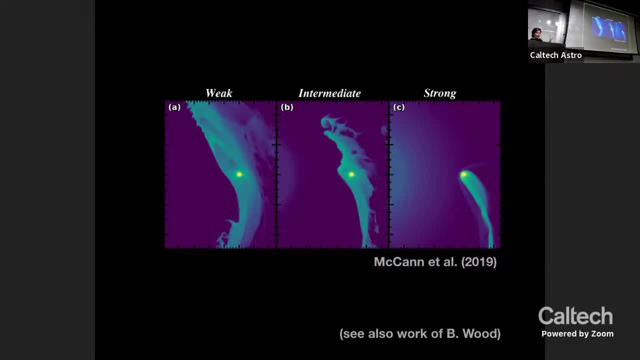 When you don't have much stellar wind there, like the very left side of the planet, the left side of the figure, here the material just sort of wisps around and forms this ring around the star. But when you increase and increase the strength of that strong stellar wind, 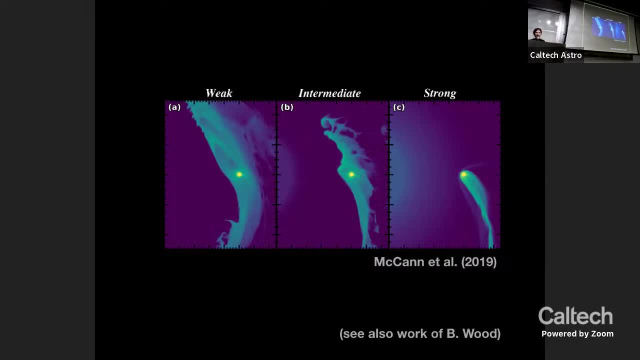 you can sculpt the material and it streams behind like on the right side. So we can actually use observations of this escaping material to measure those stellar wind strengths which have been pretty difficult to detect so far. And this is kind of the cutting edge. 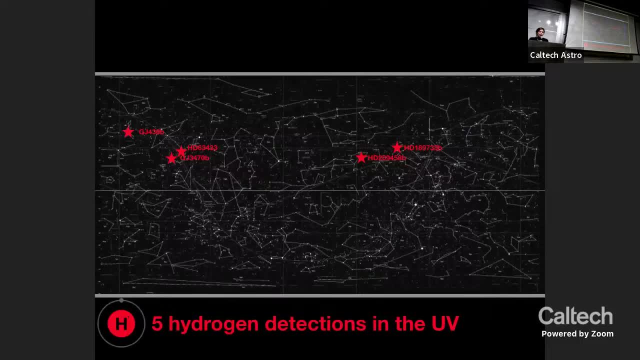 of what we're able to do today. However, since that first detection of hydrogen in an exoplanet atmosphere 20 years ago, there have only been five detections using that same hydrogen line of escaping exoplanet atmospheres, So this means it's very difficult. 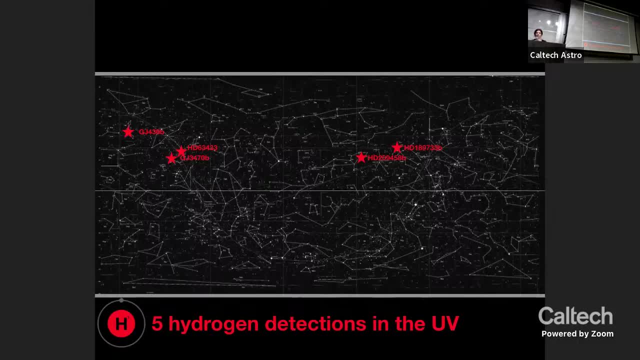 because we want to do a big survey of all the different kinds of planets and all the different kinds of stars, to understand which stars have strong stellar winds, which kinds of planets are able to hold onto their atmospheres. But we've only been able to do this. 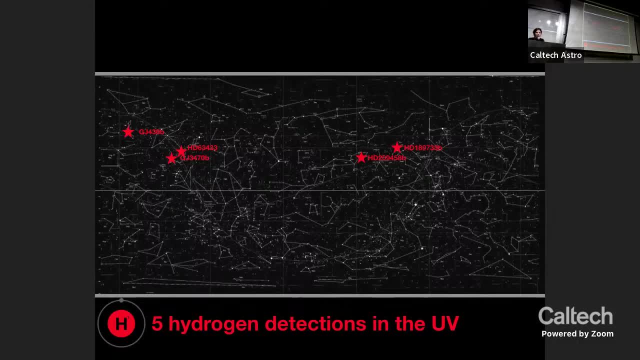 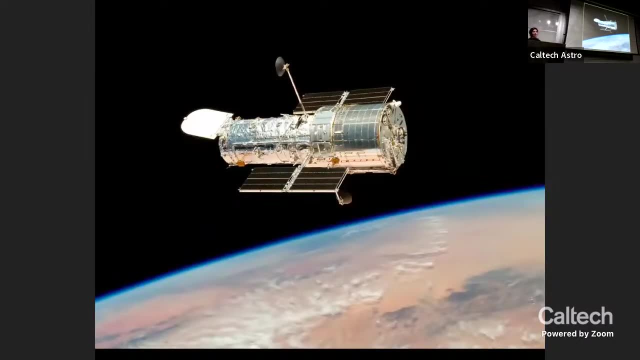 for five very big planets, And this is kind of a problem. Part of the reason it's so difficult is that you can only do that kind of work with the Hubble Space Telescope. It's the only one that can observe in the ultraviolet right now. 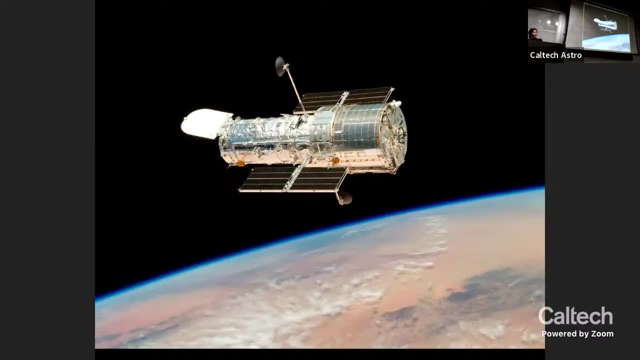 It's the only one that can see that hydrogen. When I was a PhD student, I used this telescope to look at a different planet, And this time I wasn't looking in the ultraviolet, I was looking in the infrared, so at lower energies. 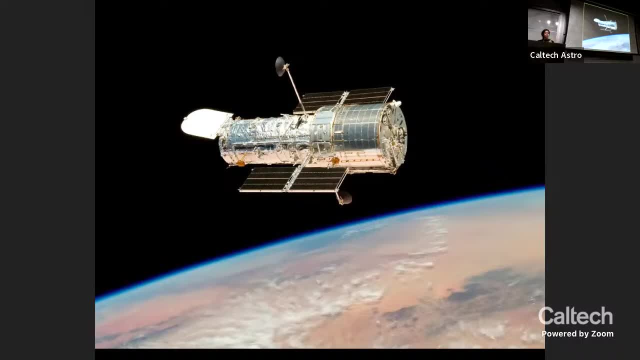 And we were looking at this planet and it's not as hot as that one I showed you before. It's slightly cooler, but still a gas giant. And we were looking for methane in its atmosphere with Hubble, So methane is like in cow farts. 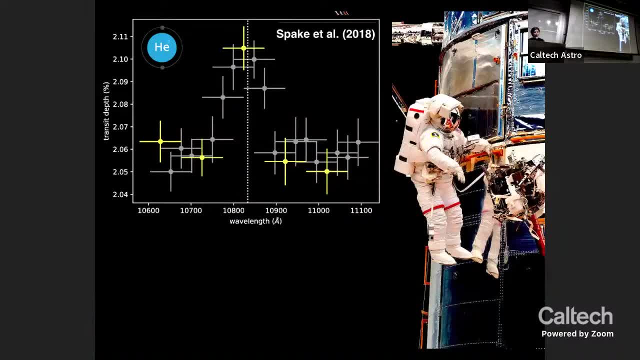 We didn't actually detect methane, however, And here is a little picture of astronaut John Grunsfield. He's installing the instrument that we used to make this observation, And what I'm showing you here is a transmission spectrum. So what this is. 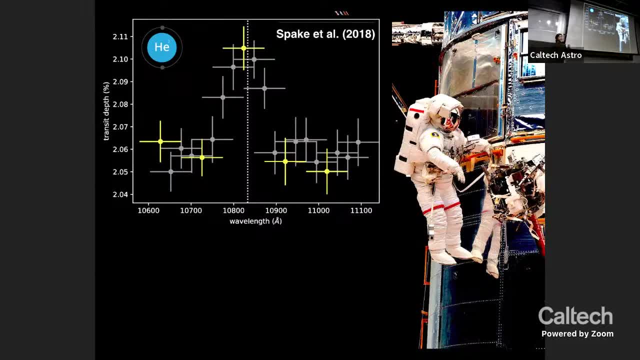 is, we have wavelength along the bottom here, So this is basically the color of the light or the energy of the light. And on the y-axis, here we have the transit depth, So that's how much light the planet is blocking out. And so when you see a peak, 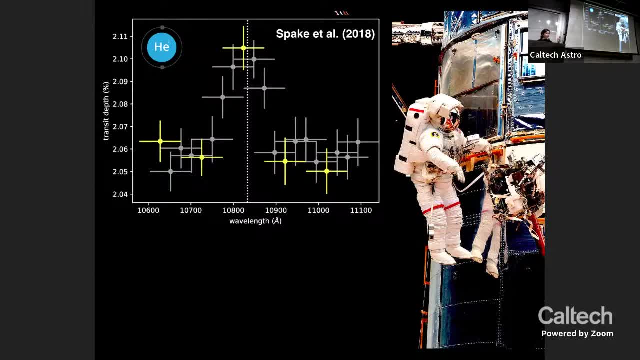 in this transmission spectrum a very specific wavelength that corresponds to one of those strong absorption lines of an atom. that tells you that there's a lot of that stuff In this planet atmosphere, And so what? this is this peak here that we saw. 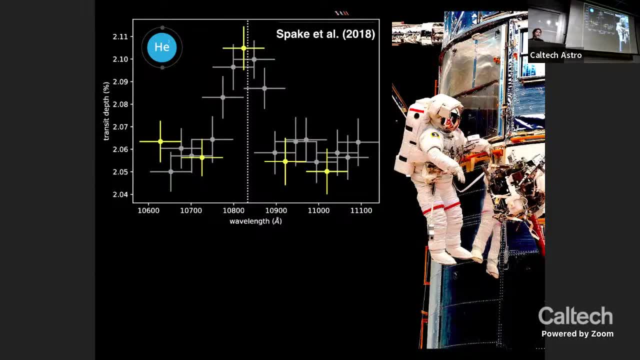 is a very strong line of helium. Now, helium is the second most common element in the universe after hydrogen, And for these planets that have a lot of hydrogen and helium in their atmospheres, it's a pretty important element to find. People have been looking for this. 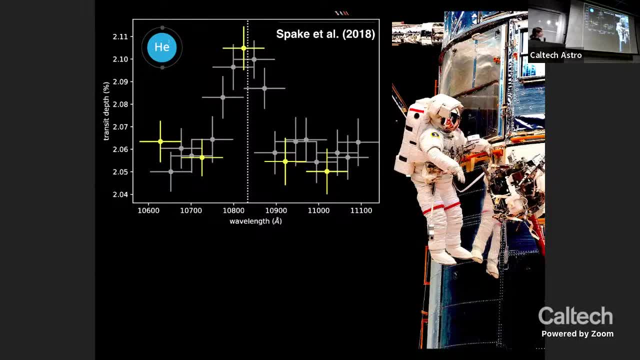 Well, they started looking in the early 2000s, but it was pretty tough, so they kind of gave up. We discovered this totally by accident, And with this helium we can also see those massive streams of material escaping from the exoplanet. 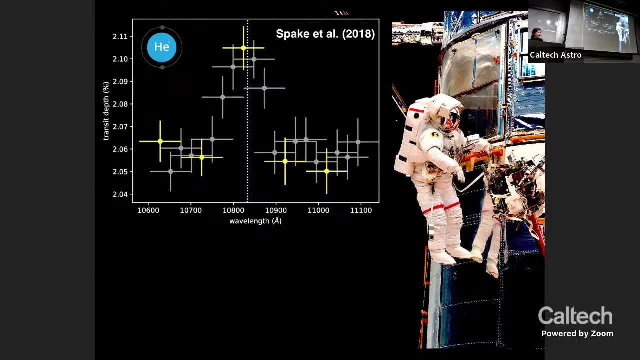 I was pretty excited when we found this. I was just a PhD student, I wasn't expecting to see something cool like that And we were like writing up the results and the paper hadn't come out yet. But I was visiting Harvard University. 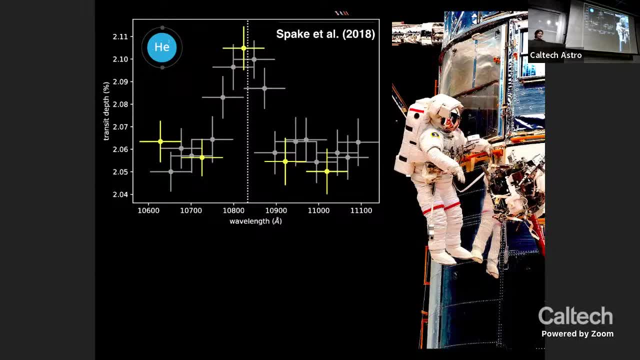 I felt very impressed to be there. I was quite nervous And I went down to coffee and I was like trying to make small talk with some people there And I started talking to this woman. No idea who she was. It turns out she's a very famous. 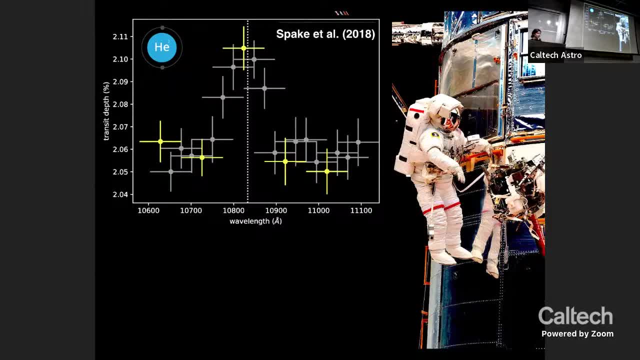 stellar astrophysicist, Andrea Dupree. She's very nice, But I was talking to her and I was like, oh, I think we might have found some helium in an exoplanet with this special line in the infrared. Do you know anything about it? 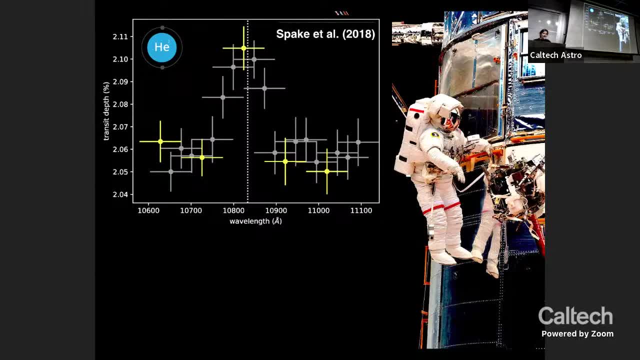 And she looked at me and she opened her mouth and she was like that is my favorite line: Come downstairs, Come downstairs. And she took me downstairs to the office of a theoretical astrophysicist, Antonia Klopcic, And Antonia was just writing. 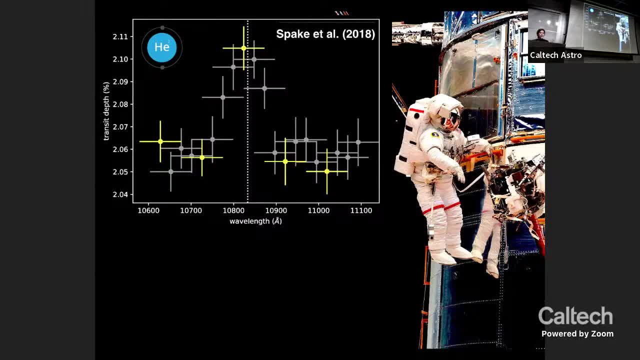 her theoretical model to explain that we should see a bunch of helium with this specific line in escaping exoplanet atmospheres. And she showed me her theory and then I showed her our detection And we were like whoa, It was like one of the best moments. 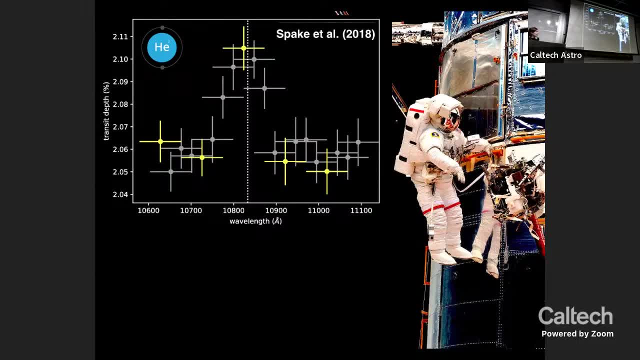 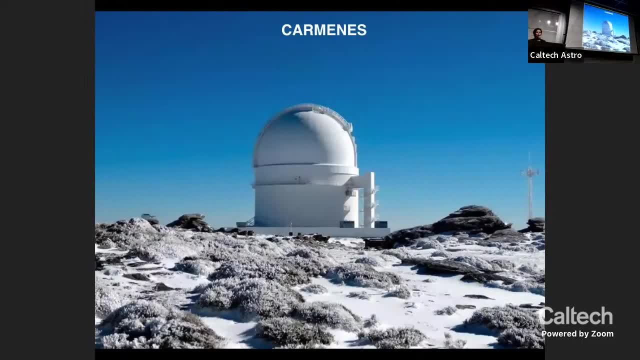 of my life. It was really fun, And now Antonia and I are very good friends and we work together. Anyway, the really cool thing about this helium line is that you can observe it with a ton of ground-based telescopes. You don't have to just use Hubble. 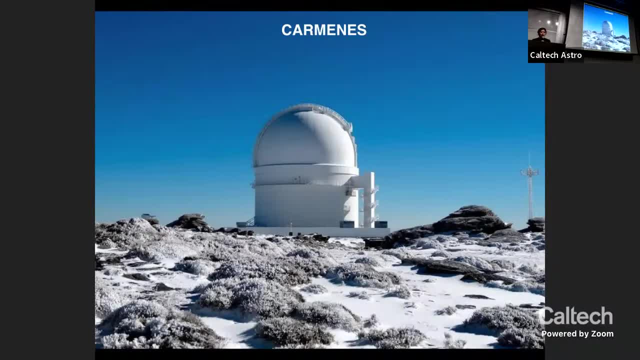 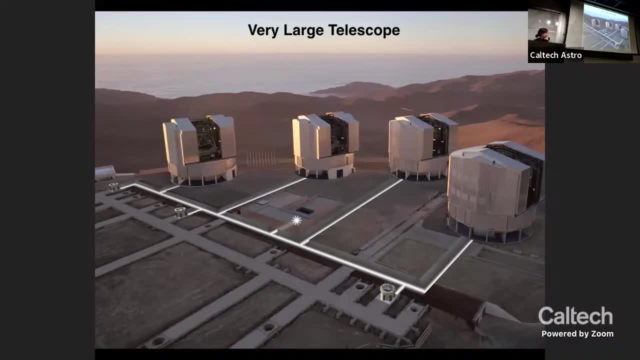 So there are loads of telescopes that can do this, including Carmenes in Spain, the very large telescope in the Atacama Desert in Chile. Yes, this is the real name of these telescopes: the very large telescopes. I really like it. 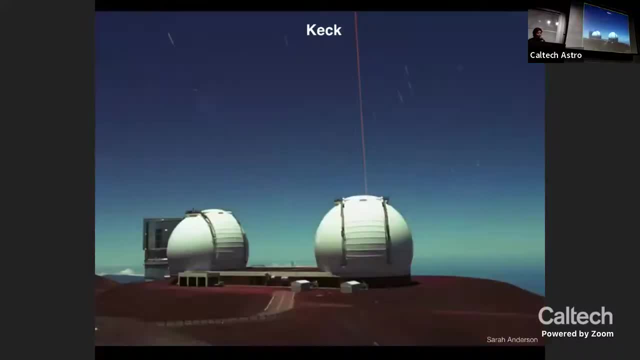 Gemini South in the Chilean Andes, and also Keck, which I use. So these telescopes stand on the summit of Mauna Kea, So this has always been a place of reverence for the indigenous Hawaiian community. So anybody like me who gets to use these telescopes- 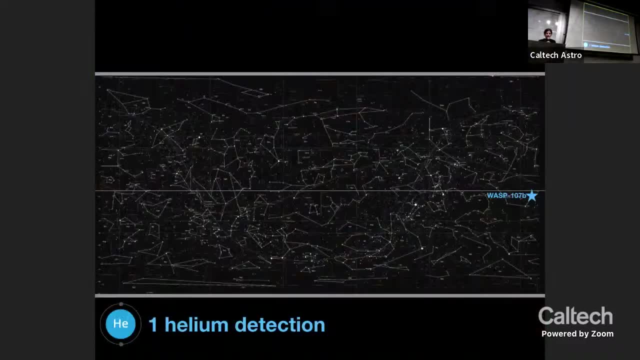 is extremely lucky and I'm very grateful. And anyway, all of those telescopes have been pointed at many planets And in the last five years we have found one, two, three, four, five, six, seven, eight, nine, ten. 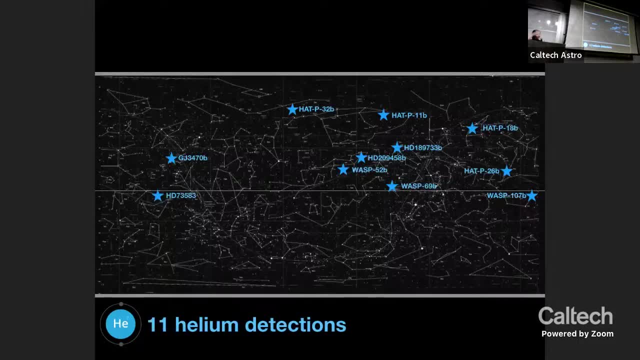 eleven planets with giant clouds of helium escaping from the atmospheres, And there's more coming this year, And this is in five years, compared to five with that hydrogen line in the last 19.. So these have been made not by me, by a huge swathe. 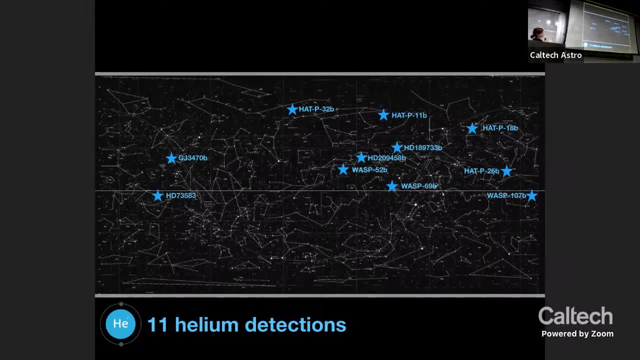 of the exoplanet community And we're kind of excited about what we can do with this. So all of these planets are all larger than Earth. We haven't been able to do this for rocky planets. We are starting to use this to understand the stars better. 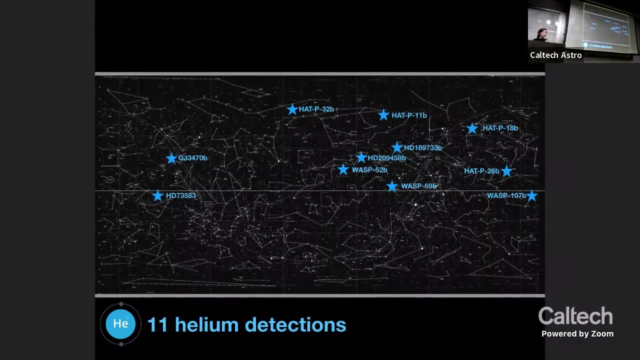 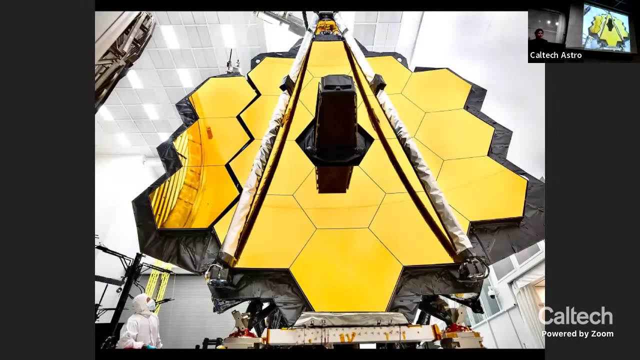 And, in general, which planets are losing their atmospheres more quickly, around which stars, at which distances. And we're pretty hopeful because we think the JWST- the largest, most expensive, most powerful telescope that we've ever launched into space- this can also see helium. 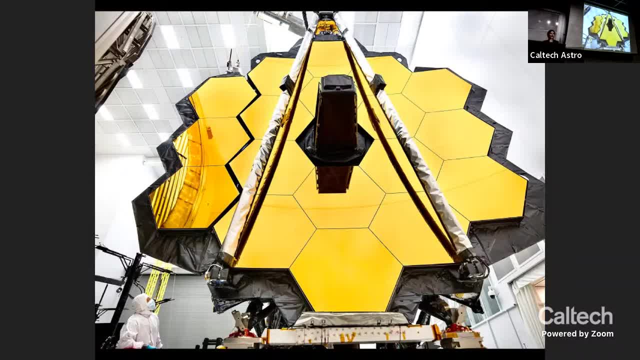 and exoplanet atmospheres and a bunch of other things, And so we're gradually getting to smaller and smaller planets. We're gradually starting to learn which ones can hold on to the atmospheres for long enough for life to evolve. We're also directly 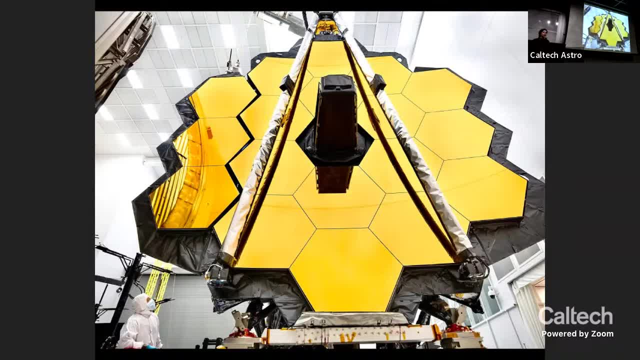 or, more directly, looking deeper into those lower atmospheres of those small rocky planets. So JWST is observing that TRAPPIST system that I mentioned earlier. We might be able to see if that system specifically has held on to its atmosphere for billions of years. 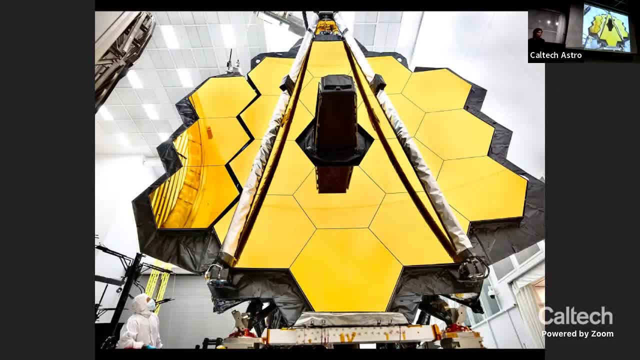 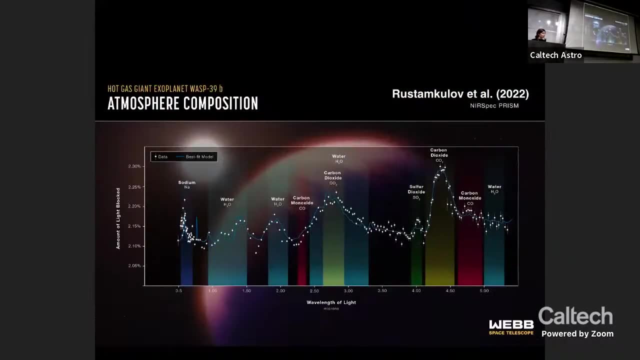 We're still not sure if that will work, But if not, we're still approaching the problem from the other direction by trying to understand the stars and these tails of wispy material. So I'm pretty hopeful And I'm especially excited to see all of the other stuff. 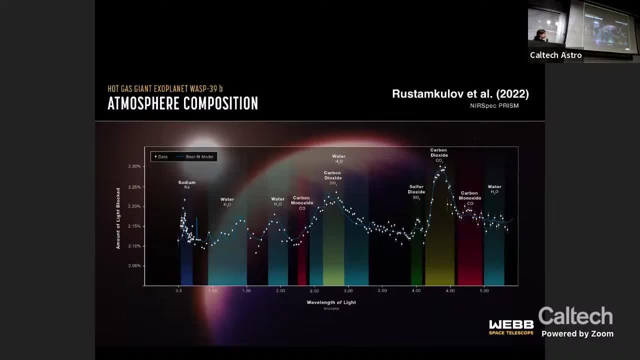 that's coming out from JWST. This is a transmission spectrum from a giant planet that was led by my pal, Zafar Rustamkulov. In it they saw just a bunch of stuff. OK, we've got sodium, water, carbon monoxide. 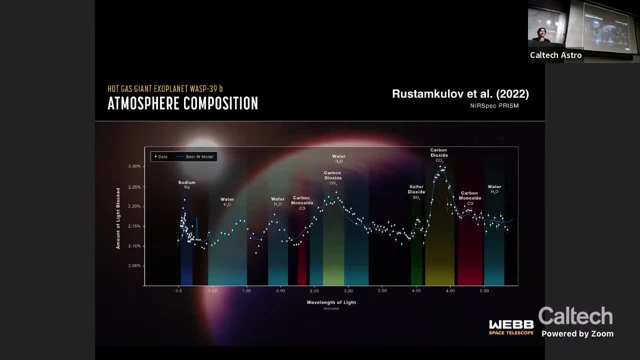 sulfur dioxide, carbon dioxide, more water- Just loads of stuff in there. A lot of this stuff we've never been able to see in exoplanet atmospheres before. So who knows, Maybe there might be other hints of atmospheric escape in other weird things. 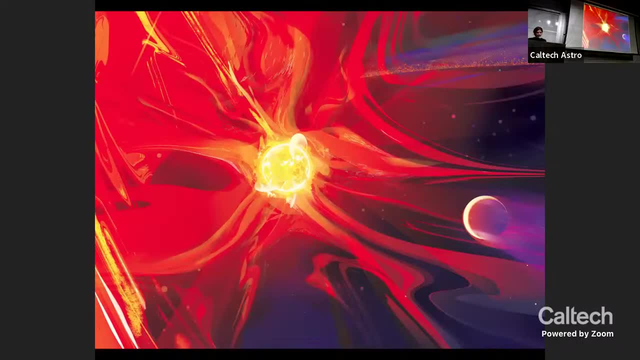 in these planet atmospheres. So can exoplanets keep their atmospheres long enough for life to evolve? I don't know. We don't know. Sorry, I don't have an answer to that question today, But we are trying to approach this. 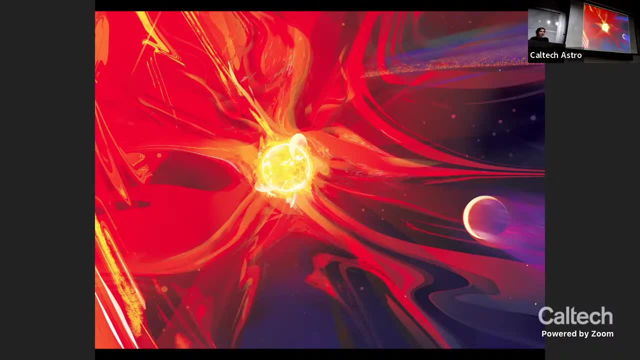 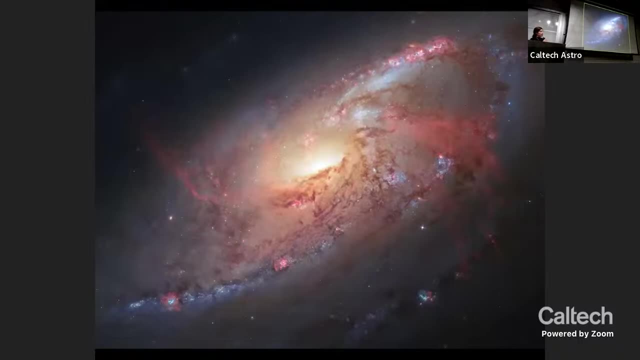 from every possible angle And today I've just highlighted like one angle that we could go at this from. So I'm an academic and sometimes being an academic is pretty hard. There have been quite a few times in my life where I have really struggled. 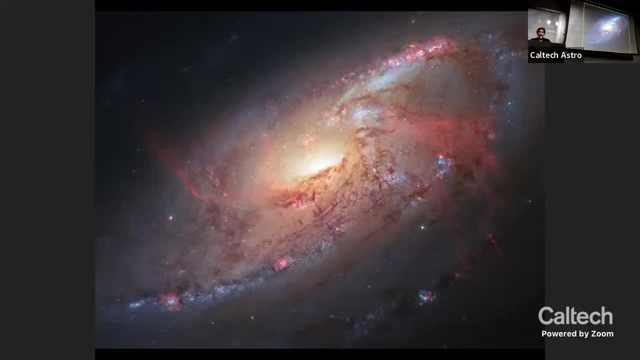 with this job and really felt quite alone. I have this image as my desktop background and very rarely I close all my windows on my computer and I see this, And this usually happens when my computer crashes because of all of those windows that I have open. 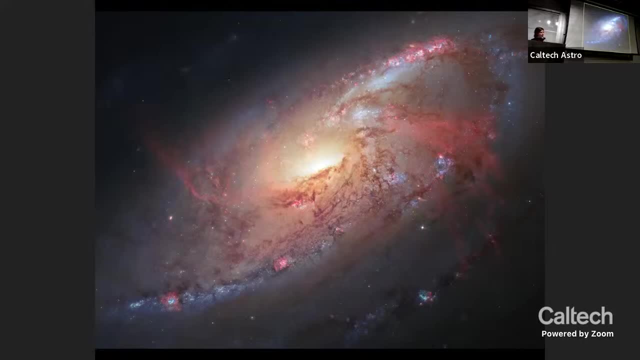 Anyway, when I see this, I'm reminded that I am a miracle. I am a tiny, fleshy creature somewhere in a galaxy like this and I'm going about my day and I have my weekly meetings with other tiny little scientist creatures, And we sit around. 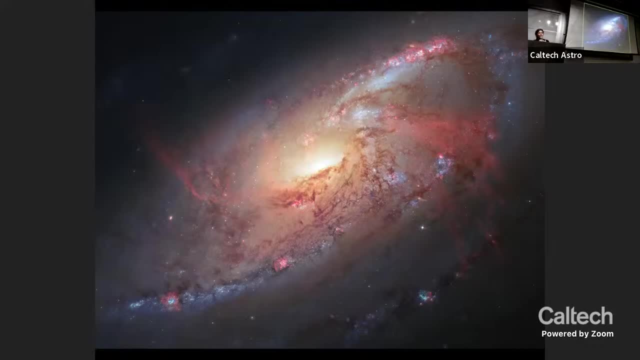 and we like shake our weird guitar voice boxes at each other and we vibrate the atmosphere at each other. We make these sounds and we nod our heads and we make weird sounds back at each other And we're sat there and we're really curious. 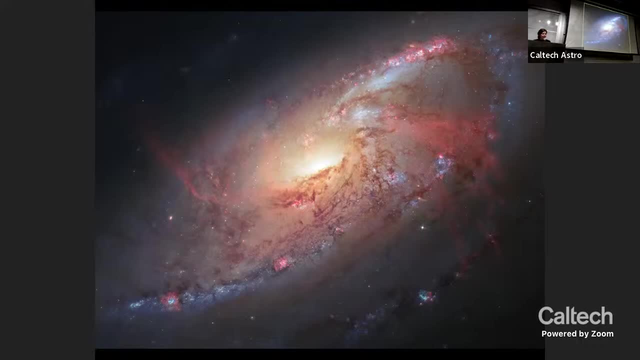 We're like, are there any other weird scientist creatures out there? Like let's have a little look Just for the fun of it. And in moments like that I feel very lucky And I look at the number of stars in this galaxy and I look at the number of galaxies. 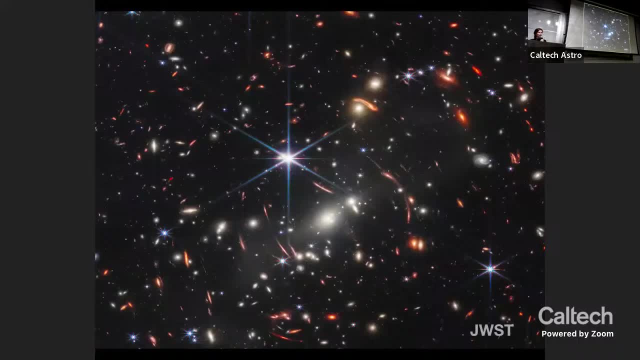 in this tiny patch of sky that is the size of a grain of sand held out in an arm's length, and I feel the opposite of alone, And it's moments like this, moments like sharing this with you, wobbling the air at you. 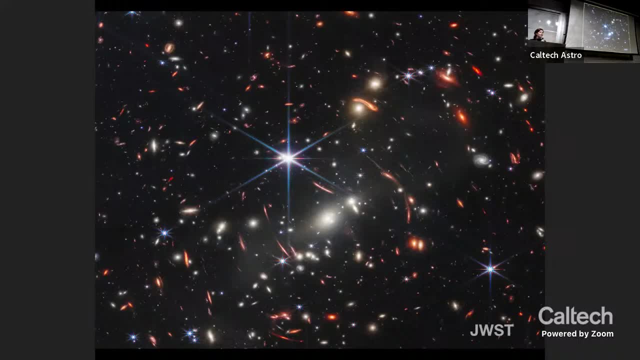 and hopefully receiving some of your wobbles back. They really keep me going and make me feel very lucky to be doing what I do. So thank you very much for coming here today despite the horrible rain, And I'd love to chat more with you afterwards. 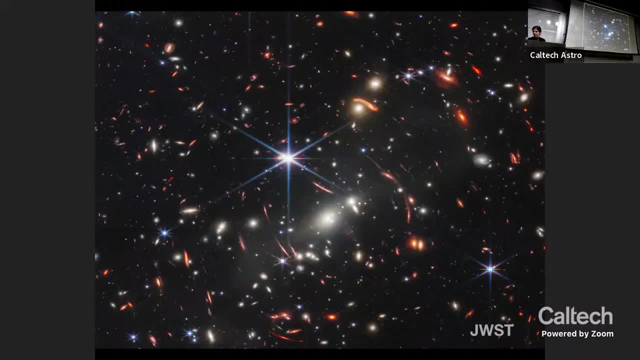 So, thanks, I will be taking questions, apparently. Yes, Hello, Hi, Just to make sure the online audience can hear us. So, going back to those stars, and when we saw the increase of, I think it was like the solar winds and other like phenomena around the stars. do we know why it's upwards of like 40% of the M type stars that experienced this, but not the like G type or the other ones? Yeah, That's a really great question. We think it's because the structure of these stars is actually significantly different. So inside a star, there are, like these different zones. There are these zones where there's a lot of like mixing and churning and there are these zones where they're just like more like stable layers, right These depending on, like, the size of the star. some of these stars have like a big region where it's just these stable layers, and some of these stars have a bigger region where it's like churning and mixing. For the smaller stars, we think they have a way bigger. much more of the star is this churning. 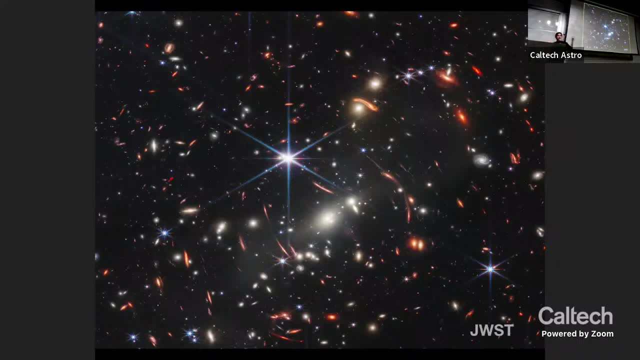 and like mixing region And it's that churning and mixing that generates these changes in the magnetic field lines. So it's like these huge magnetic fields at the surface of the star. It's a lot of like motion happening And it's those 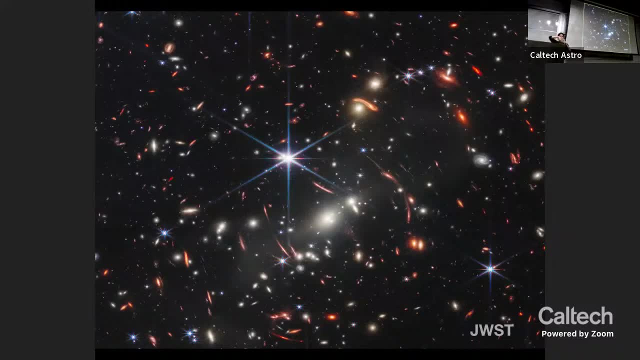 what happens to create these kind of explosions is there's those magnetic fields lines. that gets like they bunch up and they cross over And when they cross you have these like huge things. So that's what we think is why It's basically that different structures. and there's more magnetic fields and they're more violent that way. Does that answer your question? This question is about exoplanet detection, not necessarily about the atmospheres, but when you showed the animation at the beginning of the time lapse of discovery of exoplanets. 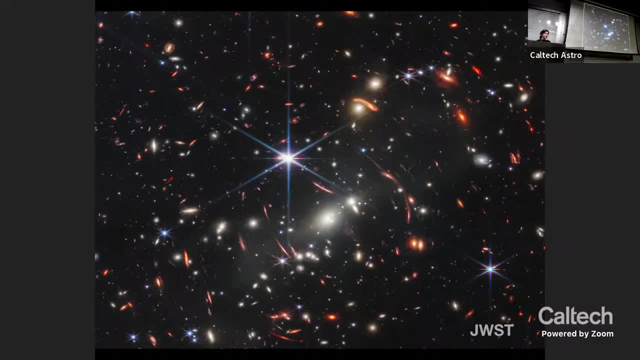 in the top left there was a breakdown of the method of detection And in the earlier years the radial velocity method was, you know, like four or five to one dominant over transit, And then at a certain point you can see but significantly before tests, maybe when Kepler was launched, transit eventually blows by it and becomes like four or five to one. So my question, two questions Prior to whatever instrument led to that spike- Kepler or something else- how were transit detections happening? 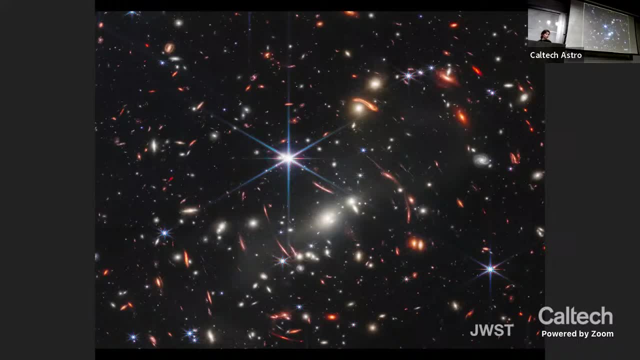 Like what kind of telescopes? And then, second, why did the radio? why does the number of radial velocity detections remain pretty static? I would think that, like over 30 years, it would be refined to where you'd see an increase. Even if you saw an exponential increase in transit, you'd still see some kind of increase, proportionally, of radial velocity too. Those questions make sense. Yeah, And those are both great questions. I'm going to actually answer the second one first. The second one is actually kind of a function. 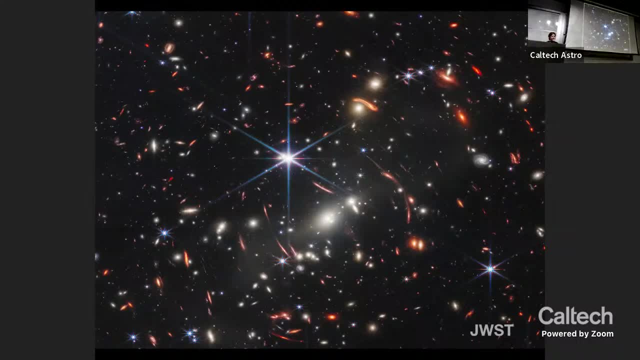 of, just like human accident. So the question is, why was it radial velocity And why was that not steadily increasing? So finding planets with a radial velocity method? So just to explain to everybody else, radial velocity when you look at a star and a planet system. the planets go and run the star for sure. But the planet's gravity is also affecting the star's gravity. It's also affecting the star. Like as the planet goes round, its gravity makes the star wobble, And so we can see those wobbles. 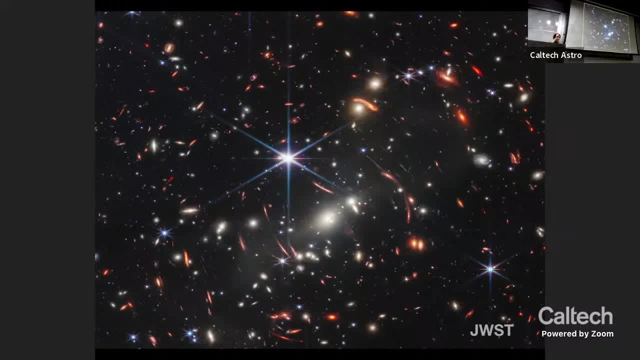 these tiny wobbles and that's how we can detect planets: by seeing these star wobble. So that's the radial velocity technique. That technique is way more expensive and difficult than the transit technique. You need to use spectrographs. You've got to get the whole spectrum of the star. and you've got to see it shift. You've got to monitor it for a long time. see these like ups and down wiggles. It's difficult, But that was the first way that people thought that we would find exoplanets. Because we had an idea that most planetary systems looked like the solar system. And for the solar system, honestly, the easier way to detect planets for the solar system is the radial velocity technique. Because the planets are so far away, the chances of them transiting is very low, right. 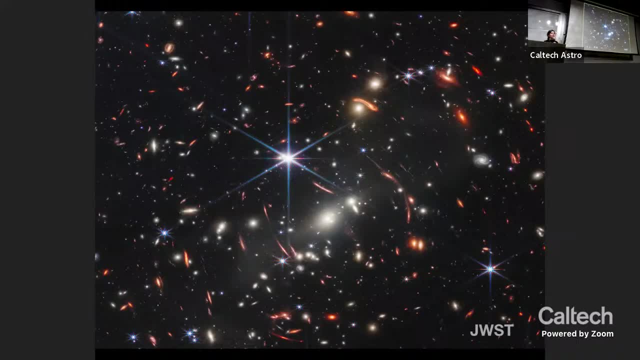 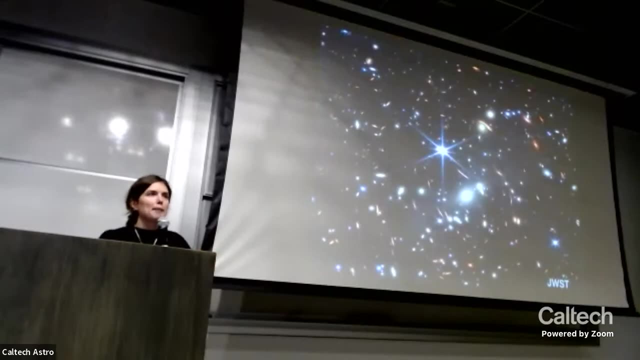 So that's why we started with radial velocity. But then, when we used radial velocity, the first planet that was found with this technique was an absolutely massive Jupiter-sized planet that took like a few days to go around its star. We literally had no idea that these things existed. 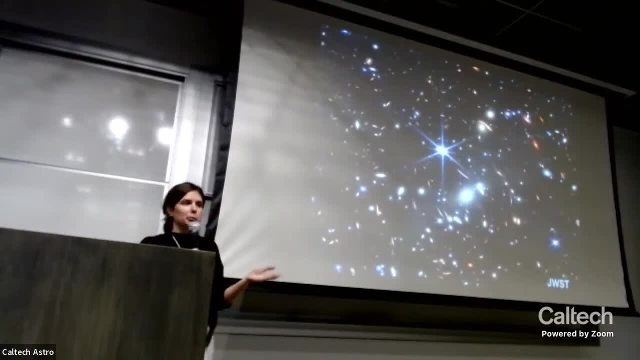 It was a huge surprise, And so we were like, oh okay, we should be looking for these things now. Those things are way easier to find with the transit technique. It's way cheaper. You just take a cheap telescope. All you're doing is measuring the brightness of the star. 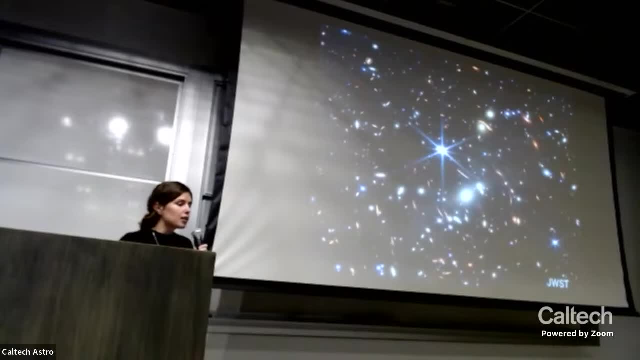 If it's a big planet you don't even need a very big telescope. So then there was a big rush. to answer your second question: what were the other things that were looking at finding those transiting planets before TESS and Kepler? So there were like in the late 90s, early 2000s. 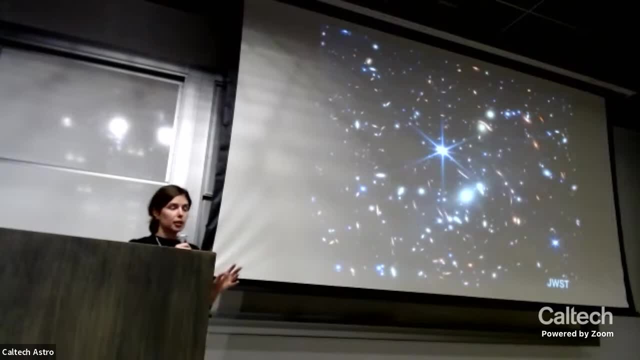 people started building these quickly, these very cheap transit surveys, using basically off-the-production-line cameras. They just pointed them at a star out of the sky and just measured the brightness of basically every star in the sky that they could see ground-based from the ground. 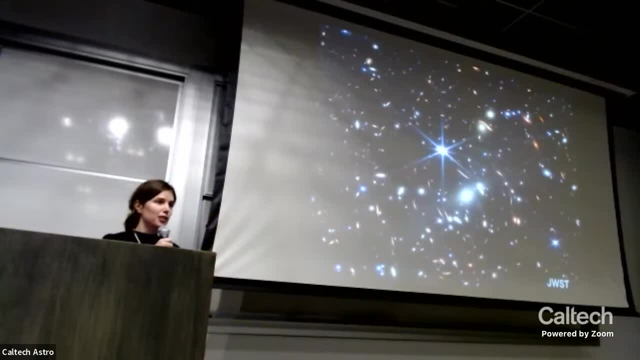 It was amazing. I actually used to work with one. It's called the WASP survey, the Wide Angle Search for Planets, And actually WASP is like it was a really good, is a really good transit detection one. So then the transits like shot up. 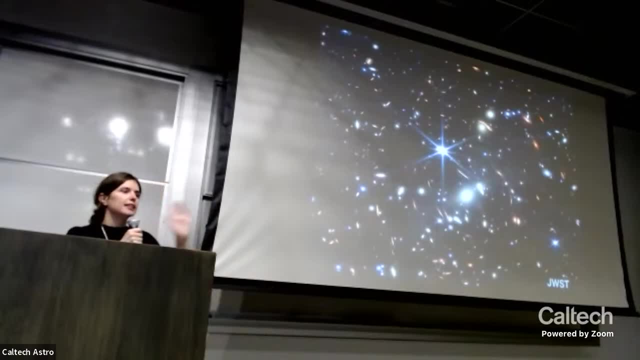 They found like a few hundred. like the earliest, the easiest planets you could find, There were these massive planets around bright stars that orbited like once every few days. Yeah, So that was a long answer. Did that answer your questions? Okay, cool. 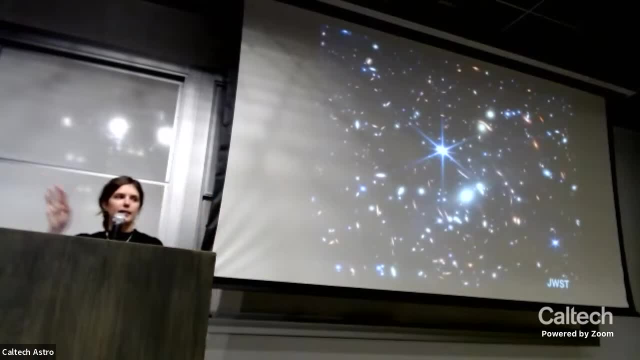 Oh yeah, Sorry, But the reason why radio velocity hasn't like shot up as well is because it's like really expensive, Like yeah. Yeah, I think that's the main reason, especially as we're also so we're trying to measure the mass with the radial velocity. 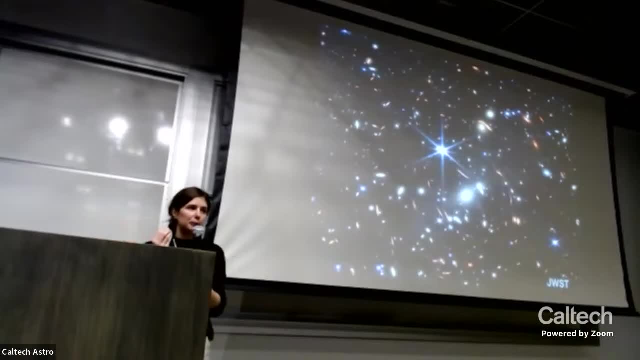 And, like smaller planets, need like a lot more telescope time to measure that mass. You're also limited because the star is like I showed you. the star is like crazy, like violent stuff, and that messes up the observations as well. Yeah, No props. 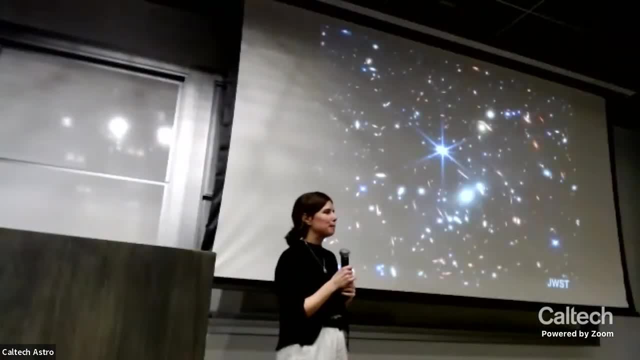 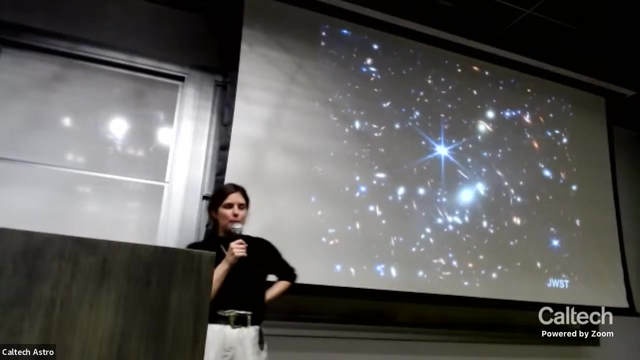 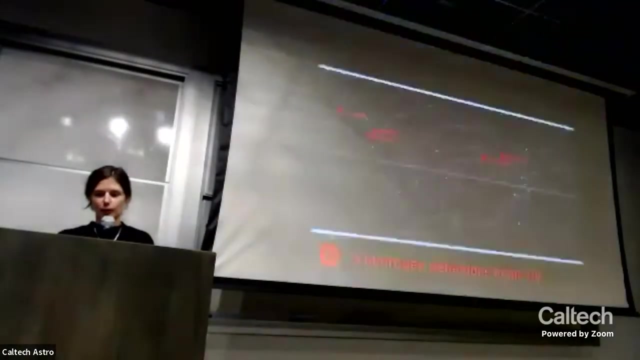 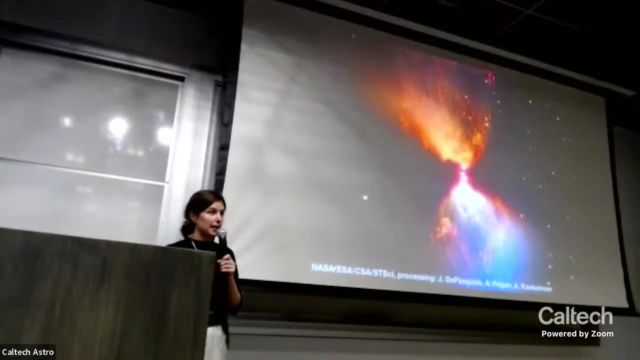 Hey, So how do animal forms? Ooh, great question, That's a tough one. So when planets form- Oh, am I still showing? All right, planets form right around baby stars. When they do that, there's like a lot of gas and material. 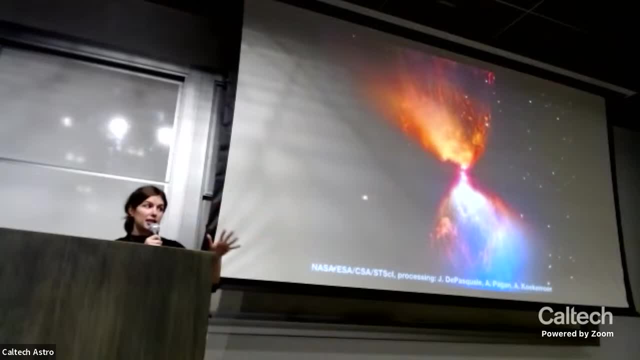 that's still hanging around, And so we think we're pretty sure that when these planets form, they like suck up a bunch of gas as they're swirling around the star Now, at some point the star will heat up the rest of the gas. 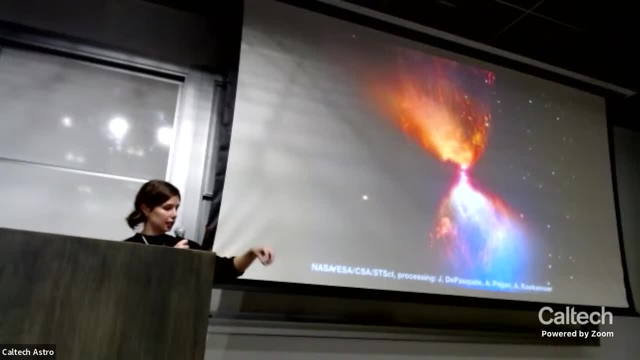 and it'll all disappear, And so you'll just be left with the star and the planet with some gas that it's captured, And then all of this other stuff disappears. We don't know if the planet holds on to that original atmosphere that it just picked up from the same stuff that made the star. 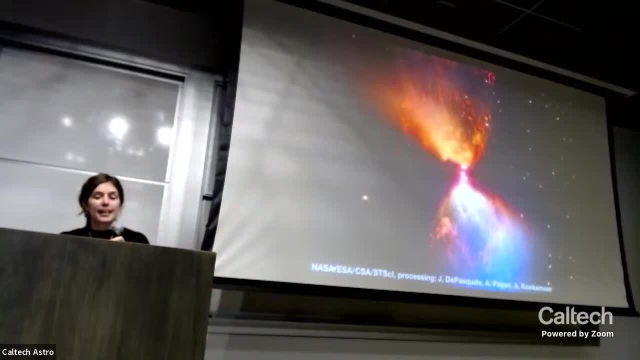 It might lose it to space again And then it might form a different atmosphere. So on the Earth we think that some of the stuff in our atmosphere actually came from the rocks and volcanoes that like exploded up, basically some atmosphere from the surface. 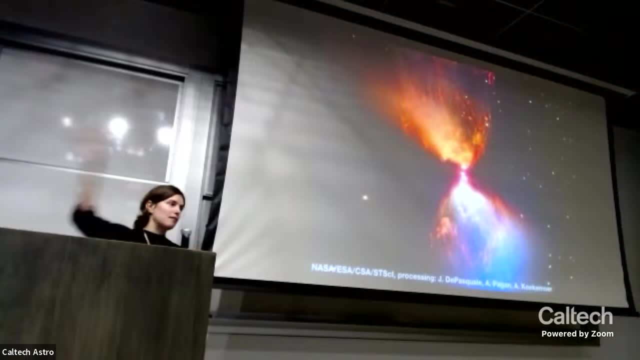 Also, sometimes there might be comets that come out of space and crash into the Earth and like dump a bunch of water on the Earth's surface And that becomes So. in short, there's a lot of ways you can form an atmosphere. 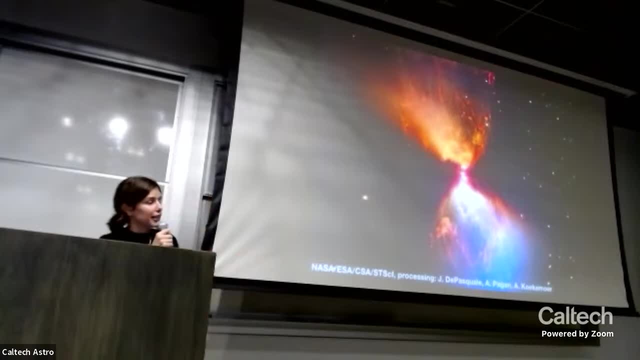 And it's pretty hard to tell for which planets where the atmosphere came from. So we're trying to answer that right now. That's a great question, Thanks. One more question from the audience before we switch to the Q&A panel and field questions on all topics. 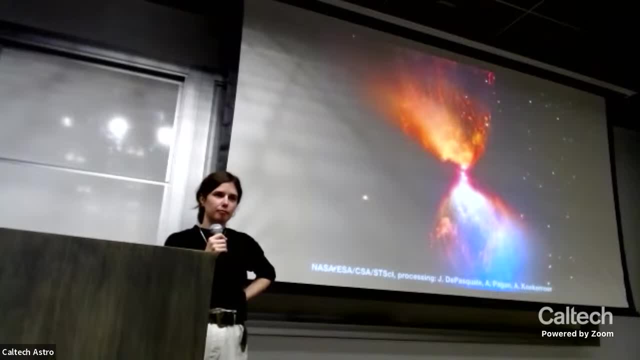 Hello, Thank you. You talked about how some atmospheres could have been there and then disappeared. Do you also Like? is there a way to tell if it's disappeared at some point And, if so, like? would that be useful? 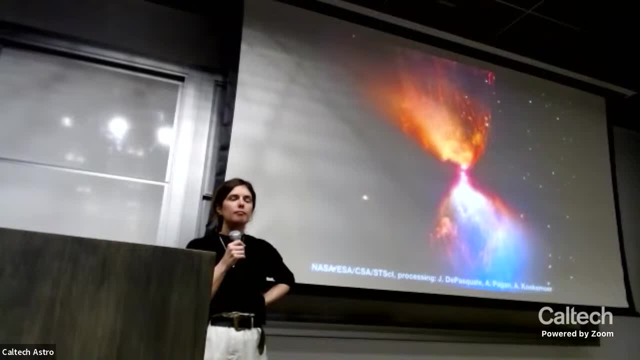 if you found like signs of liquid water or life, Like, is it significant to your research? Yeah, Also a great question. So in astronomy we have the benefit that we can look at like a lot of things, But we can only see those things right now. 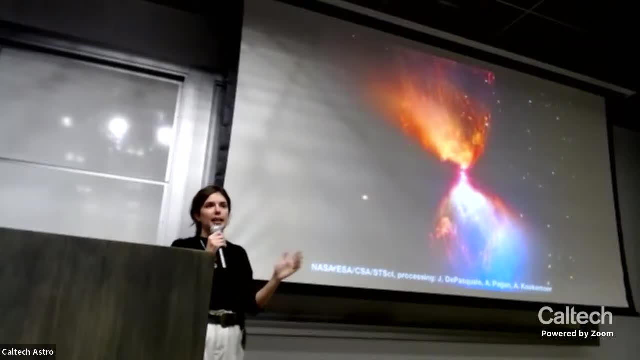 We are not able in astronomy to like run experiments, to like wind back the clock to see if there were, you know, for a given exoplanet. it's pretty hard right now to say what was its atmosphere like previously. So we can try and get around that by just looking at loads. 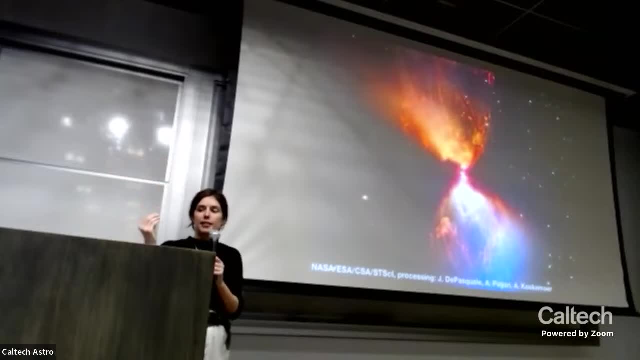 and trying to find very young planets, Like we try and find very young. We try and find planets that are like all the different evolutions that we've seen in the past. Yeah, We try and like piece them together Like we don't know, but we can if we get enough of them. 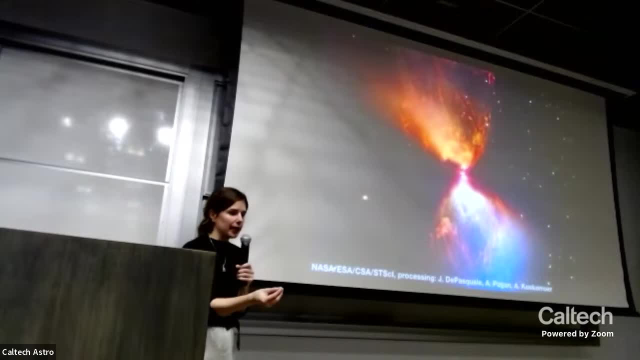 we can assume, this young planet will eventually turn into that old planet over there. They're probably about the same, But it's kind of through these methods that we're trying to figure out if we can piece those all together. You know, in the solar system we have an easier time with that. 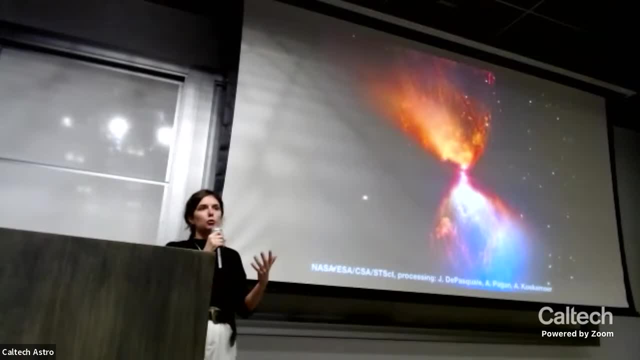 because we have like geological records of like the Earth, Like you can, you know, you can go to the Arctic and you can like dig into the ice, and the ice that was laid down like a million years ago is like really deep right. 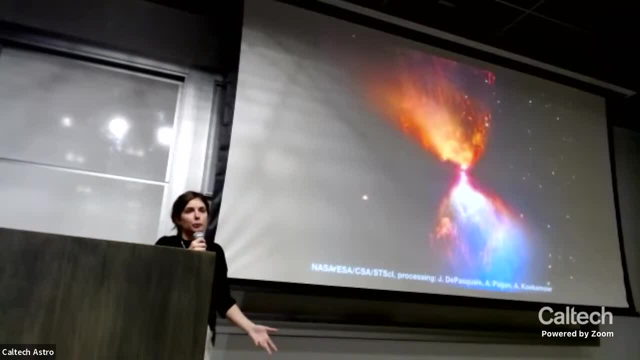 And you just dig that up and it will tell you what was in the atmosphere, like a few million years ago. It doesn't go that far back, But in that way we can, you know, turn back the clock on Earth's atmospheres. 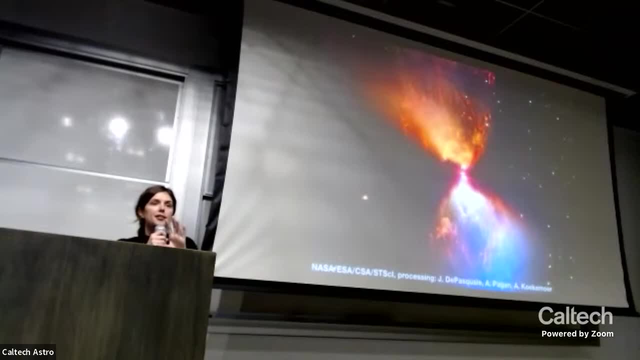 on the Earth's atmosphere which we can, And those lessons maybe we can apply to exoplanets. But yeah, it's really tough Like we also can run like models and try and wind back the clock with like theoretical models. 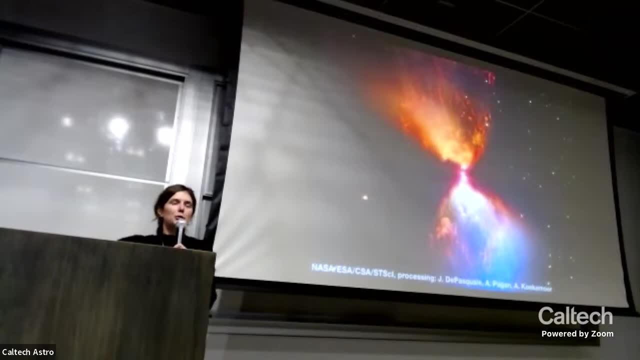 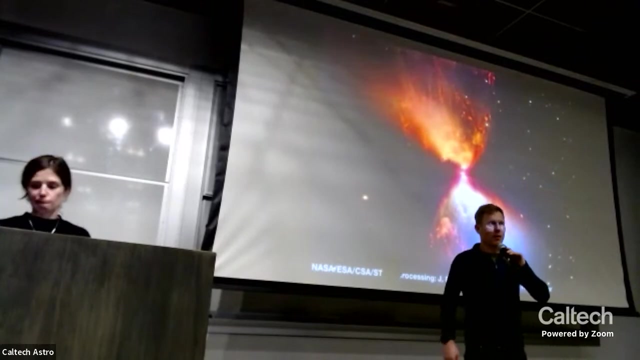 But yeah, it's still a work in progress. Does that answer the question? Cool, thanks, All right, We're going to move on to our Q&A panel. We'll get started in like three minutes or so, But please thank. a wonderful presentation by our speaker. 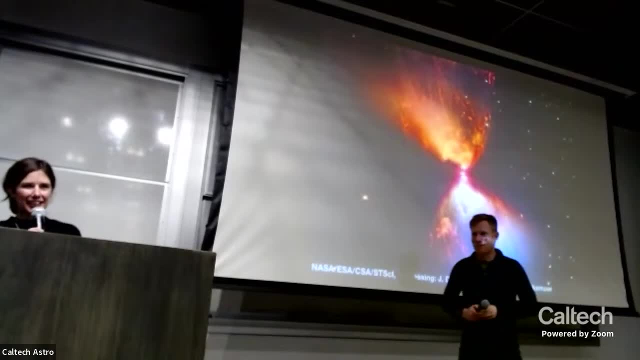 Dr Jessica, Thank you very much. So if you'll just be patient, we'll set up a table, We'll turn the lights back on, get rid of the screen and we'll start. You guys don't have to. For those of you who showed up late, 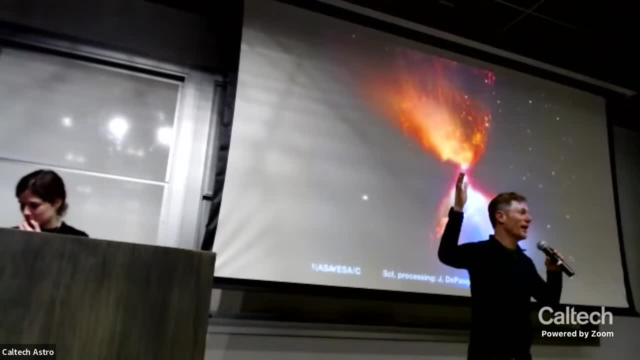 in case you didn't notice, there are clouds and rain overhead, so we won't be having the telescope viewing. Oh no, I'm not trying to give you a hard time, I'm just saying we don't have the telescopes tonight. 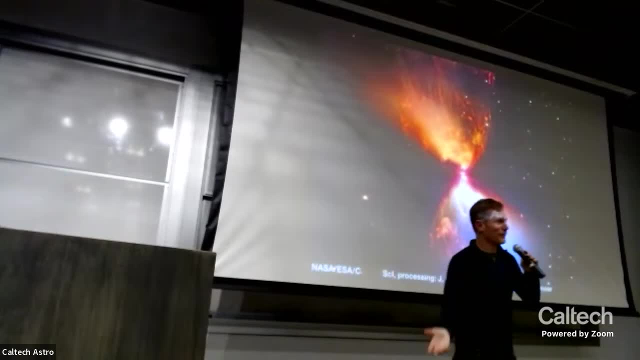 because atmosphere, our own atmosphere. But we'll still do the Q&A panel. You guys are welcome to stick around. You can take off. if you just came to see the highlight of the night And there have been about 15 questions on YouTube. 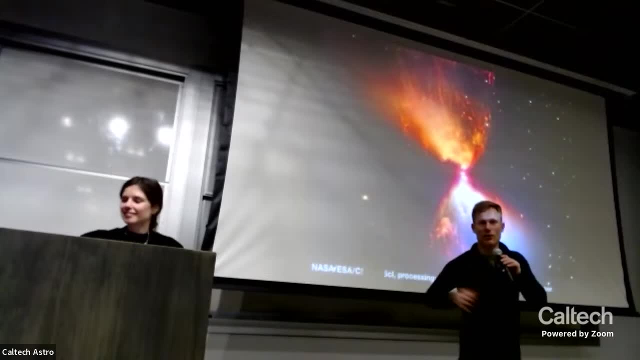 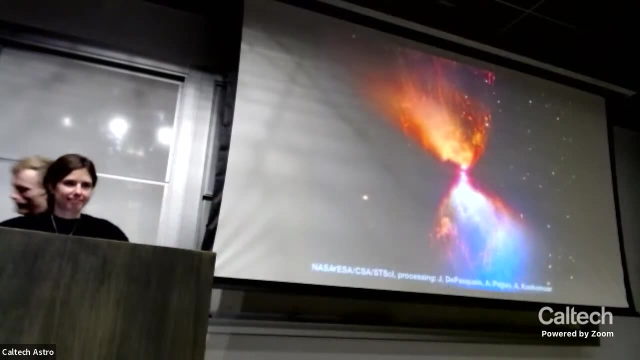 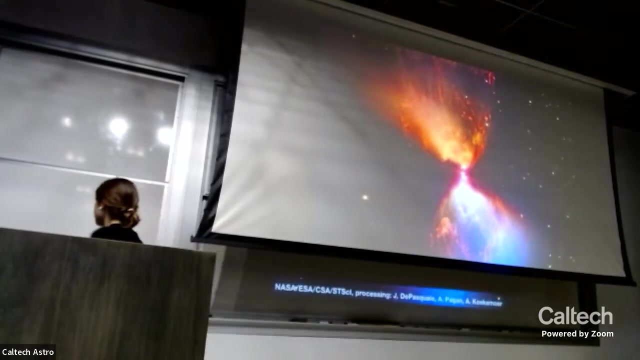 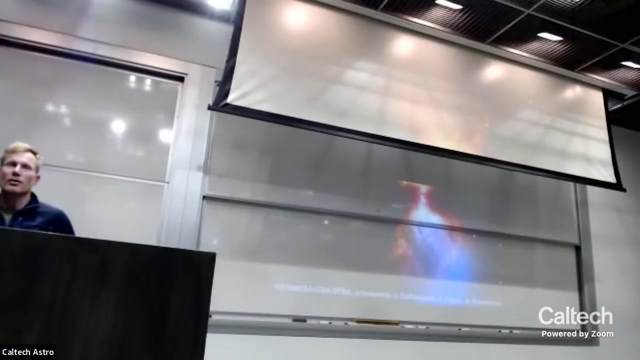 that I haven't yet asked, but lots of relevant questions that are really, really good. So we'll introduce our panel in just a moment. And yeah, just to start off the first question: are you feeling like you're seeing anything different? 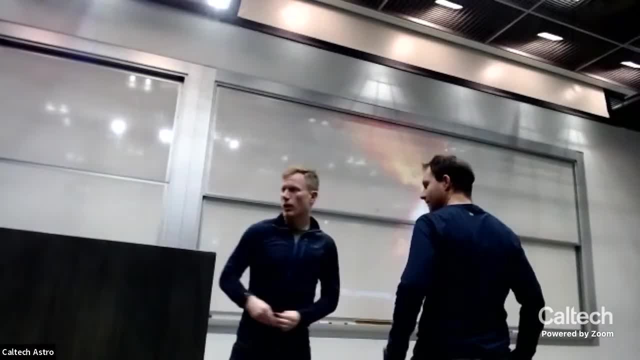 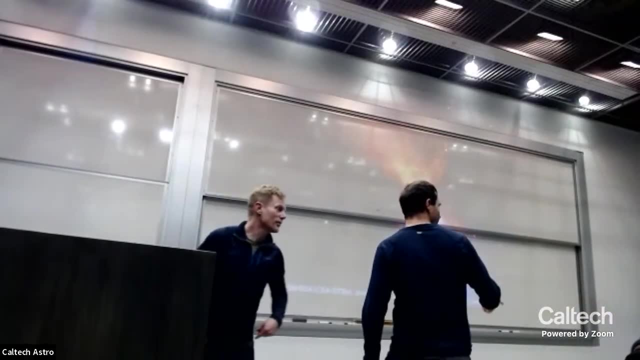 on the camera. I'll try to make as clear a comment as I can, but I'm really, really happy to be able to share it with you today. So we're going to try to finish off the Q&A right here, And the very last question is. 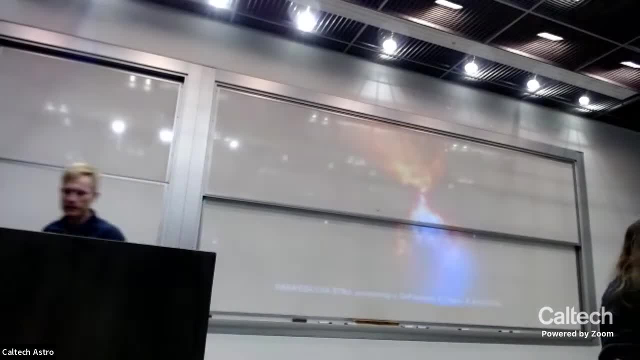 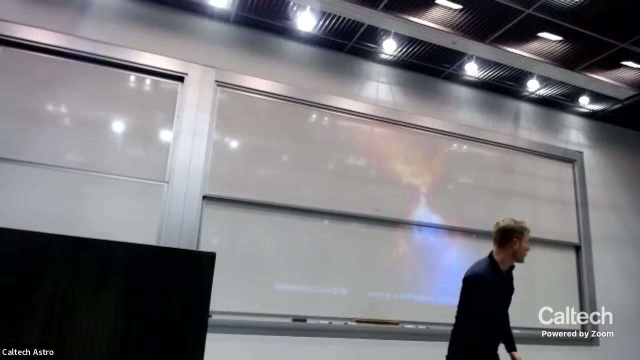 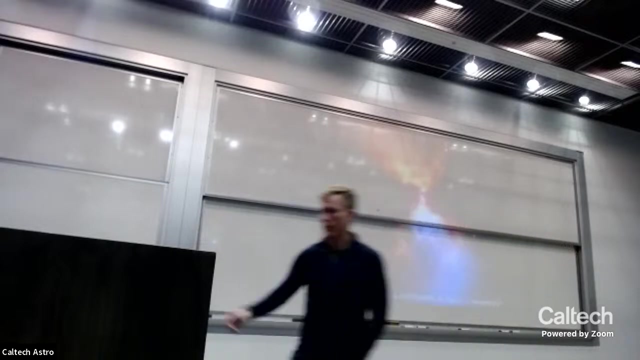 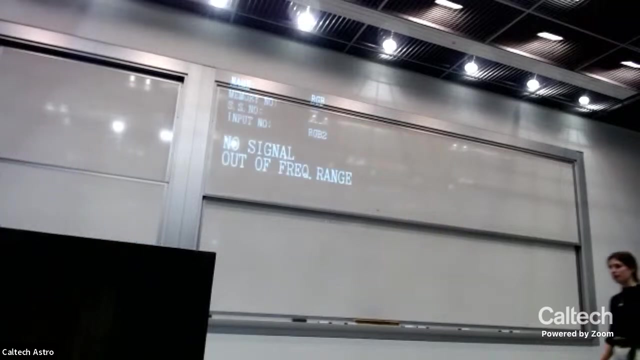 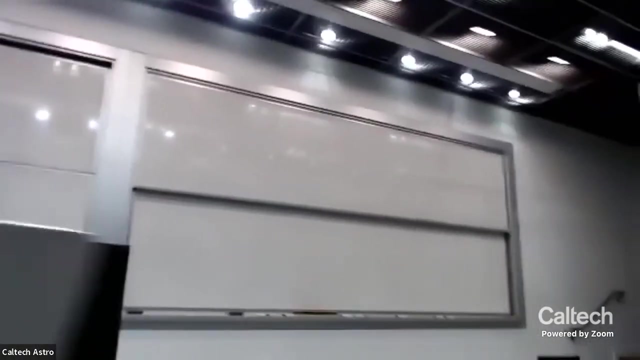 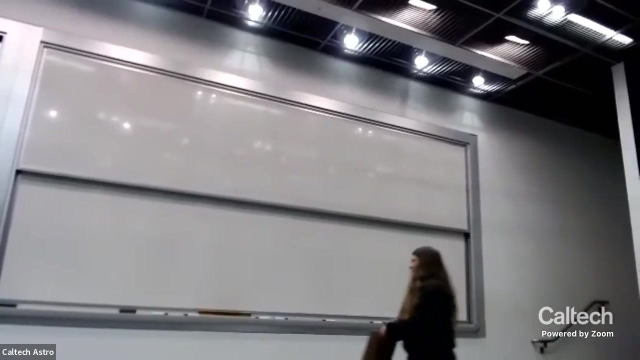 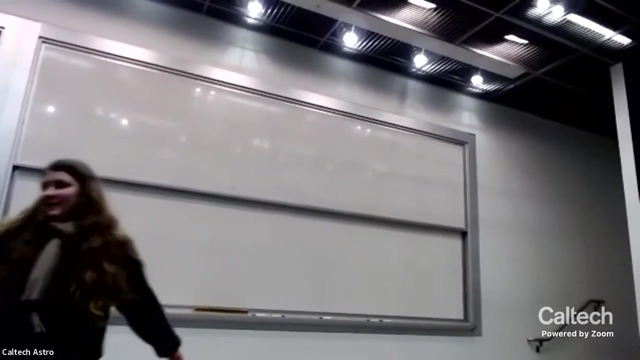 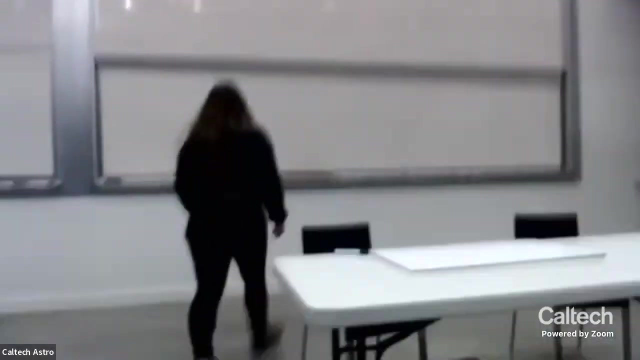 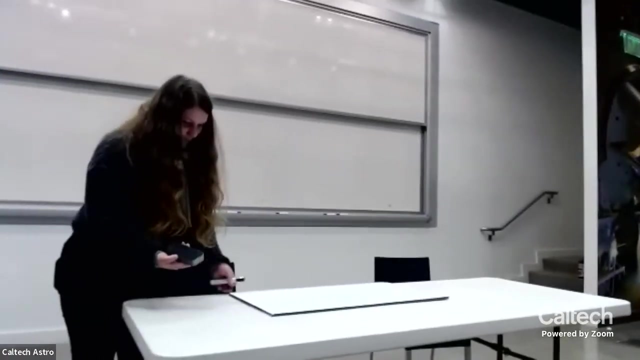 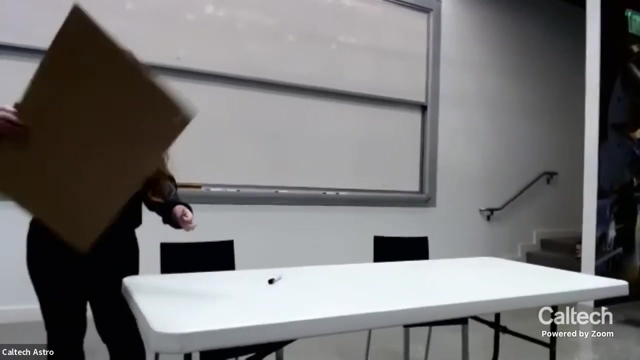 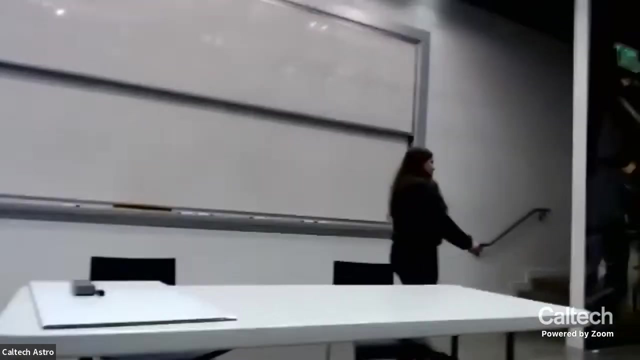 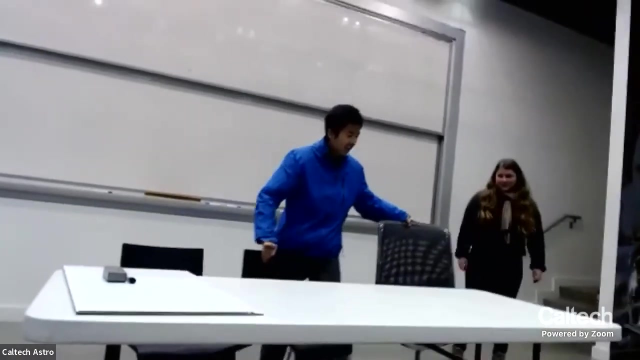 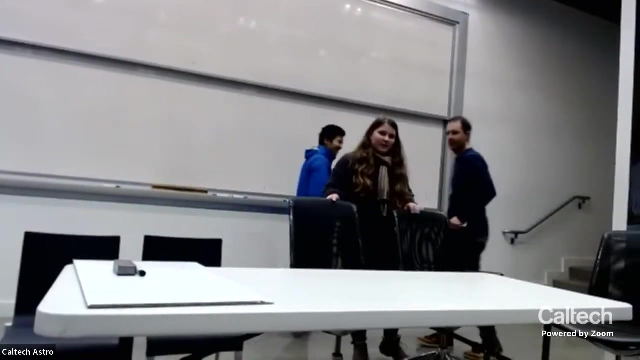 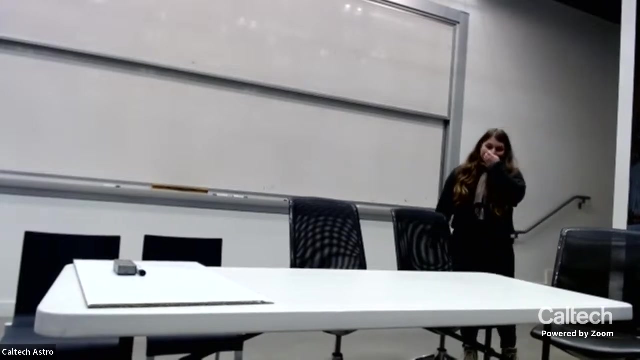 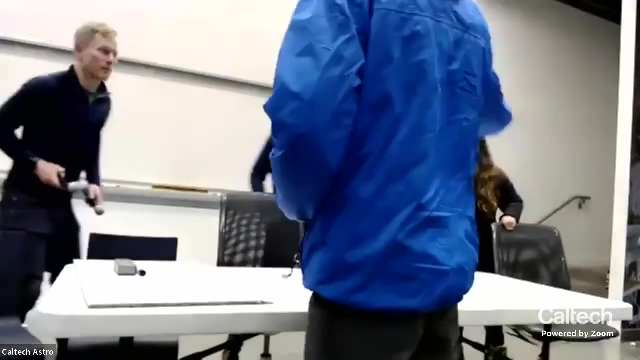 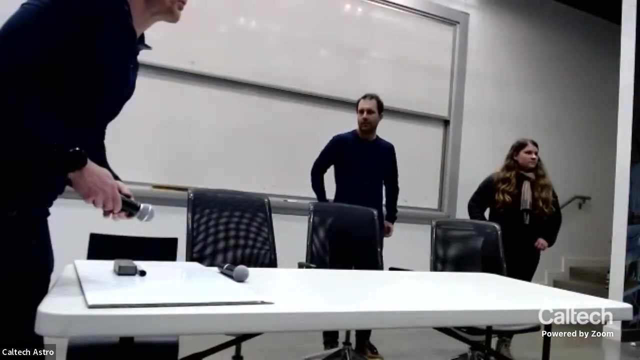 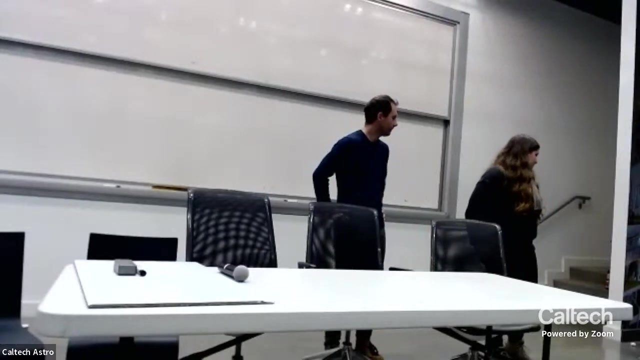 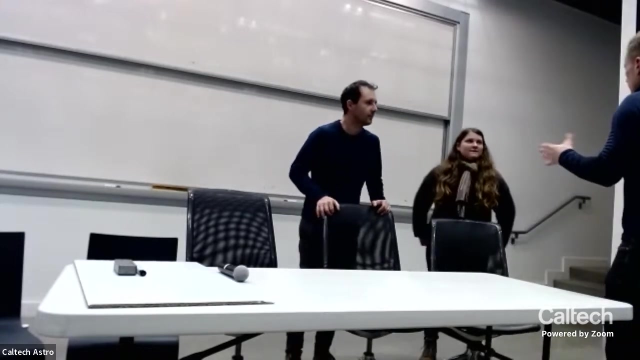 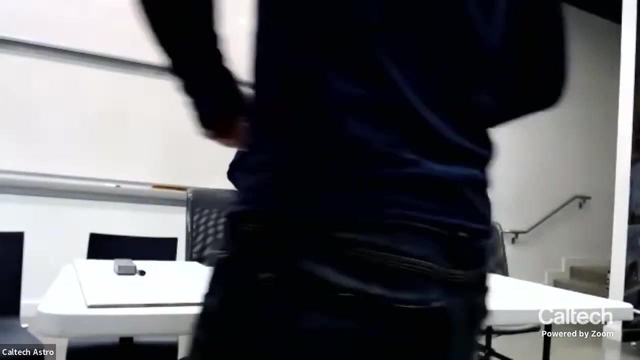 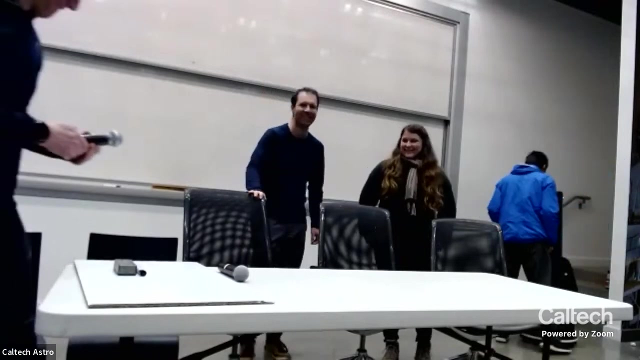 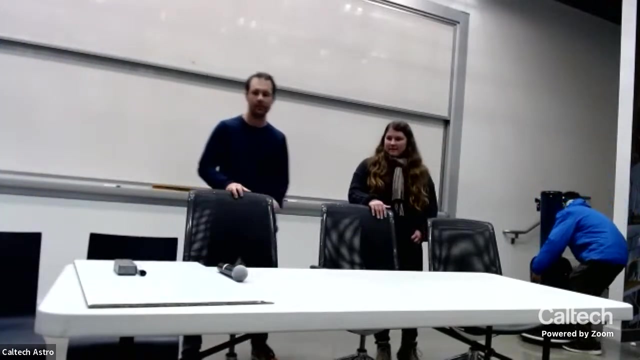 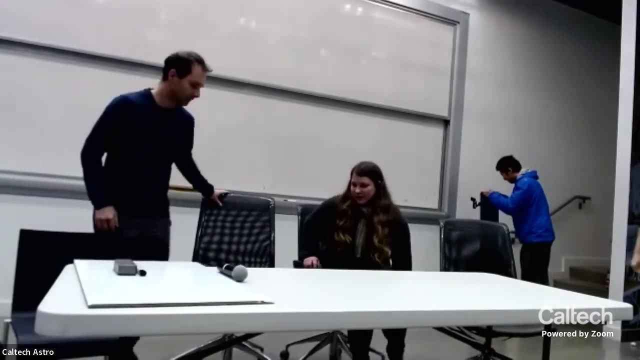 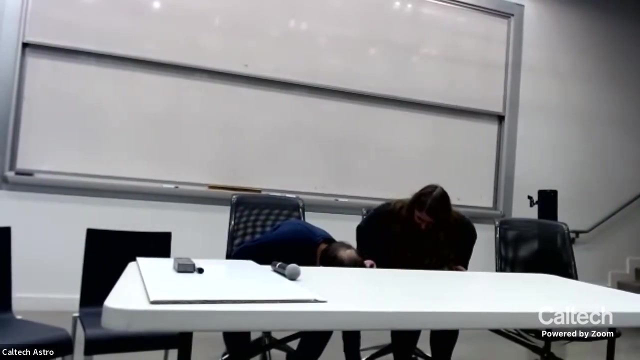 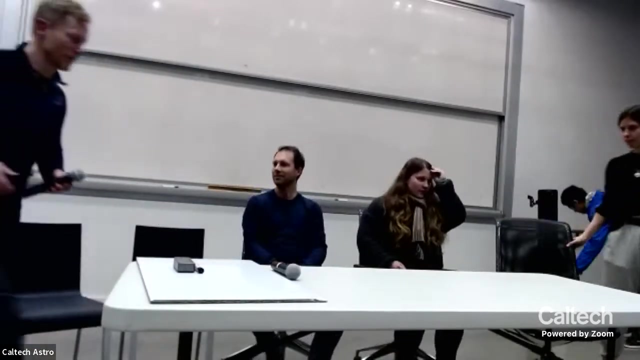 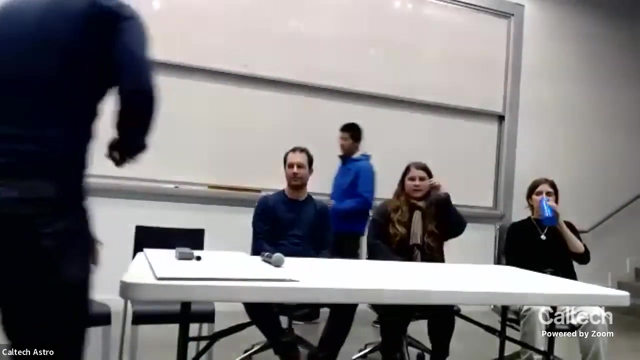 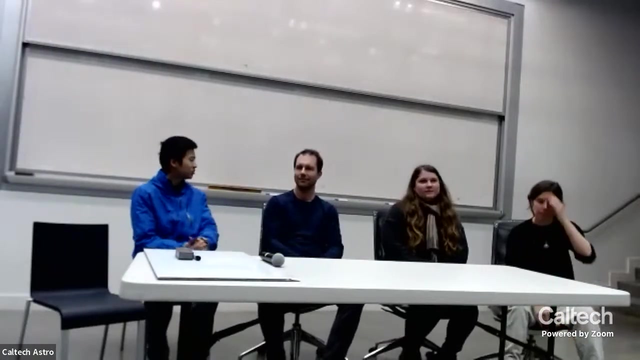 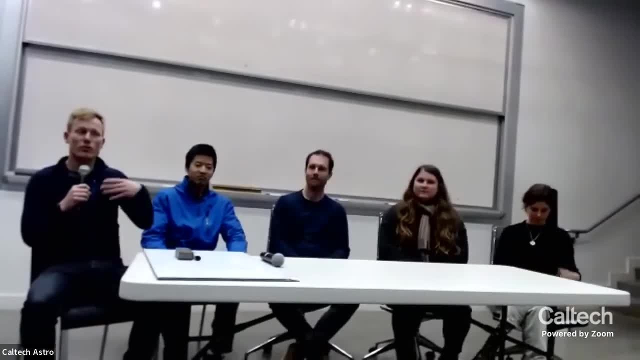 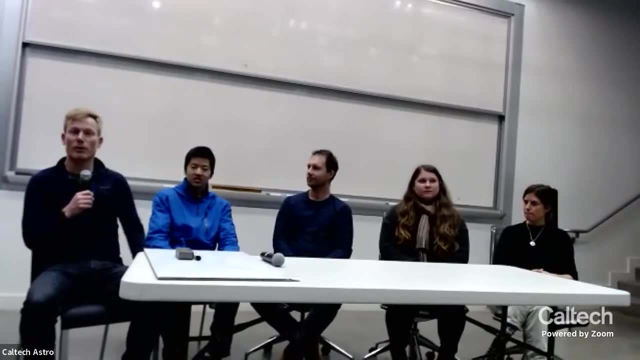 um, all right, so here's our q a panel. we'll just go through and everybody introduce themselves and give a brief introduction to the kind of science that we do, because we all do different science from each other, and i think we do actually. we we took a census beforehand and we, we we cover a. 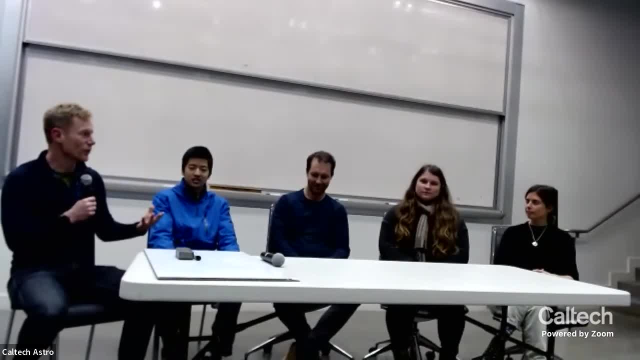 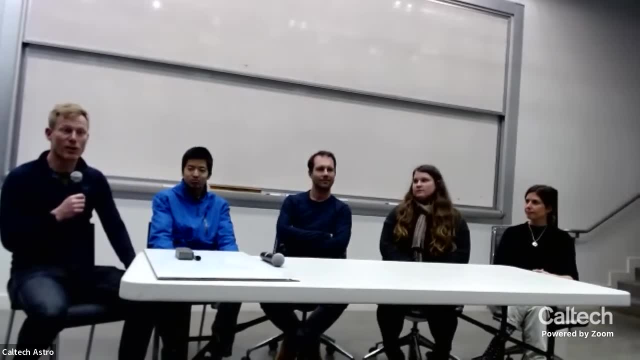 pretty broad part of the spectrum of astronomy and astronomical topics amongst our various different specialties. so i'm cameron hummels. i do mostly computational modeling of how galaxies form and change over their lifetimes and do a bit of cosmology alongside that. so like how the 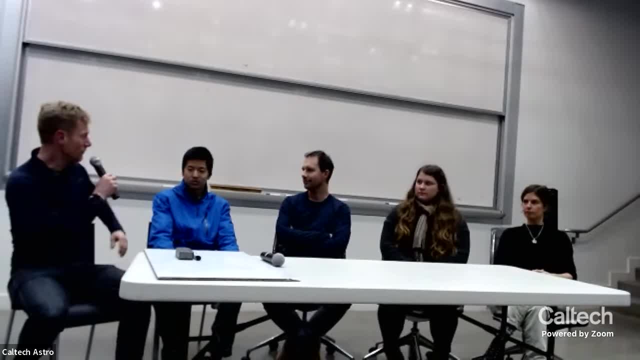 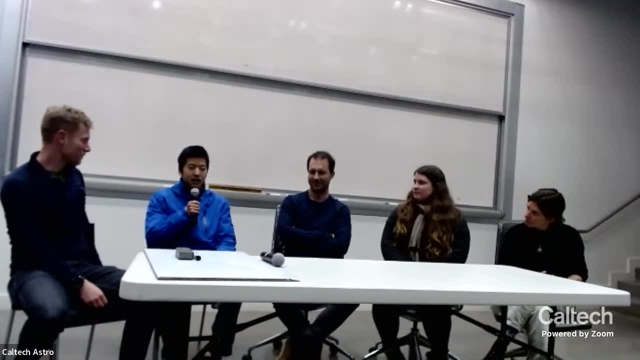 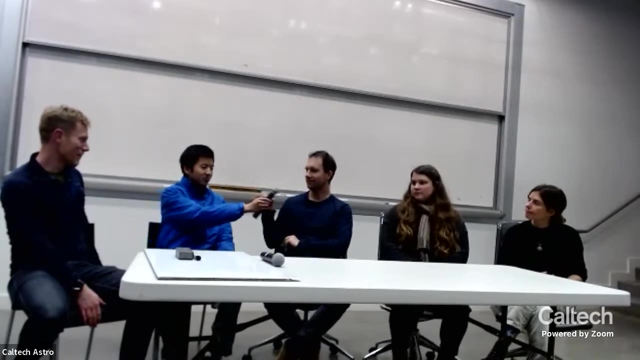 structure of the universe changes over large scales as well. um, and somebody who does something very different. hello, i'm ki chang. i'm a phd student here in planetary science. i work on comets and asteroids and related objects in the solar system. hello, my name is andreas feist. i'm originally from switzerland, but now i live in california. 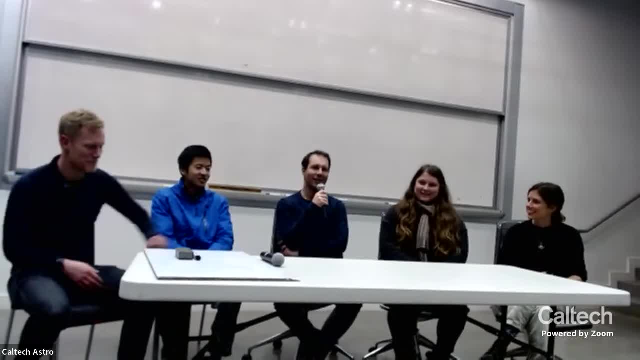 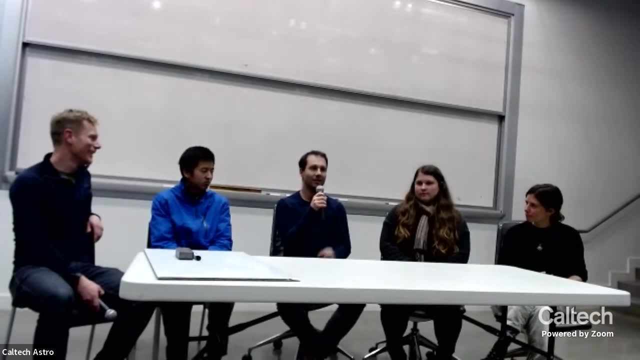 where it's um. i look at the first galaxies that are being formed in the universe. so they're very, very tiny little dots that you might have seen on the new jwst images, the tiny red dots. that's the stuff i'm looking at. my name is sam rose. i'm a phd student in the astronomy department. i'm broadly 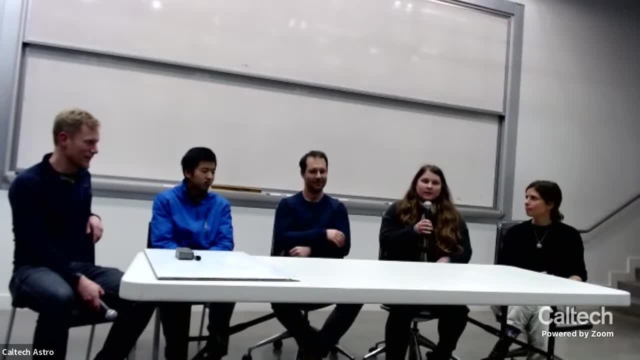 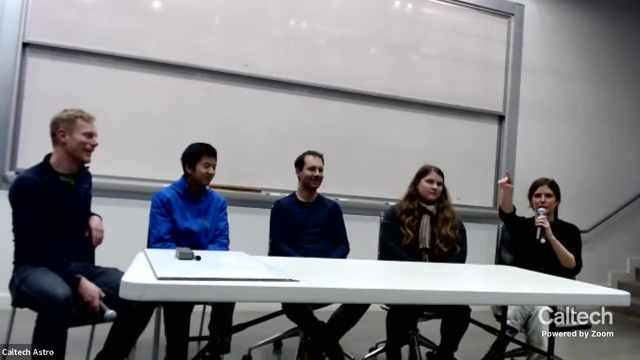 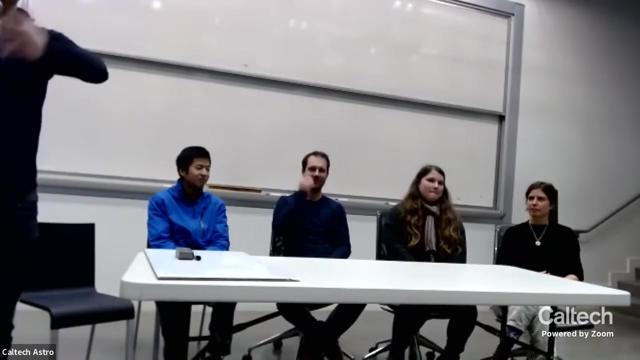 interested in explosions and the things that will explode- so massive stars- and the things that have exploded- so neutron stars and black holes. hello, i'm jessica spake. i study exoplanet atmospheres and i'm a postdoc here. actually, over the road, it's all one in the same. um, okay, so we can take questions from the audience in case. 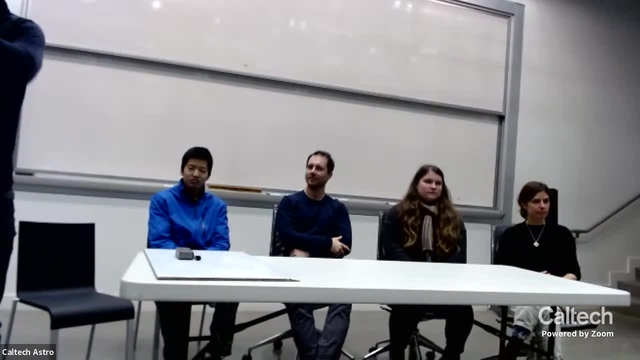 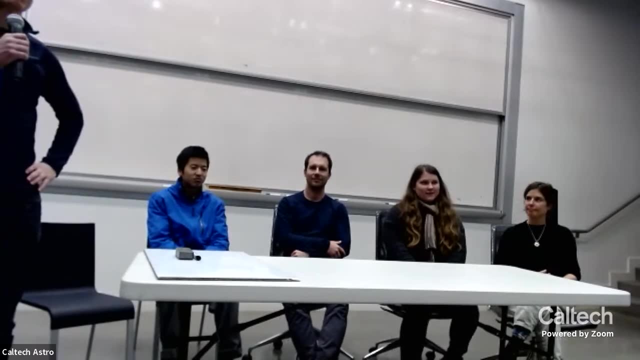 you didn't get yours fielded thus far. um, and i also have a number of different questions that have been asked online. in case you guys are like let's take a break for a second, let the online people so do you, i'll give preference to the on to the in-person audience. are there? there's questions. 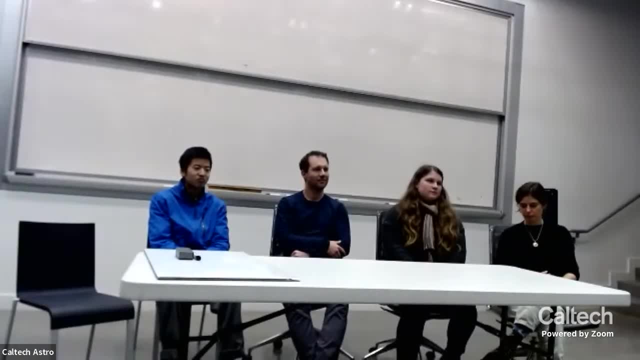 okay, um, just based off, like you know, our big bang model and everything when the universe first started, um, i think it's a question for you- is, uh, when it's based off how it expanded from like you know nothing, basically, um did, do we know, or do we think it expanded like? 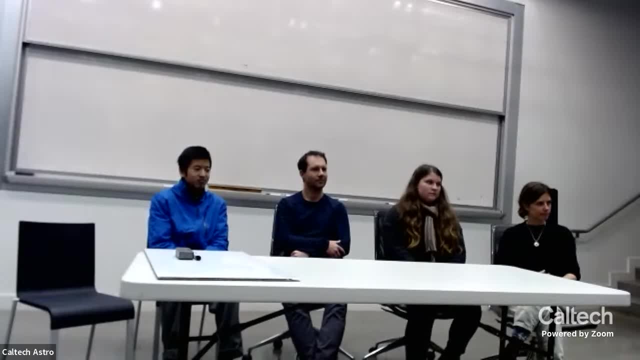 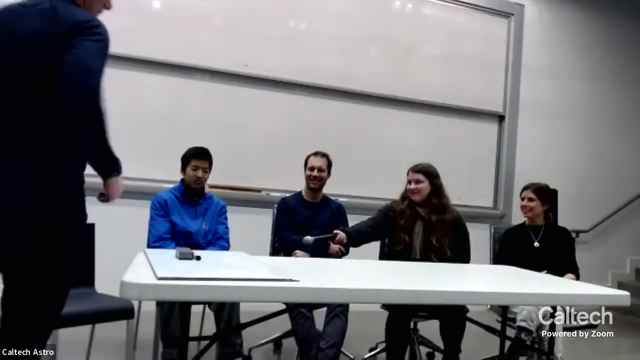 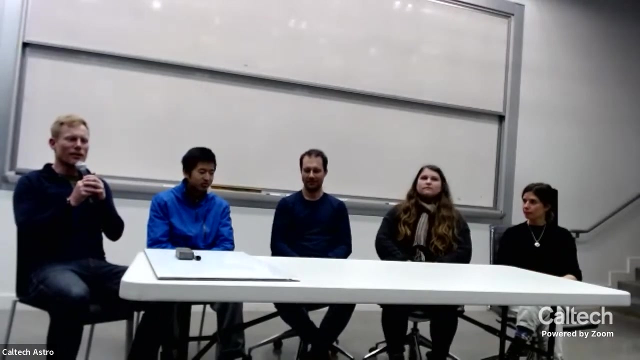 like perfectly in like all directions or some areas expanded quicker or slower than other ones, and how did that affect, like, the structure of the universe? oh yeah, okay, okay, okay, um, challenging, challenging question. uh, so basically, did the universe expand uniformly, both in terms of its speed at which it was expanding, but also its direction or their? 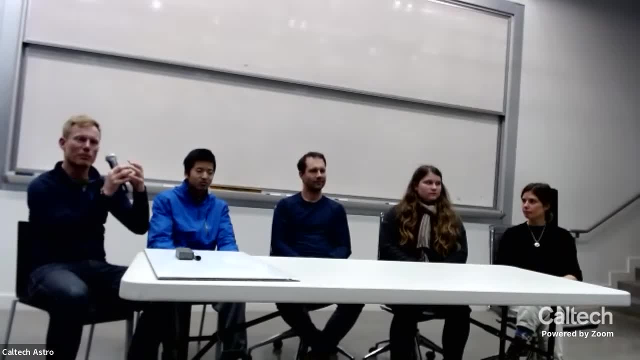 pockets where, where potentially it expanded faster in this pocket than over here, like okay, i don't think that we have a ton of evidence one way or another. i think in general i'm sure andreas can chime in on this because he works on early universe stuff as well, but, um, we do believe, okay. so one thing that we 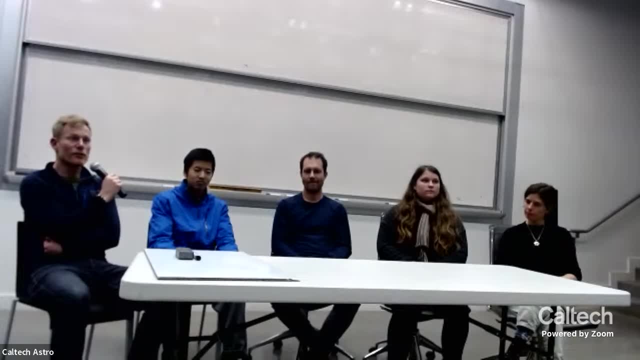 believe, based on several different pieces of evidence, is in a theory called inflation, the inflationary universe. so that means that in the very early universe, just moments after the kind of the birth of the universe and the big bang, that the expansion of the universe is going to be a lot more. 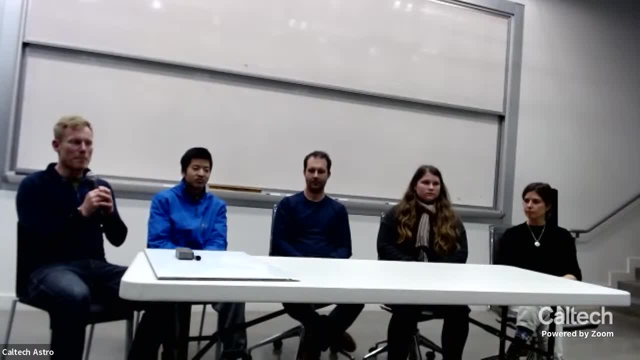 occurred exceedingly quickly, um, inflating really quickly and and the the time scale over which it is changed in its accelerate its expansion rate over the history of the universe. um, and part of that change in its expanding rate is attributed to something known as dark energy. um, so that is. 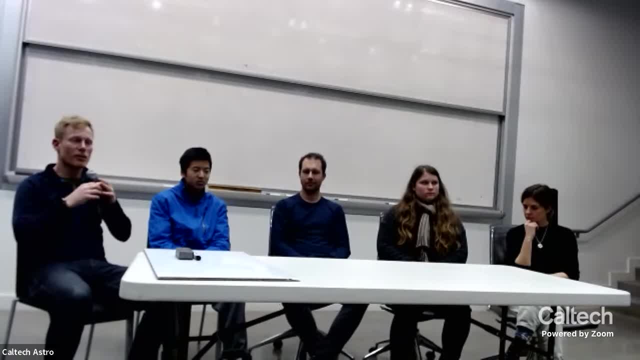 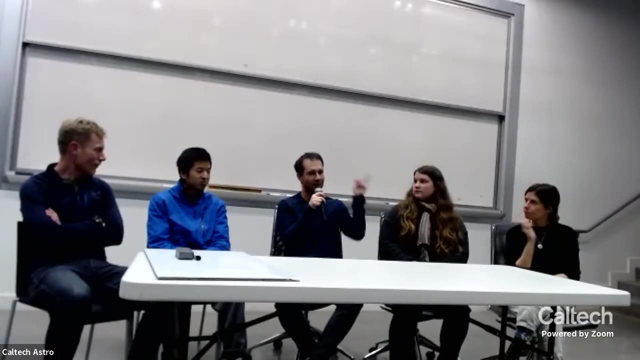 causing it to accelerate and speed up in its expansional, expansionary rate, um, but in terms of whether or not it's homogeneous, i don't know well, i mean, yeah, it's a good question. so one thing we realized is, when you look around, it's very isotropic, so there's not really a 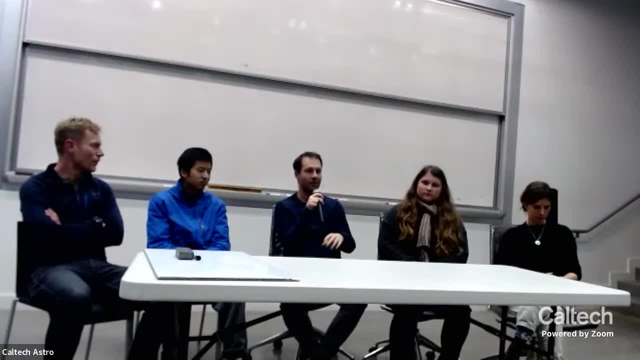 direction that it's preferred. or, you know, there's like a gigantic thing on the left or something like that right. so that's basically just describing the universe around us, right, and- and that was, uh part of this inflation theory, right, that it has to inflate very quickly. so it didn't have a chance to you. 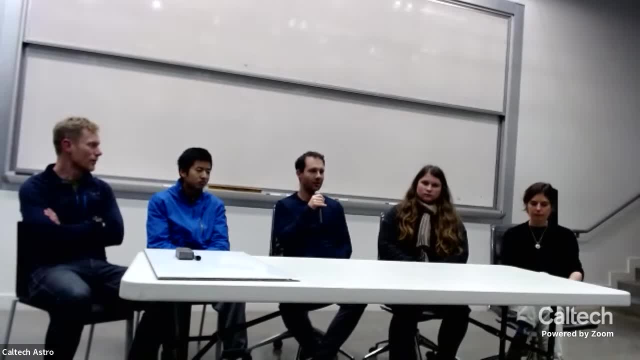 know, create this kind of clumps or asymmetric things in the universe? um, so that's from like observational evidence. but yeah, as cameron said, we don't really know, right, we cannot. yeah, it's like you're, you're standing in the forest, right, when you want to measure how big the forest is. right, it's kind of it's almost impossible. 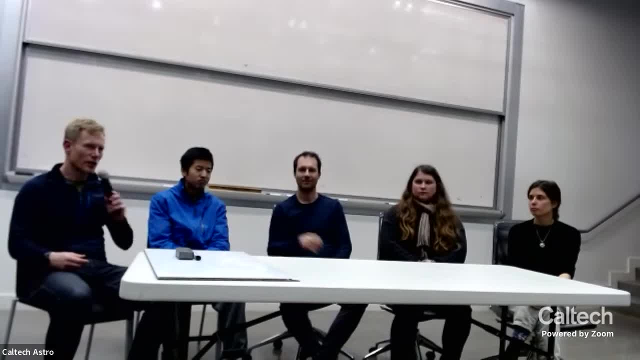 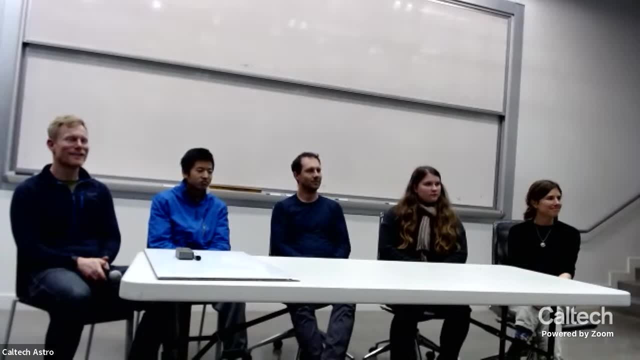 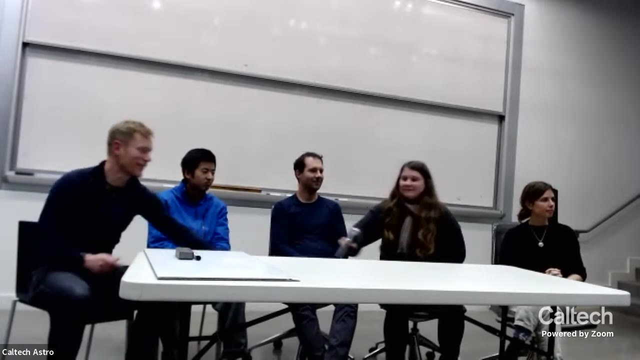 challenging question. and you, sir? so um, you talked about us being like little fleshy scientists here on the earth. let's say you're a little fleshy scientist somewhere else, not specifically. what would be your best way to look at the earth and identify that it was a habitable place, or um you? 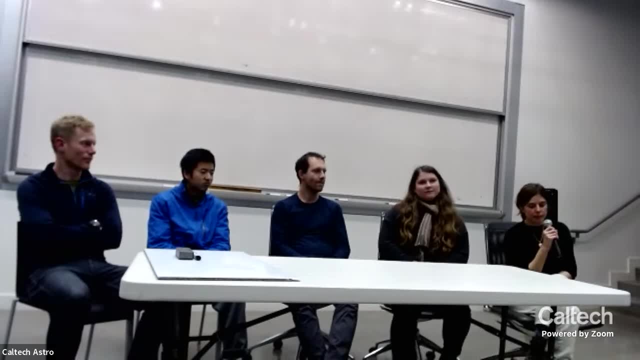 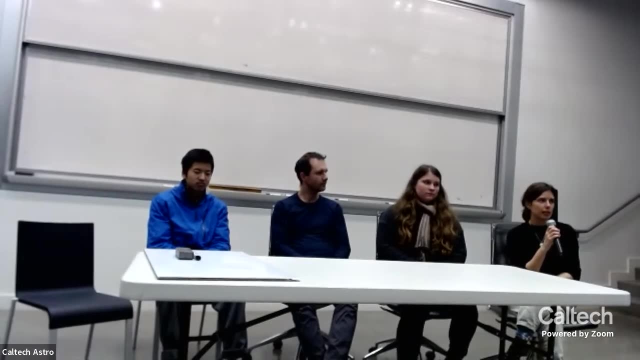 know somewhere where there might be life. um, i would say that the best thing would be direct imaging of that planet. so this is a really cool technique we have and it's just taking pictures of planets. it's really hard to do because the stars are so bright. you have to like block out. 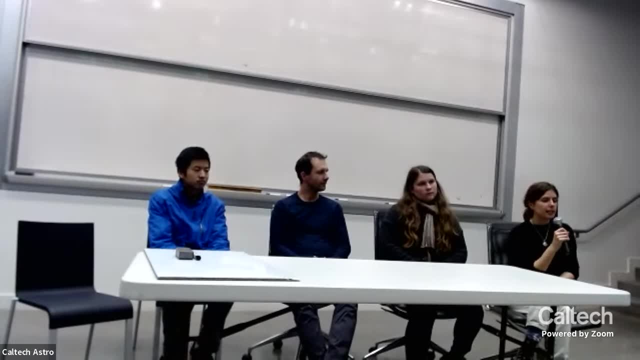 the light from the star. um, i think that is really the way that we expect: that we will be able to see truly earth-like planets in the future, and then, when you you do direct imaging, you can get direct, like the direct light that's coming from the the star. 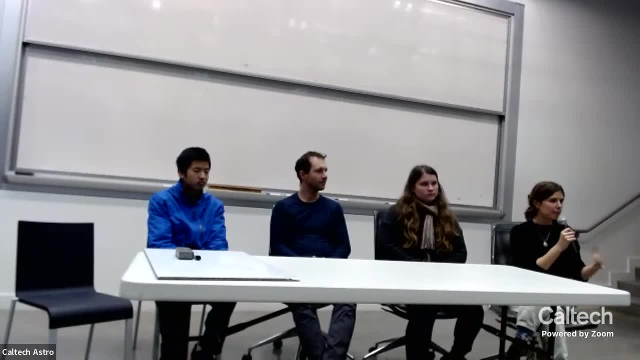 the planet, sorry, so you can kind of see its atmosphere. we don't think we're going to be able to resolve it, so it will still be like a single point, but we will be able to see, um, you know, break up that point of light into all the different wavelengths or different energies. 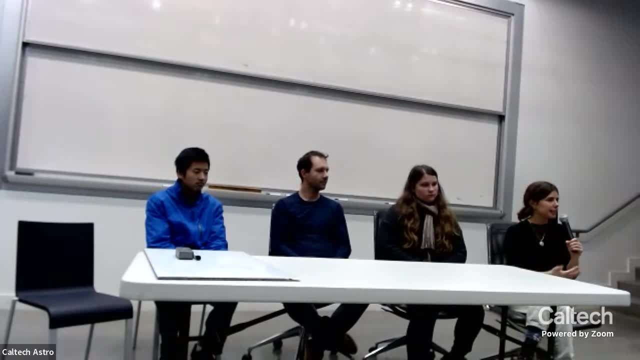 of light, we might be able to detect signatures in the atmosphere of those planets. you know, in the earth's atmosphere. all of the oxygen in the earth's atmosphere, basically most of it, came from life. it wasn't put there by the rocks and we have like ozone and like methane and 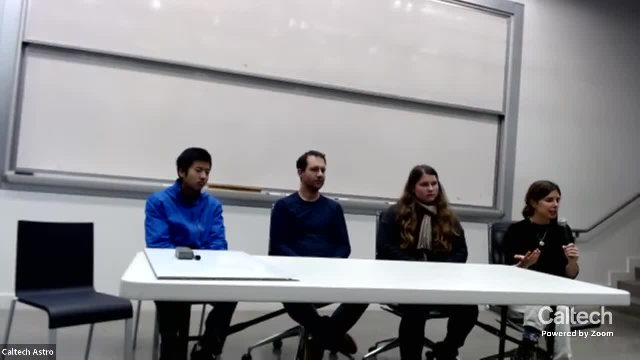 other stuff that life put in there. so people call those biosignatures, and so a lot of people think that the best way to look for signatures of life is by looking for biosignatures in the earth, in the atmospheres of earth-like planets, probably through direct imaging. we need, we don't have the 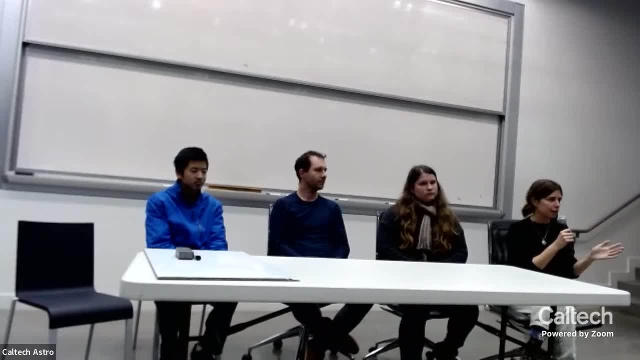 telescopes to do that. yet we need way bigger telescopes in space. we don't have, um, i think it's still pretty difficult, and i think to do that you really have to understand the atmospheres very well, because there are very many ways you can fake biosignatures. um, recently we found some. 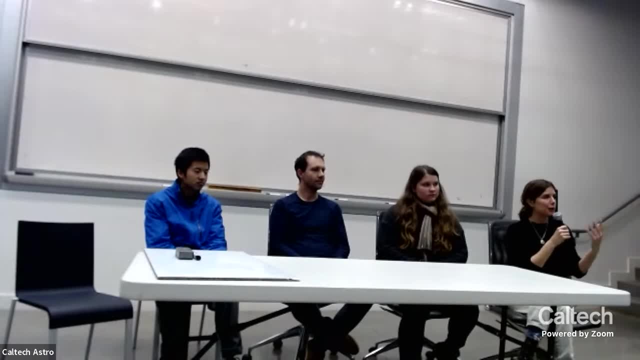 anyway it's. we need to really understand the atmosphere properly to know whether it's from life or from something else. um, oh, another question. oh yeah, it's just a piggyback off of that: if, if, if you were a, if you were, if there were intelligent life on, like say. 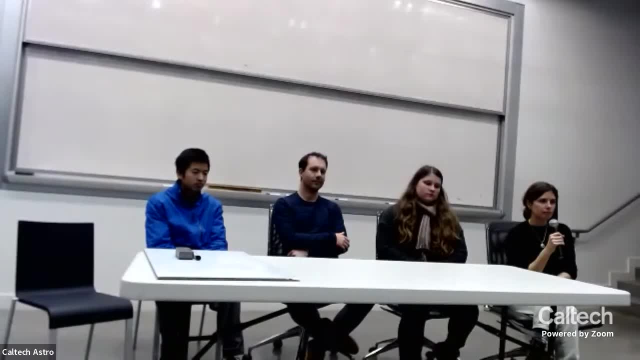 proxima centauri b, which is like four light years away. we've been putting out radio and television signals from the earth for 80 years, more than that radio for 100 years at least. so could those theoretically be picked up at that distance, would they be so? 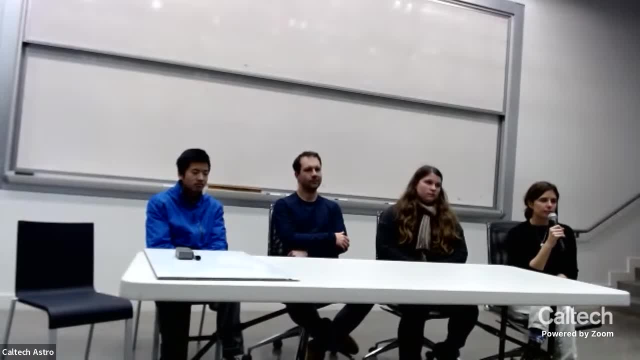 attenuated, that they wouldn't be intelligible, or like what. could that be a way? i mean, obviously there's a limited number of exoplanets we know of within like a hundred light year range, but is that, could that theoretically be a way that his question is somebody on one of those planets? 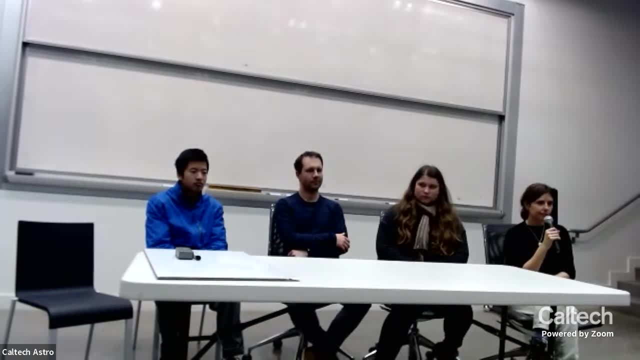 could detect that there's something, not something that's not a natural. you know transmission, sure i? i think it's important to um distinguish between the types of life that people are looking for. so most of the people that i work with um, or you know the kind of stuff that i'm doing. 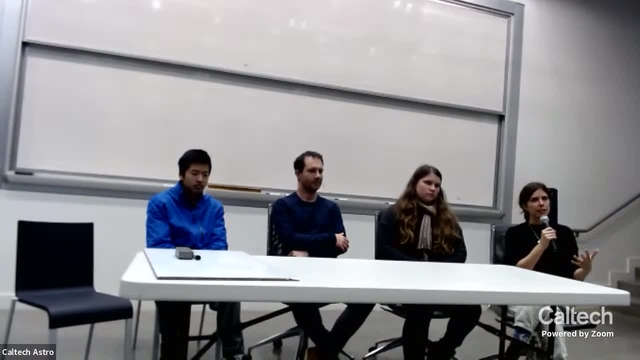 i guess the kind of life that we're really expecting to find is not in the intelligent life that you're talking about. so for most of earth history there's been no, none of that kind of life, not like technology, as you would call it, like most of it's just been bacteria dominated by 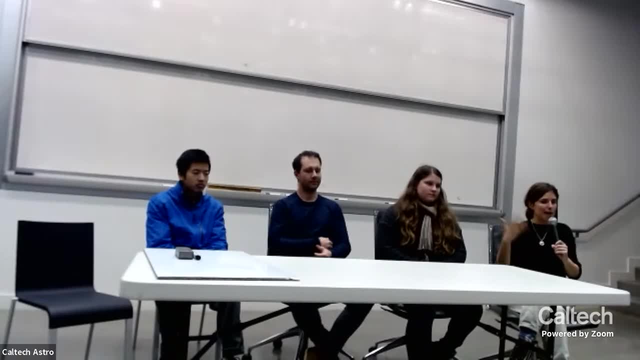 bacteria, and so the chances are if you see a habitable, if you see a habitable life- that's not just look at a random time- if you look at a habitable planet, we think that that we don't know how long human civilization is going to last, but we do know that bacteria have lasted for. 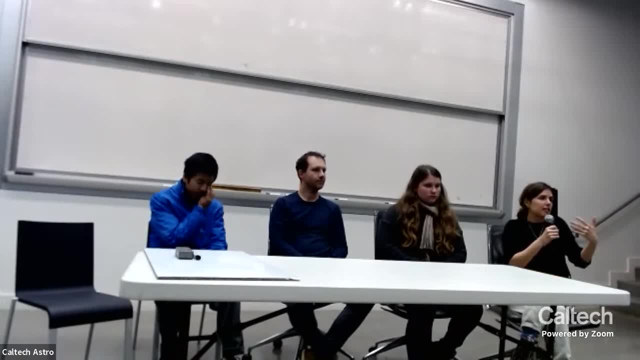 billions of years. so that's why you know we're hedging up me and you know people who are focusing on their atmospheres, hedging our bets. that that's the most likely way we'll find it. i think it's really exciting question, though, um techno signatures, because honestly, personally i 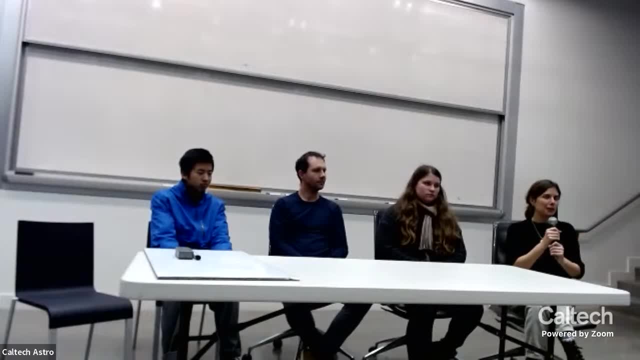 um, you know, i don't know how- it's very difficult for humans to travel between the stars, but it's, i think, a lot easier. it will be a lot easier for robots to travel between the stars, and so signatures of like techno, future technologies, um, is a pretty interesting thing to think about. 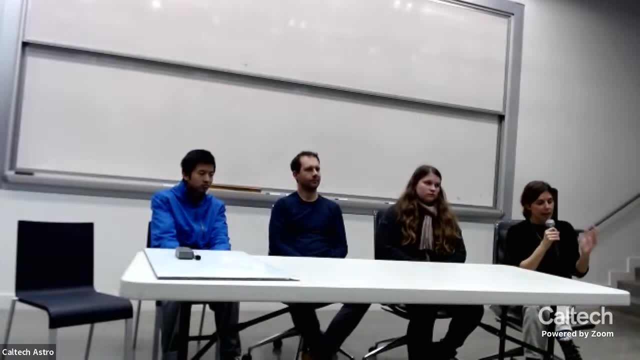 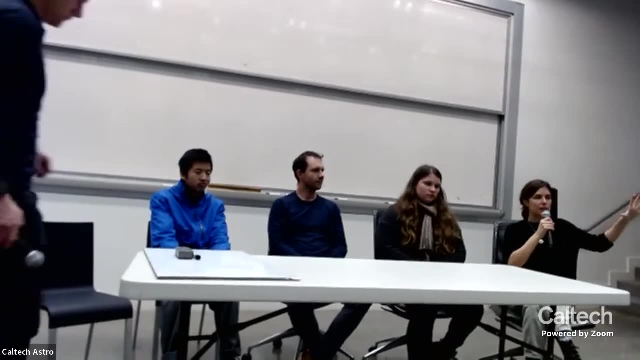 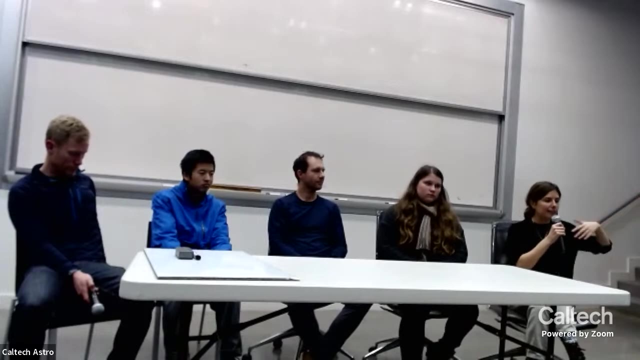 and very uncertain. you did hit on a good point, though, in the radio waves or any kind of um light or electromagnetic signal that you just beacon out in random directions from, uh a planet um. the further you go away, um, the weaker the signal gets. you can like focus lasers at like specific points in the sky, and so some people 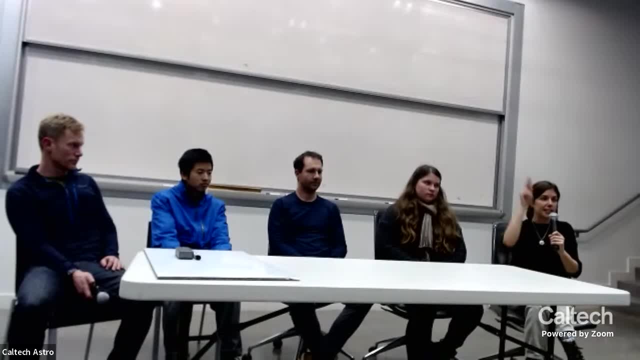 think about um civilizations who specifically target all of the stars in their neighborhood with like lasers, in that kind of that kind of stuff. there's also other like weird ways that people think um civilization might leave their marks by putting weird things in weird orbits um around stars. that would make 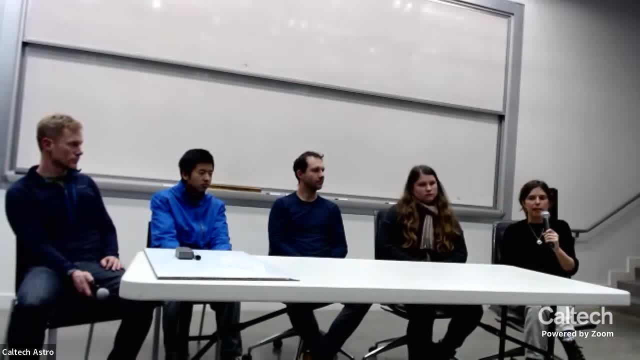 um, very clear signals of life, um, but yeah, i i am not 100 sure how um easy it will be to or how. i think it's very difficult to estimate the likelihood of finding a technology like that when the main thing we don't know is how long technological civilizations 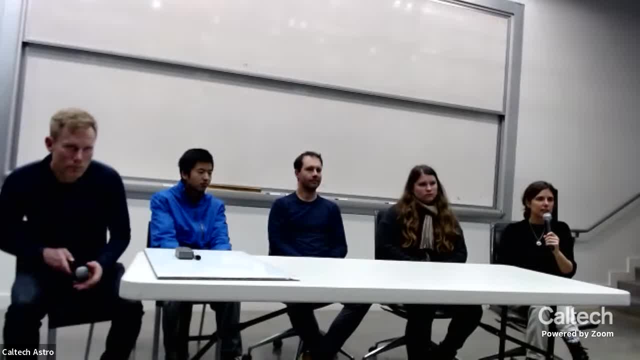 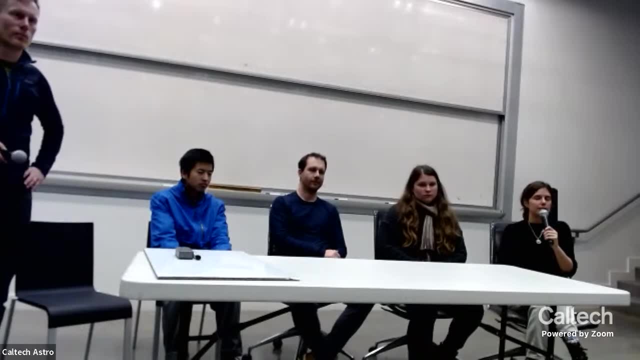 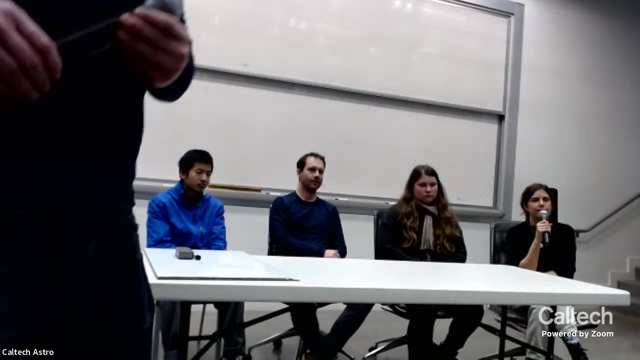 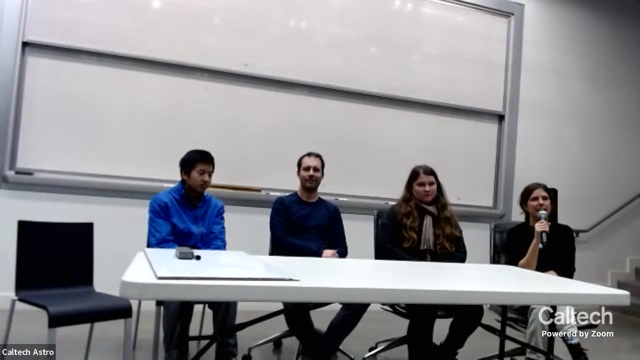 last, i think. right, right, i think i don't know the answer to that, sorry, yeah, i'm not. yeah, i, it's a good question. i don't know the answer, sorry, well, i, they sound like intelligence with great taste. uh, i don't know, hi, um, so i know that the atmosphere is very important for fostering the emergence of life. 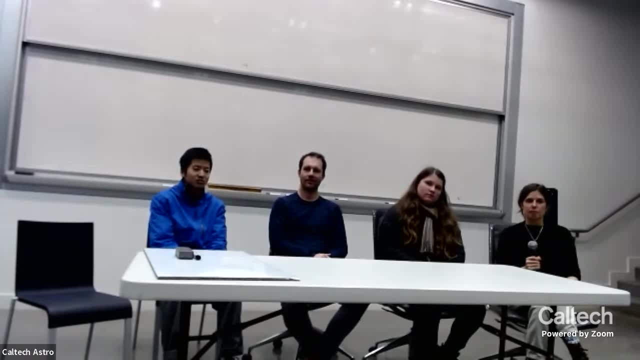 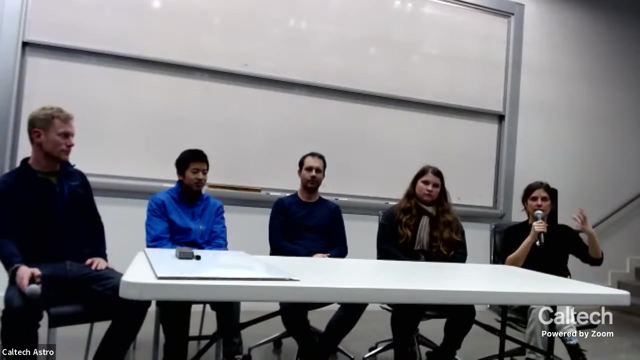 so on another planet, even if there wasn't an atmosphere, would a body of water? would that serve a similar purpose of an atmosphere for fostering life? yeah, it's a great question. so in the solar system we have a couple of moons of the giant planets further out that have massive oceans of water under a surface of solid ice. people are really 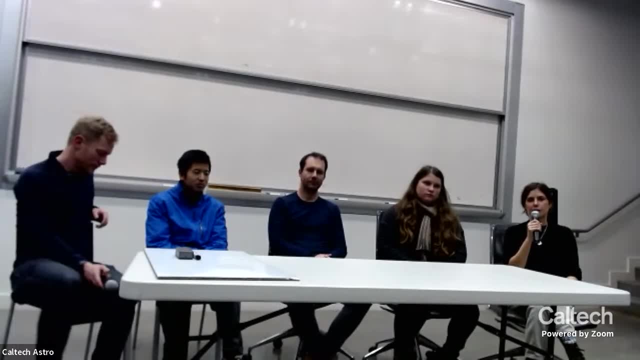 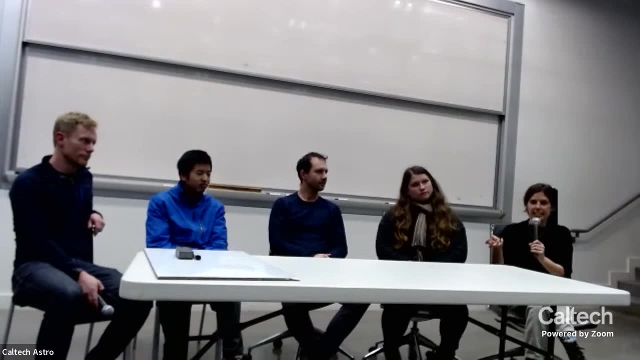 excited about the chance of finding life in those oceans. they have like a heat source as well. those, the cores of these planet- not planets, moons- are like, heated by, like tidal gravity as they go around the planet, so that and that's what melts the planet, and that's what melts the planet, and 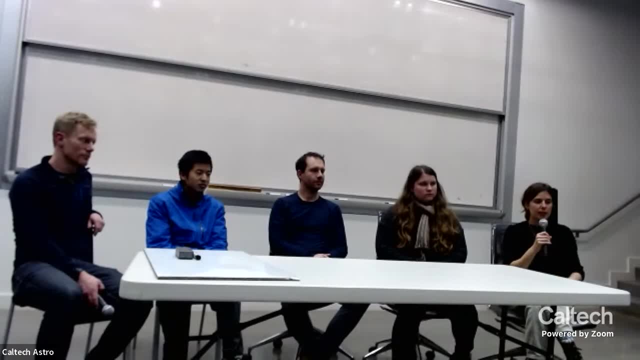 that's what melts these water, this water ocean, and keeps it liquid. and there are, we think, the ingredients of life in these um oceans and we are sending probes to try and like look at the escaping plumes from these um. so yeah, i think there are. there are a lot of people who think 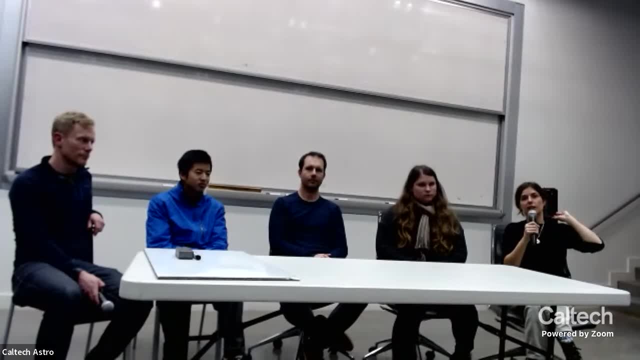 you can form life in these oceans even if you don't have an atmosphere. um, yeah, i think you still need like a special set of a special environment because you you still need to, maybe protected by the um, solar wind and radiation somehow, and still have a heat source. 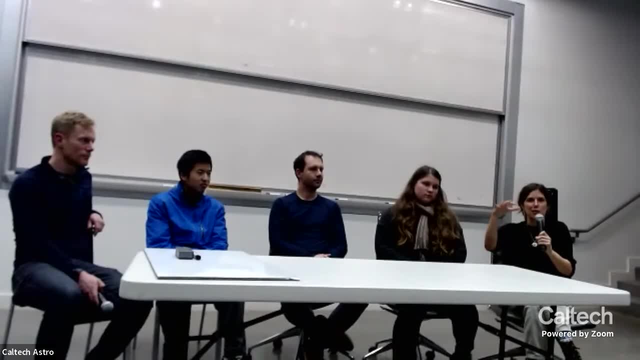 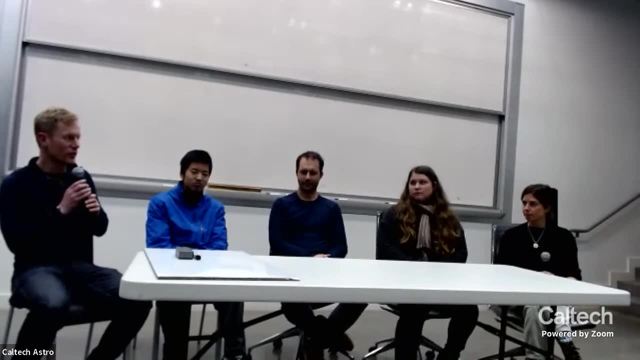 from somewhere to keep it liquid if you don't have the atmosphere protecting it. yeah, related to that, there was a question online about the presence of oceans on exoplanets, and would it be possible? uh, so, roger, i asks this and he he asked if i can paraphrase: um, you know, we 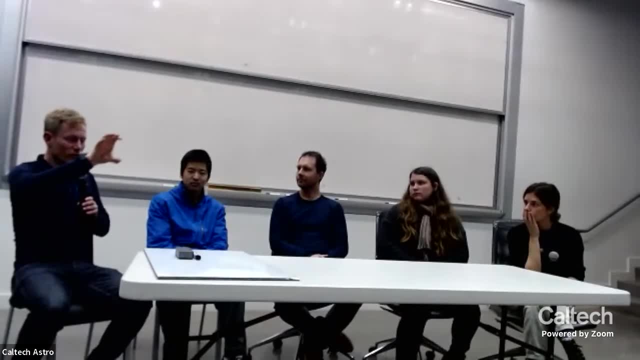 we can figure out how to protect the atmosphere from the exoplanets and we can figure out how to figure out the wobble of a star and figure out that there's a planet orbiting around it, causing the star to wobble wobble. can we also figure out something about the distribution of stuff on the 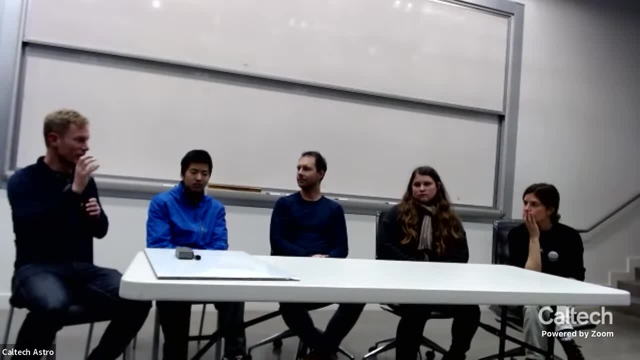 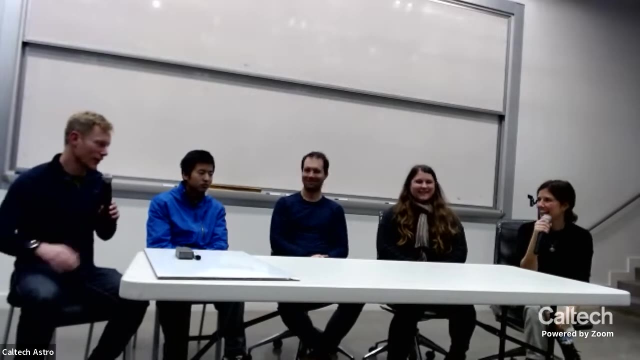 surface of a planet, like sloshing oceans or something like that. that would wobble the planet that might show up in the wobble, or is that is? is that too far from like our detection limits and what our instruments can pick out? um, yeah, i sorry, i feel like you're the exoplanet. 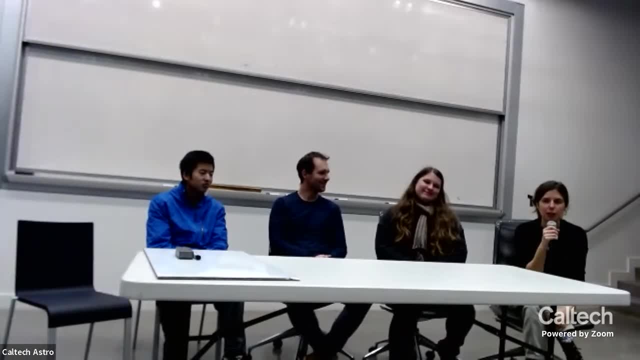 so right now we are approaching the level where we could detect the wobble of earth-like planets around sun-like stars. when we're like getting, there's a ton of experts in california who are working on this. um, so that's to do the wobble of the sun caused by the planet i actually have never. 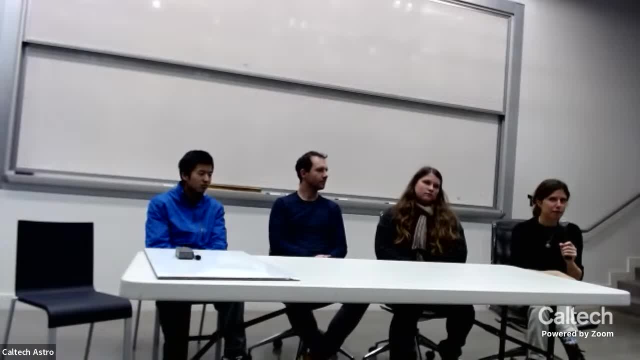 thought about the sloshing around of um liquids on a planet to see the wobble of the planet itself. that's a really good question actually. i think seems like there'd be a tidal effect from it. yeah, i distributing mass, yeah, but so right now, you know, we have maybe like 10 or 12 systems. 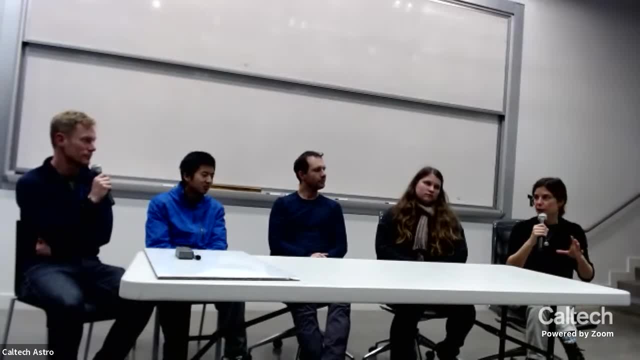 where we've detected direct light from the exoplanet itself. so i imagine that you probably want- it would probably want to be a direct detection of the light from the planet, and then you get that um wobble, so i think, and all of those plants we found are like massive gas giants, so they don't have 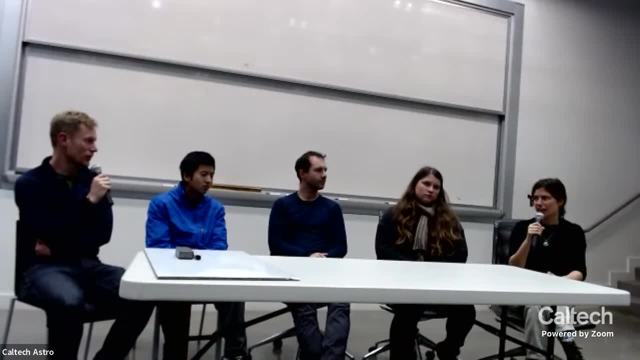 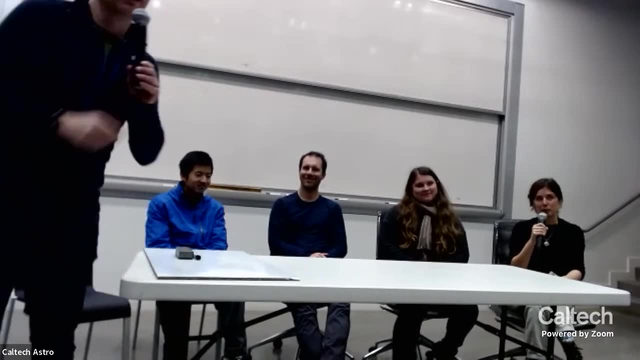 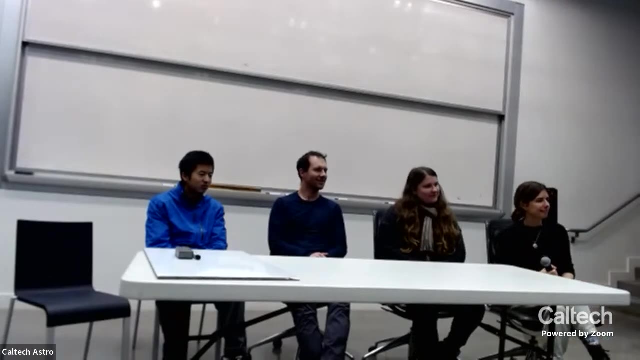 you know solid surfaces, but that's a really cool idea. i like it. yeah, well, we'll. we'll cite you. yeah, i will credit you on my next paper about that topic. there's a question from our young audience member here. uh, so how do atmospheres affect planets? 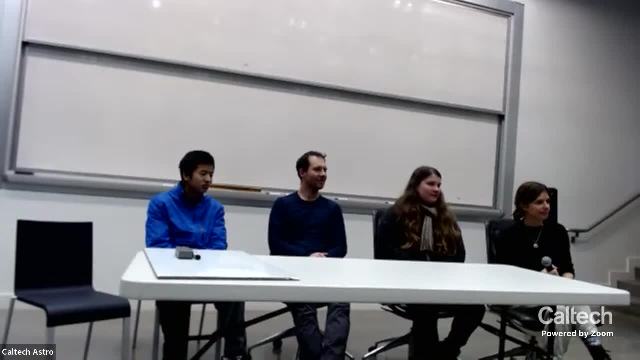 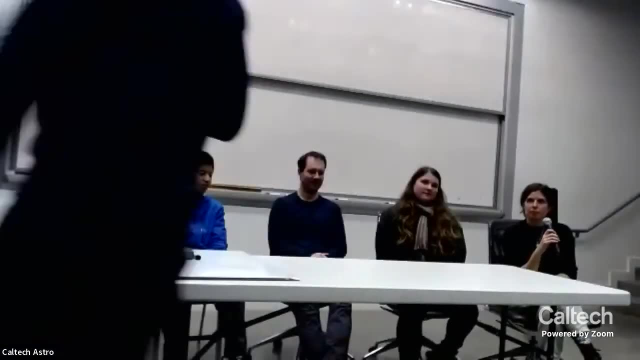 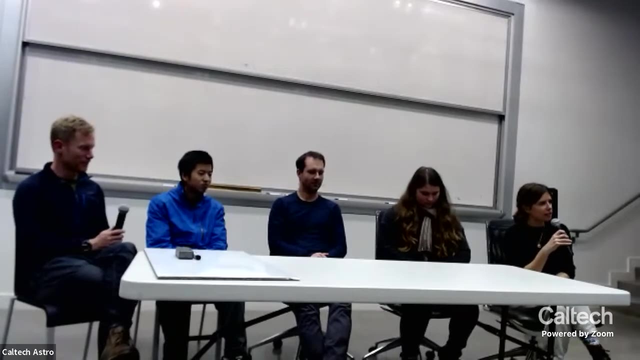 yeah, okay, how do the atmospheres affect planets? do they change the dynamics of the planet? do they change surface properties of the planet? yeah, and you like the earth's uh surface has been like weathered by, uh, the earth's atmosphere. um, you know, when you go and look at some like cool rock formations, the 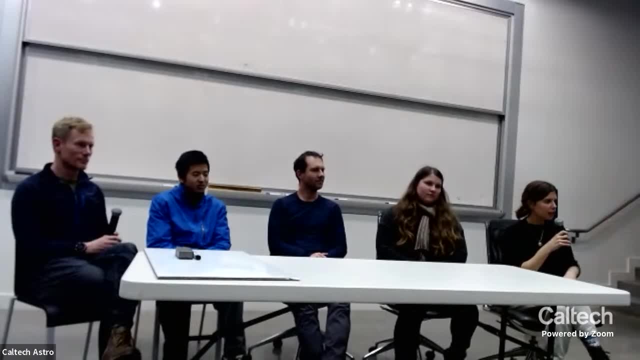 wind is like blowing through them and kind of change the shape of the rocks. um sand dunes- yeah, sand dunes, and actually so, uh, in the solar system there are some kind of sand dunes on. this moon called titan has a very thick atmosphere. it's the thickest um atmosphere of any moon in the 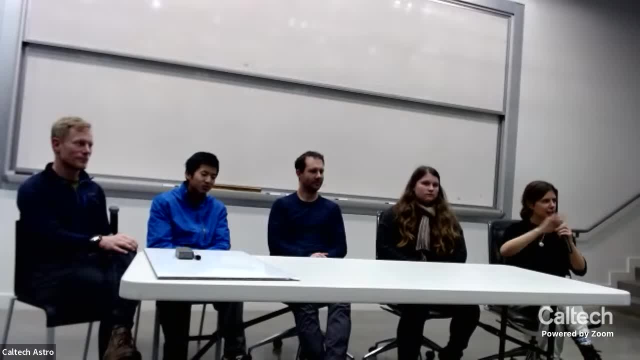 solar system and you can see these dunes sound like sand dunes of like water, ice, and like there's winds that whip around and like we're learning about those winds from looking at the shape of those dunes. and so yeah, the atmospheres can affect the shape of those dunes and so yeah, the atmosphere. 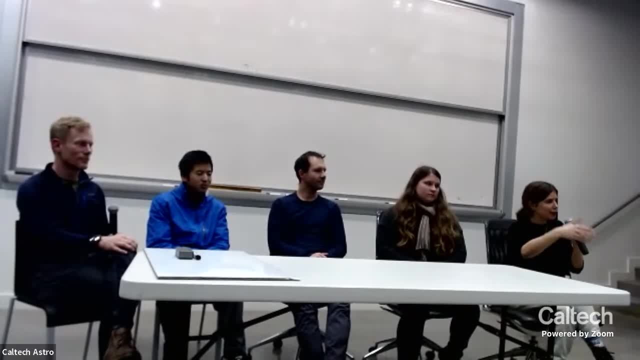 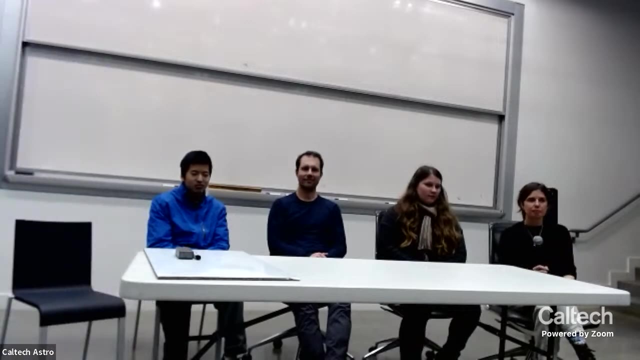 can affect the surface and by looking at the how it the surface is affected, we can learn more about these atmospheres. um so yeah, great idea. i like it. just a question from a new audience member. i was wondering if there are any current methods to gauge the isotopic composition. 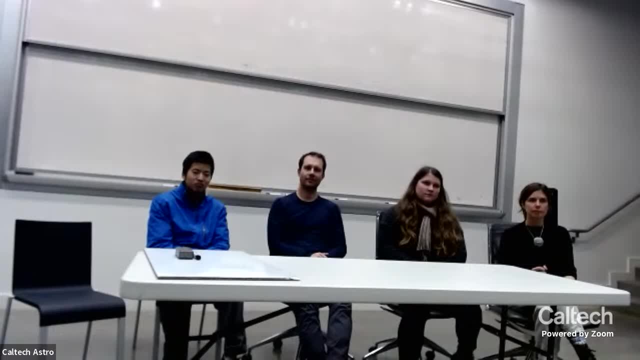 of an exoplanet's atmosphere and if we could detect any isotopic fractionation from that. did you get that? yeah, yeah, so if there's any way to look at the isotopic ratios of things in a planet's atmosphere, so, uh, an isotope. so when i showed that picture, 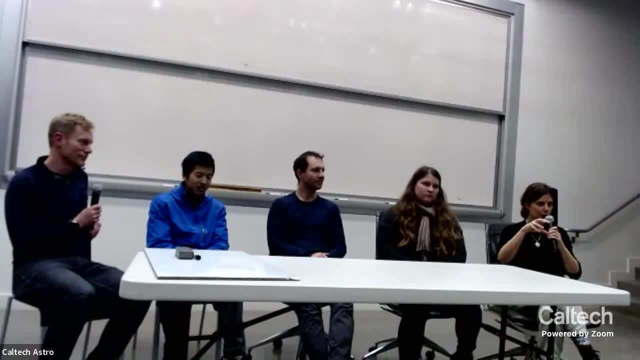 are of a atom. you got the nucleus in the middle and a bunch of electrons on the outside. so we had these examples here and washed it out and we found that. so yeah, we, we had these examples of the black holes and black pipery and stuff. so, um, i had to give it back. but very 이후, but i saw one. 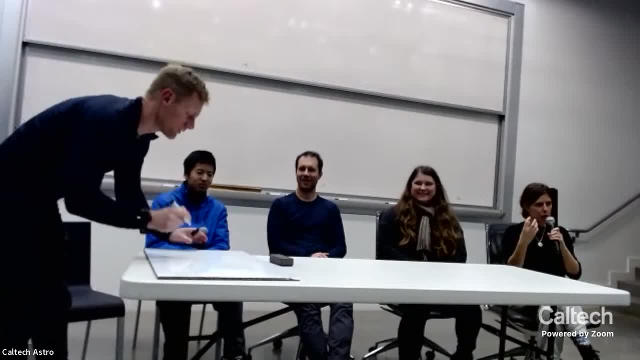 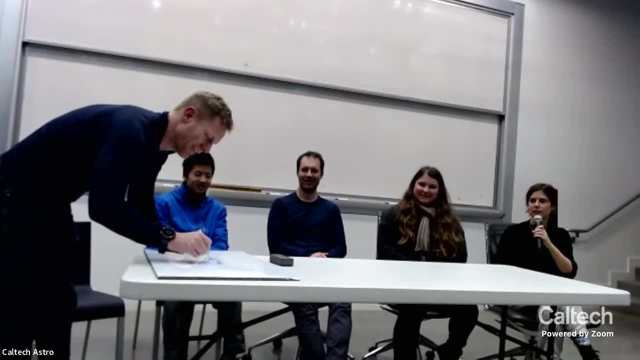 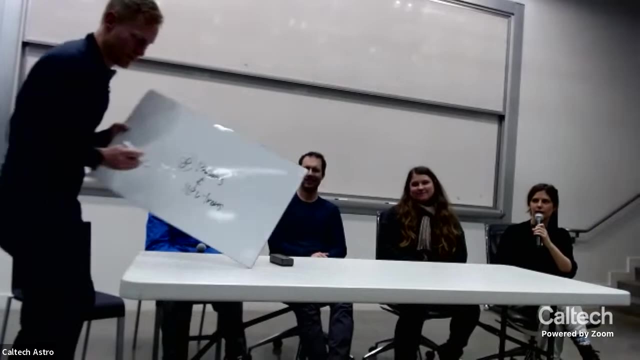 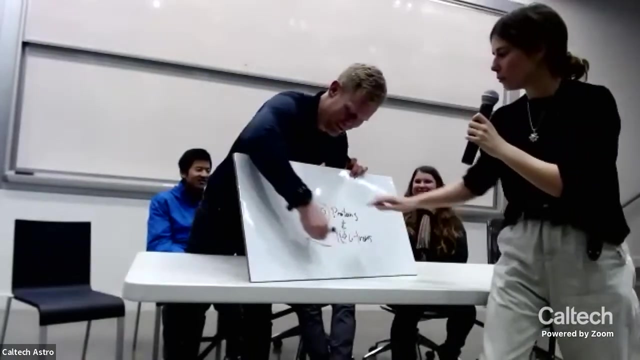 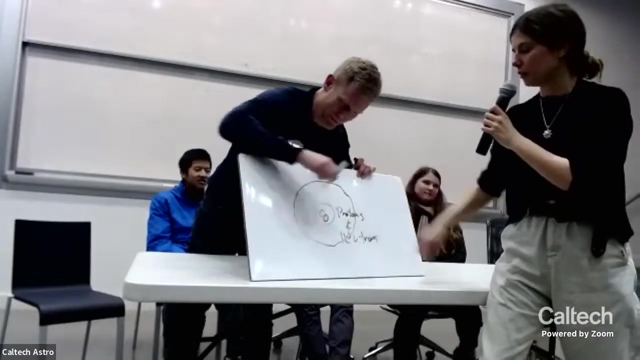 inside the nucleus. you have protons and you have, oh, the whiteboard. yeah, we've got protons and neutrons, yep, all right. so, yeah, great, can i just like cool, right, can we do like, can we do like deuterium and hydrogen, so we just get rid of one of those, right? so this is one way you can make hydrogen, and then this is: 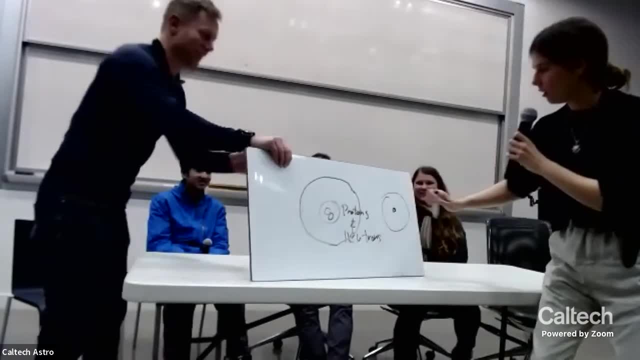 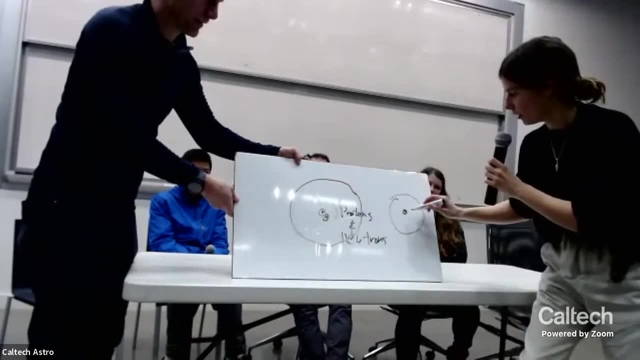 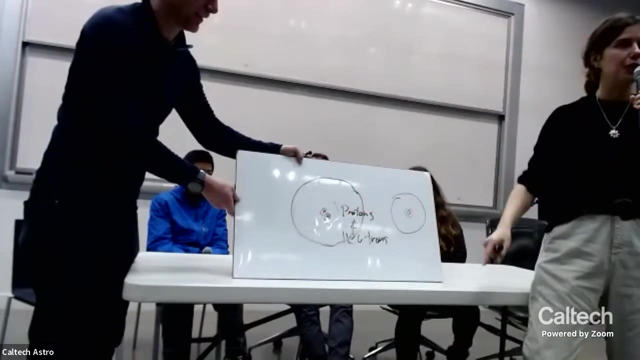 another. we'll just actually sorry, i'll do that as well. so we've got p here and an n and we got just a p. so in the, in the nucleus, you can have these protons. these have a positive charge and these are like the really important ones for telling you. 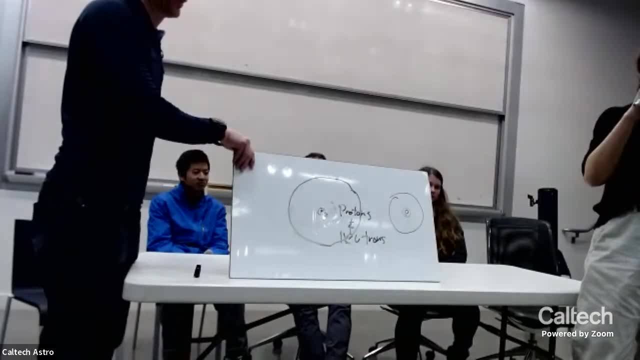 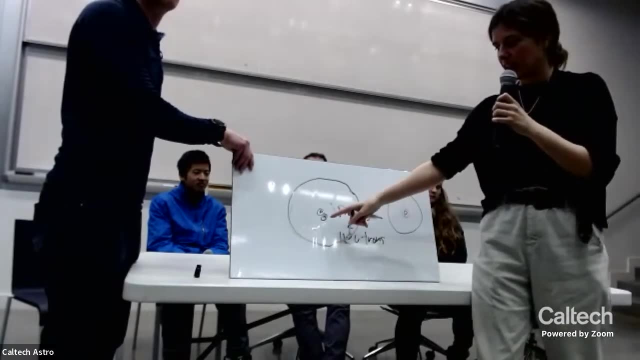 you can make hydrogen, so we just get rid of one of those, right. so this is one way you can make what this atom is. so hydrogen atom always has one proton, but there are these other things called neutrons, so they have no charge, but they have mass and they can hang around in the nucleus. 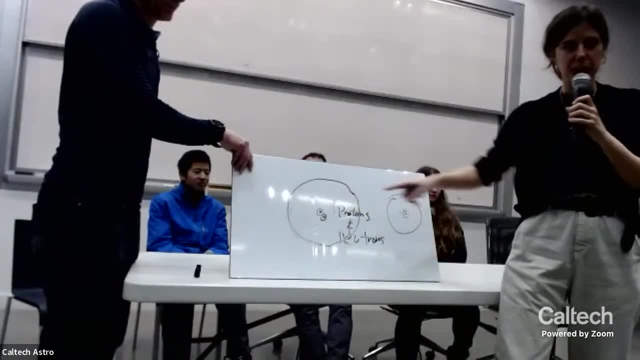 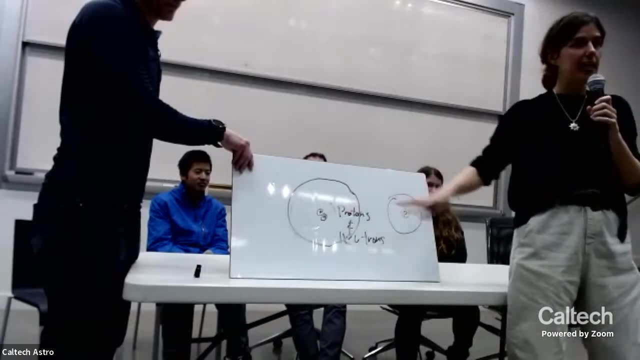 it's still hydrogen, still have one proton, but this one has, uh, one neutron and this one doesn't. so this is heavier than this thing, even though it's still hydrogen. and this means this hydrogen, like chemically, is the same, has the same kind of reactions, but like if you have like a 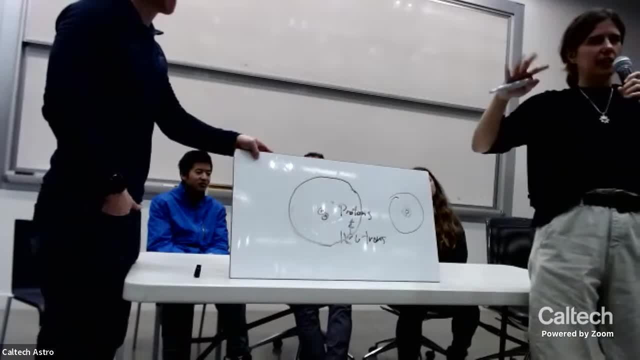 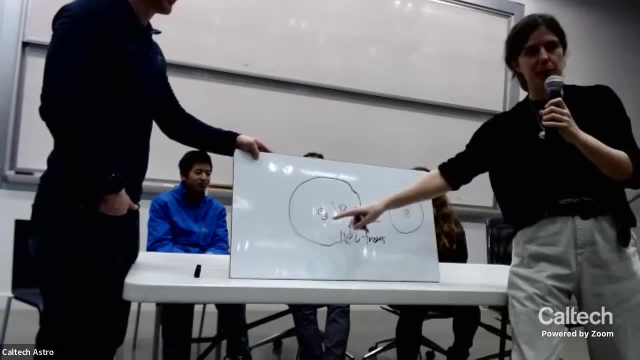 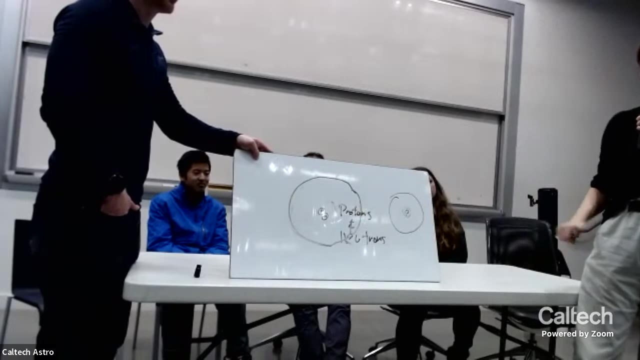 bunch of hydrogen in a bottle at the right sort of temperature. maybe some of the heavier ones might like sink to the bottom because they have this extra neutron. so so these are isotopes, the a different isotope has a different number of neutrons in the nucleus, so this is really cool. 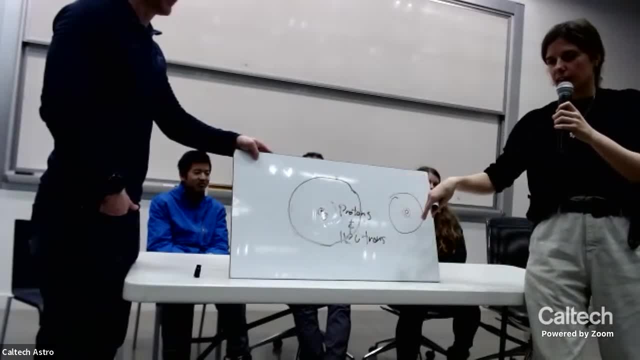 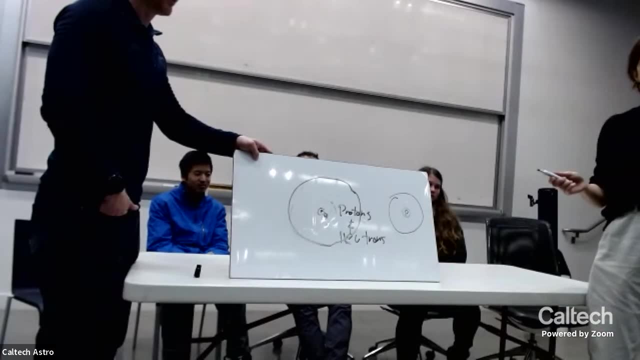 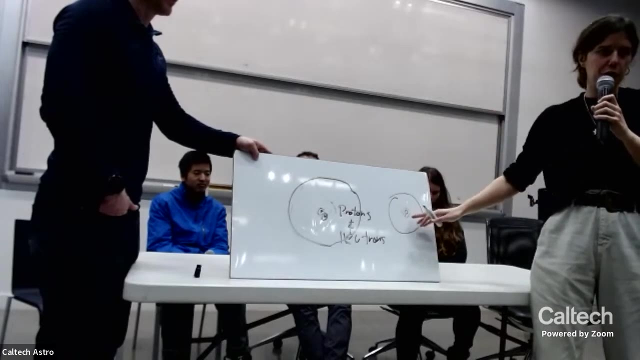 because, like the, these uh isotopes are affected by like a bunch of different processes in different ways, so you can learn things about like: oh yeah, how much hydrogen did it start with? and how much of this light hydrogen with no neutral, with no neutron, got like sifted off into space. because this is because it's lighter, it's probably easier. 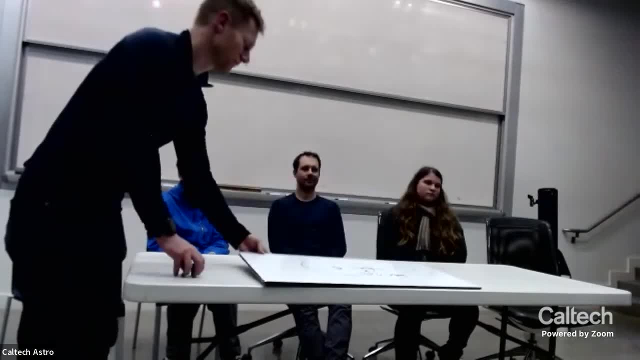 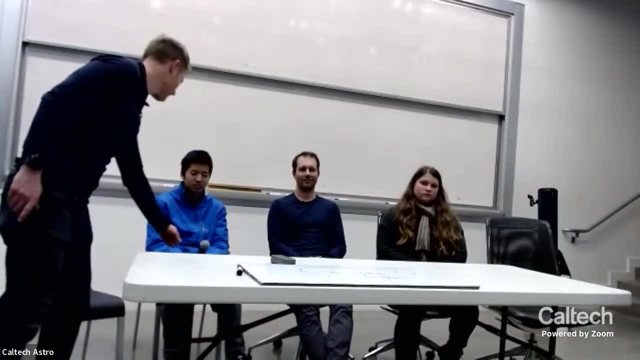 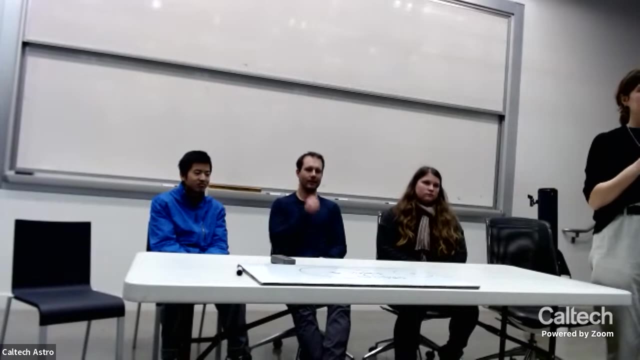 to lose. so, yeah, this is, this is what an isotope is, is why we're interested in them for planetary science, especially atmospheres. and the answer to your question is: we are trying to do this, but it's very hard. um, but yeah, uh, the uh, the signals of different isotopes, the different um effects. they 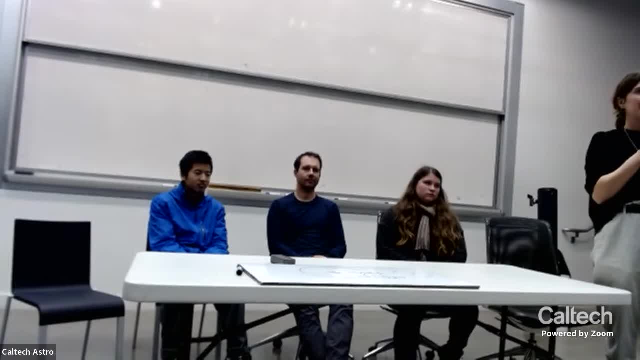 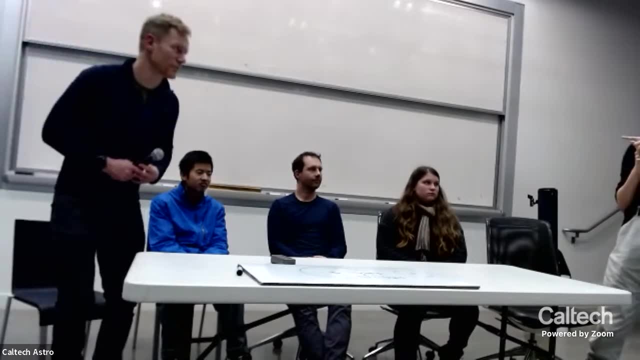 have are like really small, smaller than the precision that we have our telescopes right now. it's really cool. i think in the future, when we have bigger telescopes, um, we might be able to see. i think some people are maybe trying to do it with jwst because like there are some like carbon. 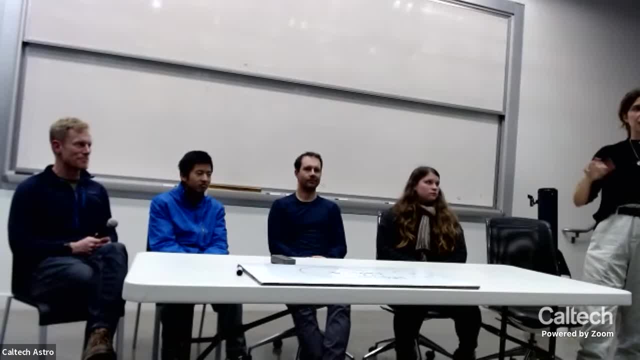 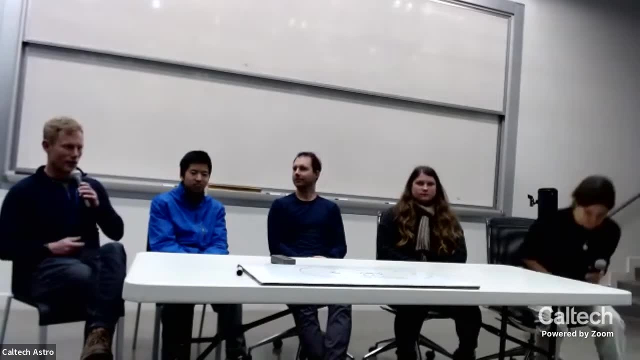 bearing species that look kind of slightly, with different isotopes that look kind of slightly different. no one's done it yet, but people are trying. so, yeah, cool. um, there was a. there was a question online. uh, i don't know if you have any questions, but i think it's really cool to have. 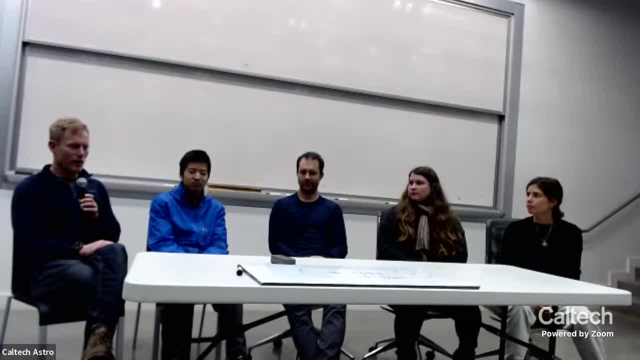 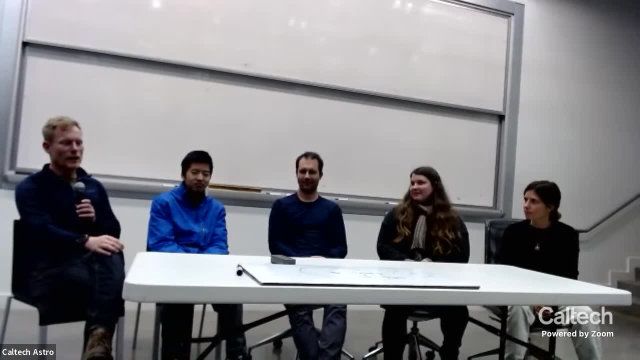 uh from one of the online audience members about uh, a recent paper that came out that's been all over the news, at least all over the science news, and if we had any opinions about this paper. so the paper is a very controversial paper, suggesting that there's a relationship between black holes. 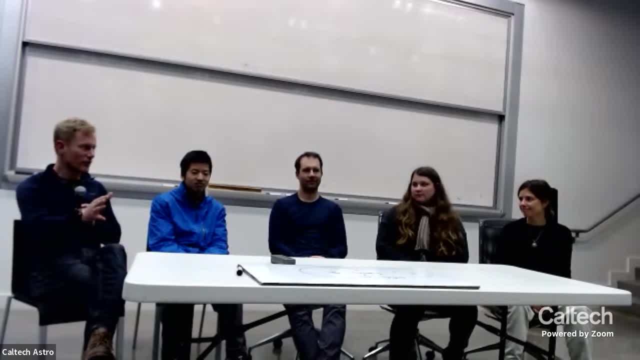 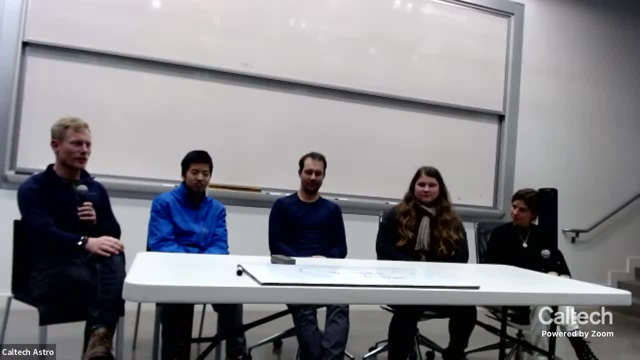 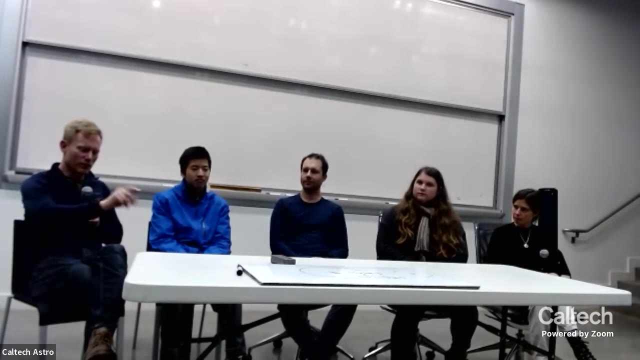 energy, which is another thing that we don't really understand. in fact, we understand, i think, a lot less about dark energy than we do about black holes. dark energy, as i alluded to before in the question, in addressing, uh, the one that you'd asked, is this kind of strange thing that we- we we- describe as 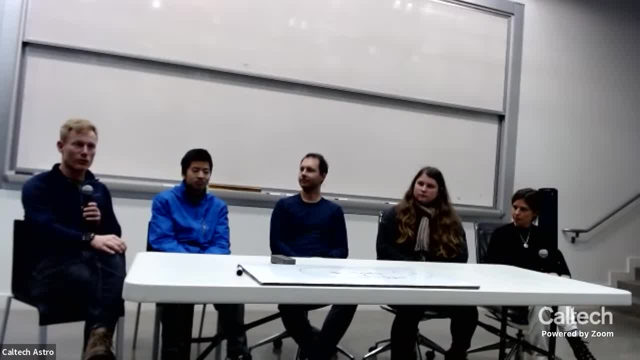 being responsible for the acceleration of the expansion of the universe. so the universe is getting bigger over time, it's expanding outward and dark energy appears to be accelerating that rate over which it's expanding. and, uh, the so. did you guys read this paper? no, oh, so i'm, i'm here, i'm. 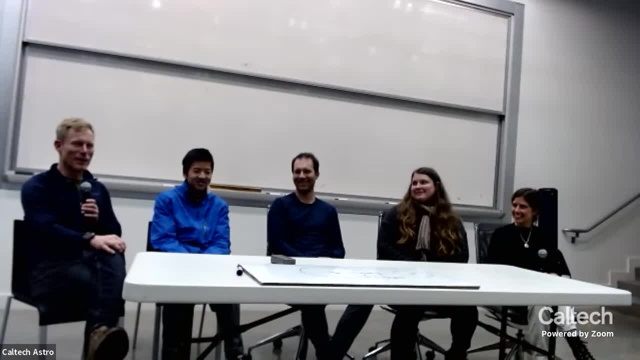 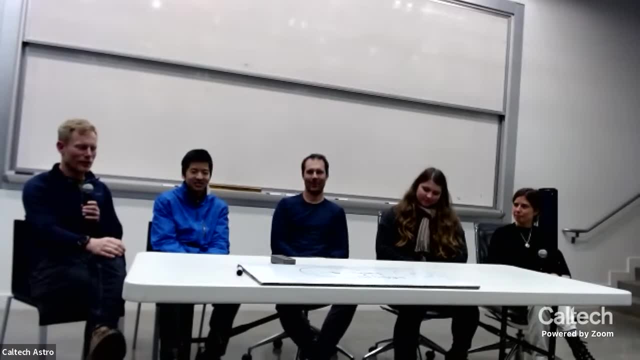 stuck by myself, not having read the paper very in depth. well, i'm not an expert on this topic, but i will try and posit what what was written in the paper. so the idea is that there's a relationship between these two things and, uh, what's described in the paper is that there's a relationship. 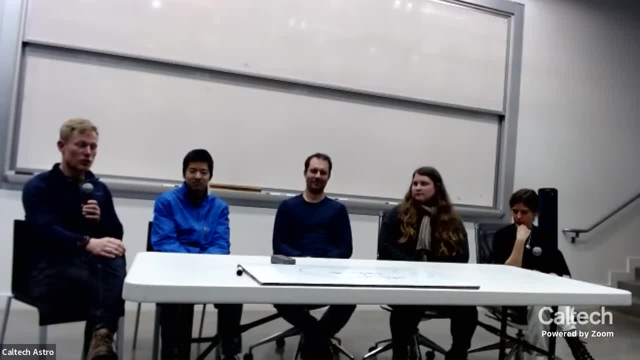 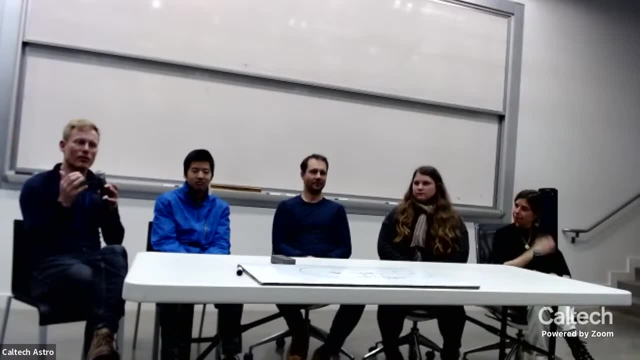 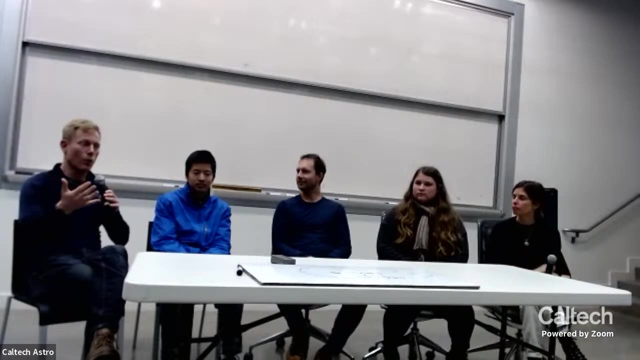 between the mass of a black hole, of a supermassive black hole in the center of a galaxy. we think that most galaxies contain a supermassive black hole in their centers. it's difficult to get constraints on the properties, even the mass of that black hole, because because they're black holes, they're 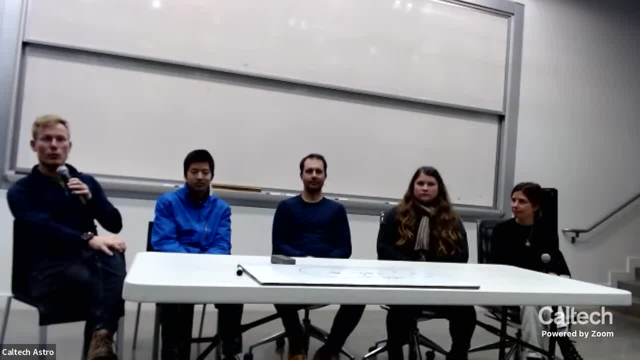 dark and they're hard to find. i mean, oh, peter, did you read this paper? you did. do you want to get up and help me with this, or no? oh, you'll probably do better than me. uh well, shout out if i'm wrong on any of the things that i state. 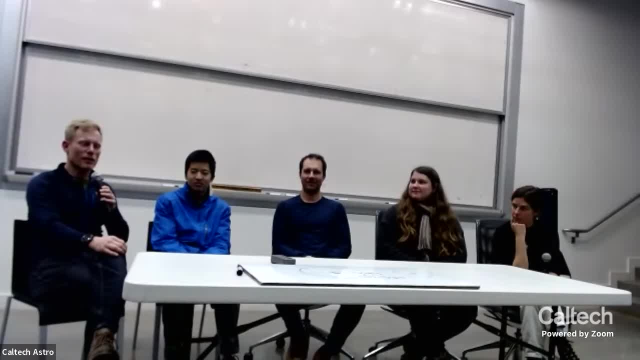 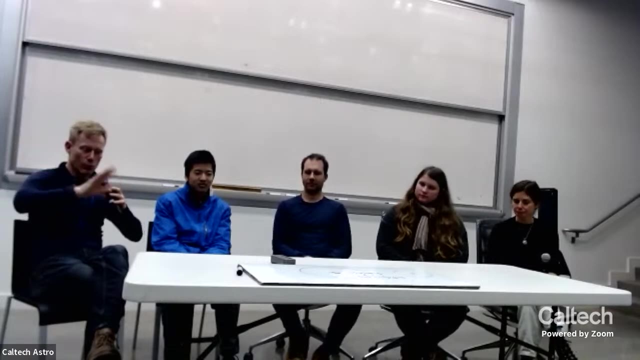 here. um, so basically, uh the authors, based on previous evidence, there seems to be some relationship between the mass of a black hole and the mass of the galaxy that contains it, and what people have previously found is that between redshift of two, which is some distance away from us, and some time in the past, and the present day, uh, the, the, the black holes. 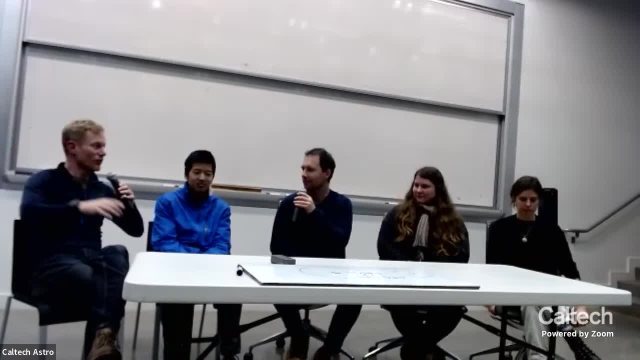 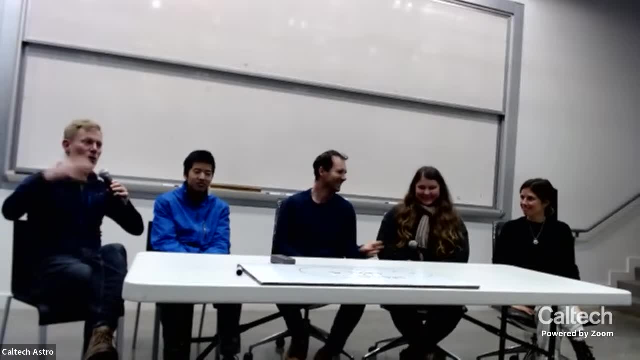 appear to be getting bigger and more massive relative to the size of the galaxy. 10 billion years- 10 billion years, thank you. 10 billion years ago to present, the black holes appear to be getting larger relative to the size of the galaxies, statistically speaking. we aren't watching a. 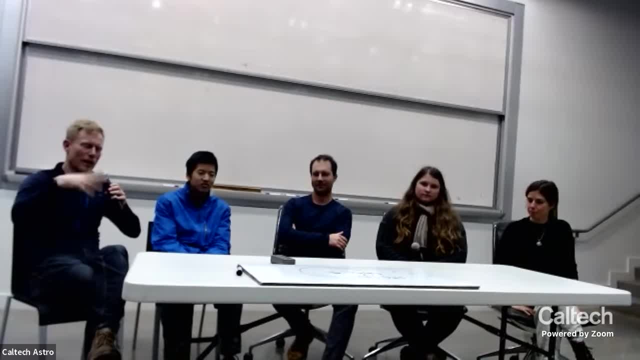 single galaxy change over that period and watching the galaxy or the black hole get bigger. we're just seeing that this. there's this relationship between the mass of a black hole and the mass of a galaxy relationship, but even that is contested, that that whole relationship, because it's really hard to do. 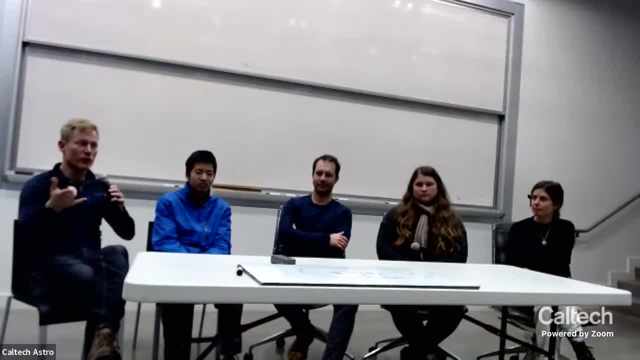 this and it's not clear. some some authors will describe the reverse thing, that galaxies are shrinking relative to the size of these black holes, um, so that already calls this a little bit into question, but the argument that, as far as i can tell, is being made by the authors is that, um, 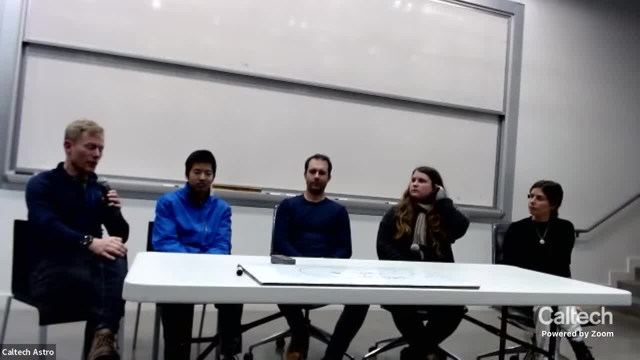 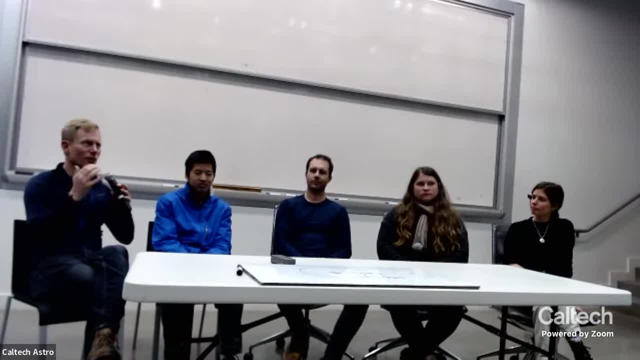 energy, the quantum rest energy, and and that somehow, as the universe expands and accelerates in its expansion, it's causing those balls of energy to grow, and thus the supermassive black holes appear to grow relative to the size of the galaxy, and so that's a huge ball of energy, that's. 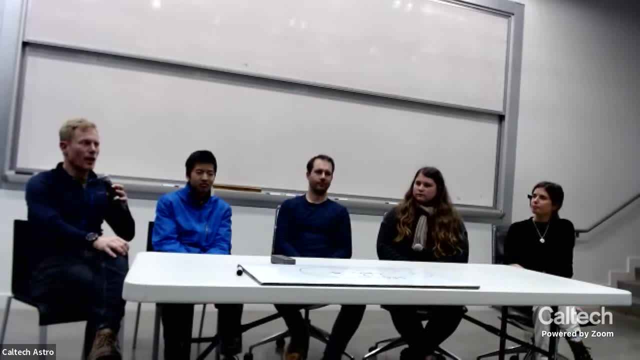 the size of the galaxy. but, as i hopefully demonstrate, i don't fully understand uh this, this, uh this argument and in talking with other colleagues in in the department there it's, who are more expert on this, it seems like there's a lot of. it seems like we don't have enough um. 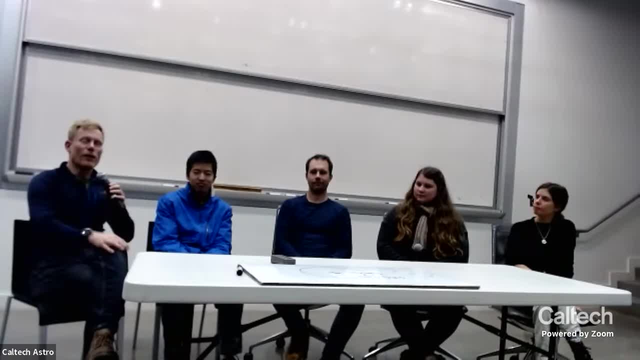 let's see what's a good analogy if, if i go outside- this is maybe this isn't the greatest analogy- but if i go outside and I see a flashing light in the distance, What is that flashing light? Probably one could say, oh, it's an airplane, Oh, it's somebody with a flashlight shining it all over the place, Oh, 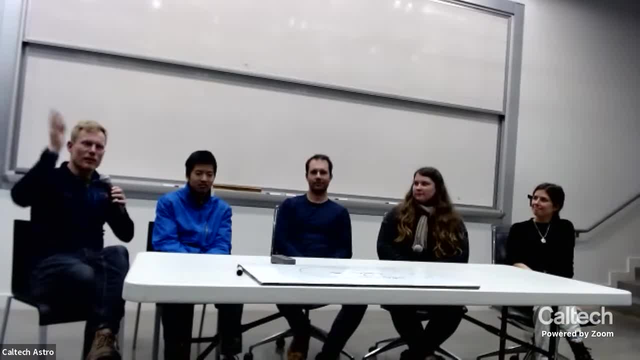 it's, you know, a bird with a flashlight attached. There are a variety of different suggestions for what, what that could be, rationalizations for what that could be. I could be hallucinating in the desert, but if you immediately go and say that's an alien, 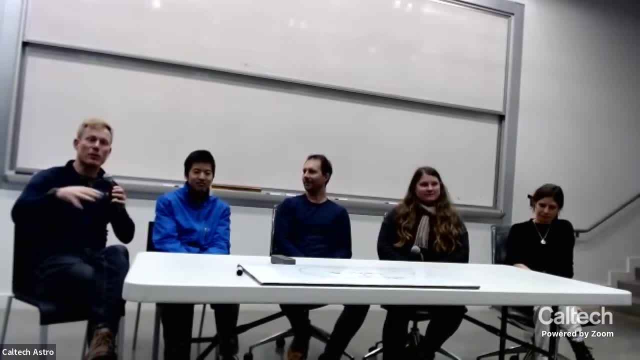 that it seems like there are much more likely explanations for the observation that you've made than to invoke some sort of kind of exotic and wild explanation for that thing. And in this case as well, it seems like there are more mundane, more, uh, more kind of probable explanations for 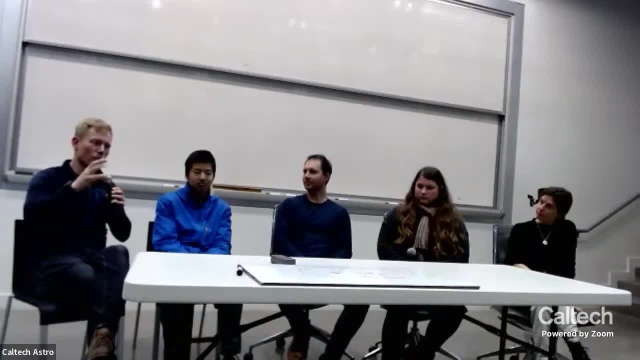 the observation of do supermassive black holes grow at a different rate than their galaxies over the evolution, That you don't have to create some sort of wild explanation. And the only reason you would start to create wild explanations is is if you've ruled out all of those kind of easy to explain things. 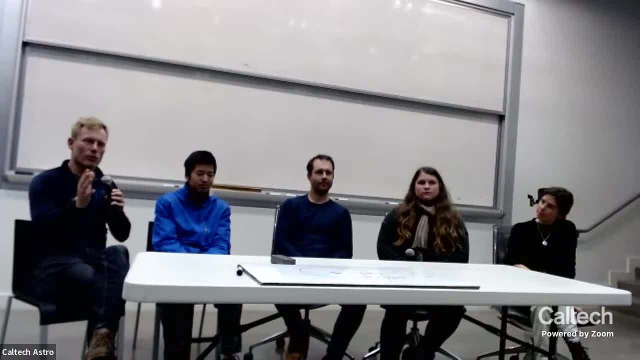 that don't break our model of cosmology or or cause craziness. So that seemed to be the general conclusion of the people with whom I spoke about this is that you don't have to invoke something quite so exotic to explain In this relationship. Peter, is that roughly consistent with your take on it? Okay, Since he's. 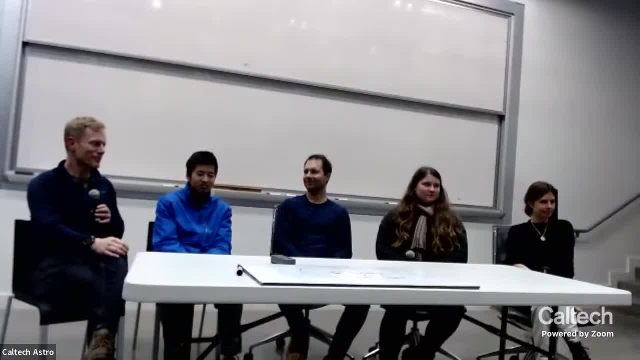 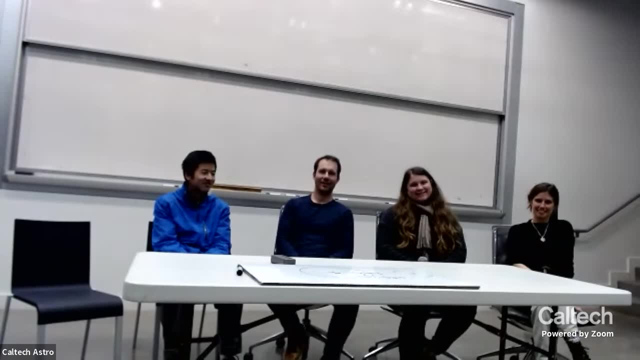 more of a black hole expert than me in the audience. Thank you, Peter. Okay, Sorry for that side topic. I wanted to break from the straight exoplanet atmospheres question. Uh, you have a question. Um, back to exoplanets, Uh, um. so you talked about stellar flares and the possibility. 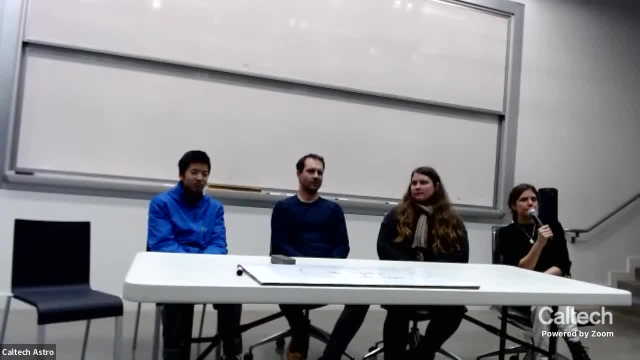 of stripping atmospheric elements from the planet. My understanding is that there's a school of thought that says that, that posits that maybe, like radiation in the form of stuff getting to be from a star or other other other sources, um could be actually be essential to the formation of life. 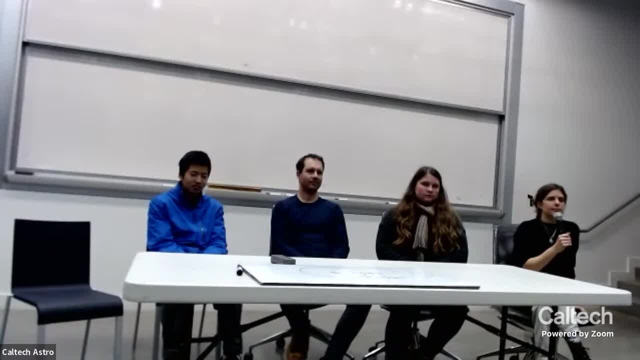 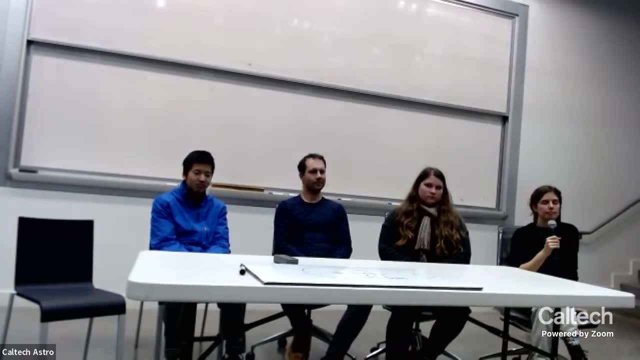 Like it, like an X, like a galvanic, you know, kickstarts a process, So a process by which life forms. So do you have any thoughts on that? And you know where do you come down in that school of, with that school of thought. 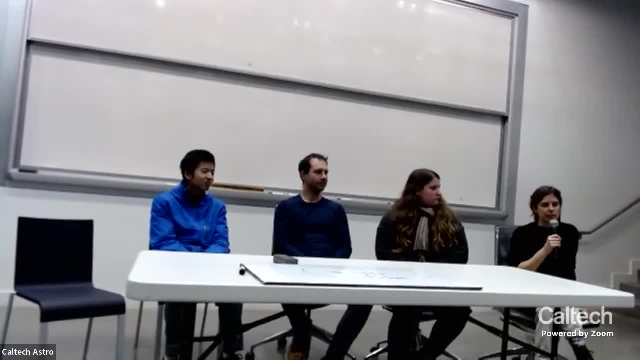 Um. so the study that I showed, where they like search tests with like a like a bunch of flares, um, and they found like the M-Dwarfs have like loads and loads of flares. They did specifically look at these kinds of flares that people have suggested as like necessary for the um, like, 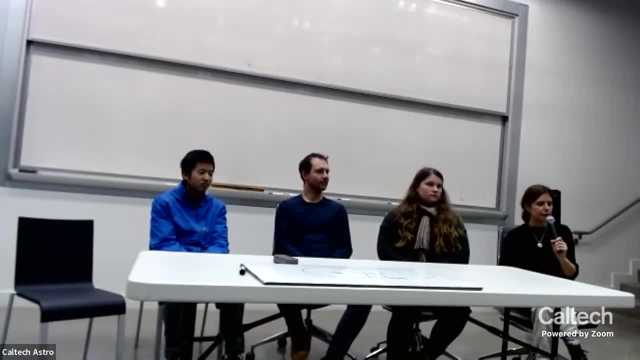 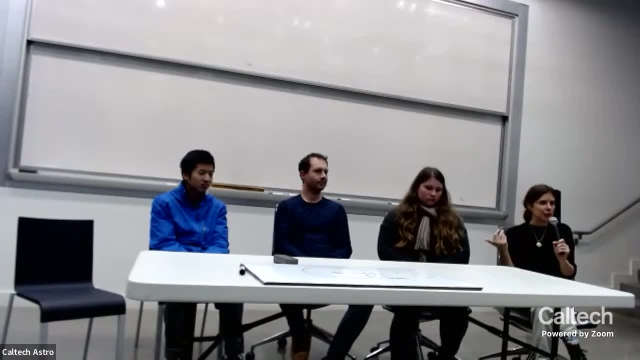 the, the bigger the flare you have, you know, the more dangerous it is to the actual atmosphere itself. So those are indeed more common for these smaller planets, but also so are the ones that, um, yeah, will just strip away the atmosphere. Um, I don't actually know too much more about it, but um, I don't think many people know. I think we still don't know if they can maintain any atmosphere, which I think is the question to start with, um, before we can answer that. But yeah, maybe, though if they can retain their atmospheres, then maybe they are more likely to. 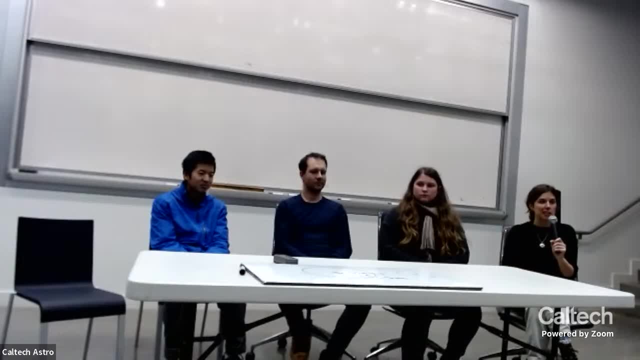 start kickstart life with these flares Definitely is a possibility. That would be sick. Yeah, That's a scientific term. yeah, I think it's a scientific term. Okay, Um, let's see. I have a a related question, um, about comets that might be appropriate for Qicheng. 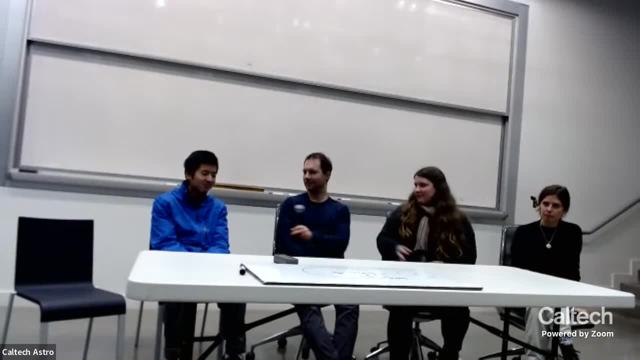 So Kieran Mehta asks back: in 1986, I participated in an international comet Halley watch That collated various observations by spacecraft, observatories and amateur astronomers from all around the world. Um are there. why haven't projects like this internet, this um? 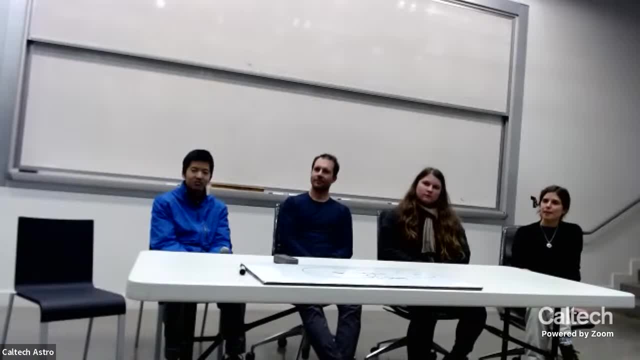 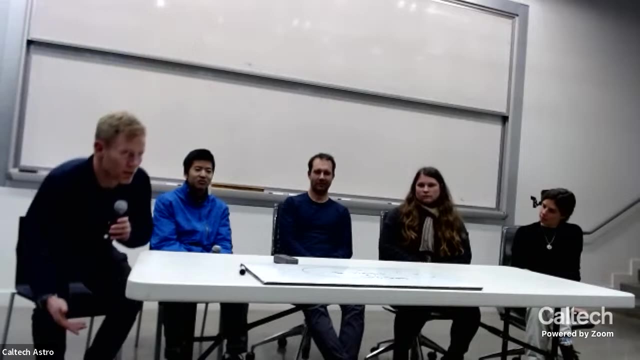 international Halley watch happened since, either for this comet or for other comets, And what is kind of just in general, can you speak to, since I know you're a comet observer? um, can you speak to like what? what are the ways in which we detect comets and then continue to? 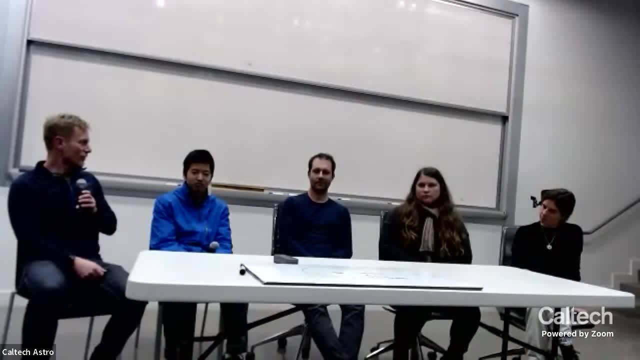 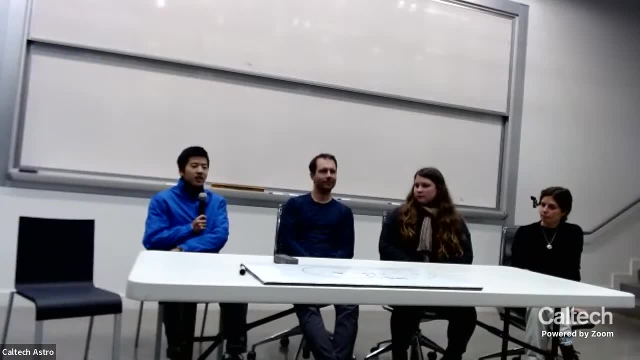 observe them to better understand their orbits and their trajectories and their implications in the inner solar system. Right, Sure, Yeah. So uh, it's actually been a quite a number of different uh comet observing campaigns since the 1980s. Uh, so of varying degrees of uh complexity and 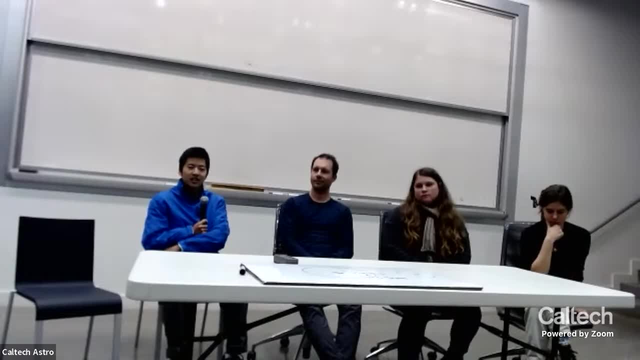 spacecraft and involvement in size. Uh. so in the last uh decade or so, we've had uh, the biggest one was probably the comet ISON campaign, which is back in 2012,- 2013.. This was a big uh. it's actually a not that big of a comet. 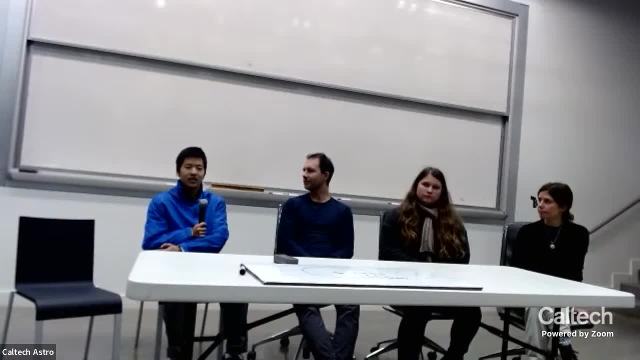 but a uh sun grazing comet that uh came from the Oort cloud and uh was uh destroyed by the sun in November, on Thanksgiving, actually Thanksgiving day of 2013.. And so th there was basically This comet that was found still out in the outer solar system about a year before it was to 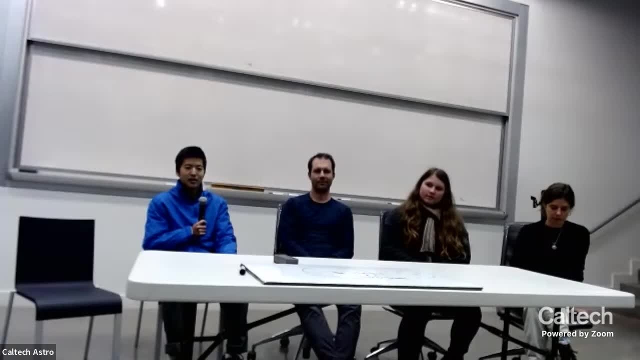 have this close approach to the sun And lots of people got super excited about it And because it's not very often that we get like an ice ball that's diving straight into the sun or almost straight into the sun, And so there was a huge 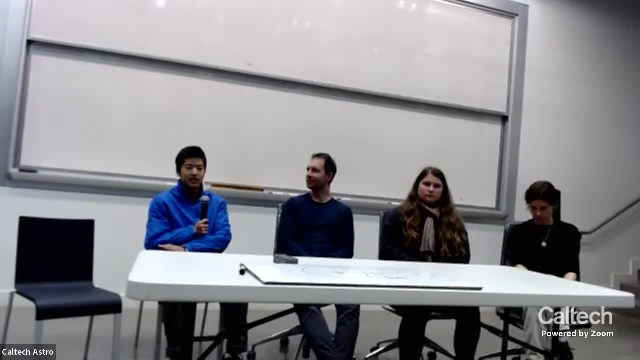 campaign involving pro maybe a dozen different spacecraft, as well as number of- uh, large number of amateur astronomers as well and, of course, many standard ground-based professional observatories as well, and so this comet was observed by the hubble spitzer, even one of the mars rovers, i. 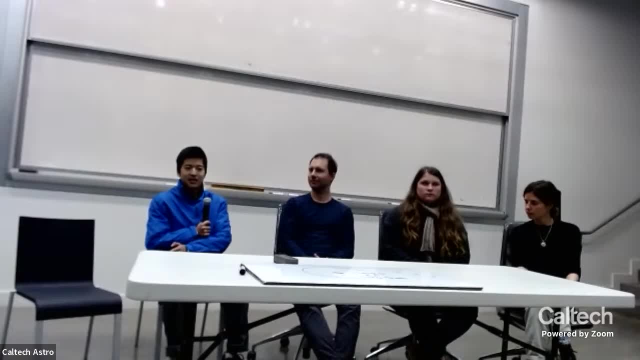 think, got it uh spacecraft around. uh, the messenger spacecraft that was around mercury at the time also observed it, as well as the solar coronagraphs we have in the vicinity of earth among a huge armada of other things. how bright was it, uh. so this comet peaked at around magnitude. 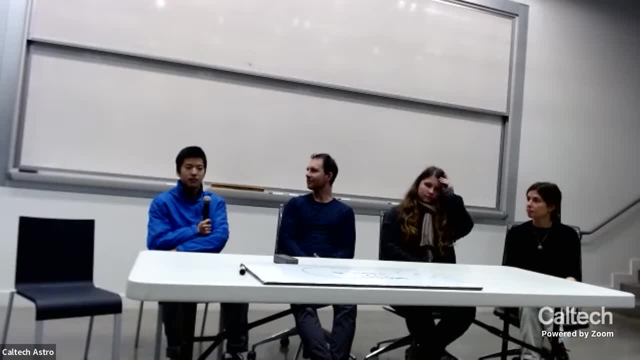 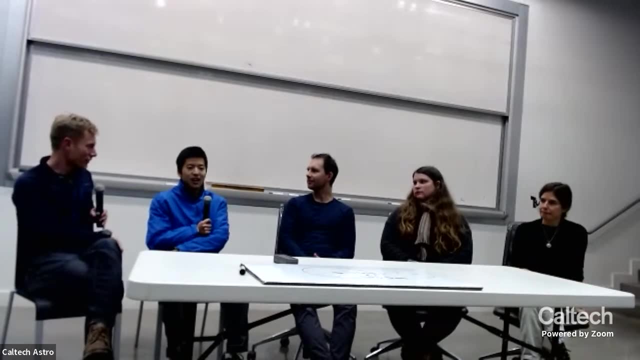 minus three or so. so it's about the brightness of venus. yeah, not quite as bright as venus, uh, maybe about, yeah, somewhere between jupiter and venus in the sky, uh, but it only got to this brightness when it was a few degrees away from the sun. 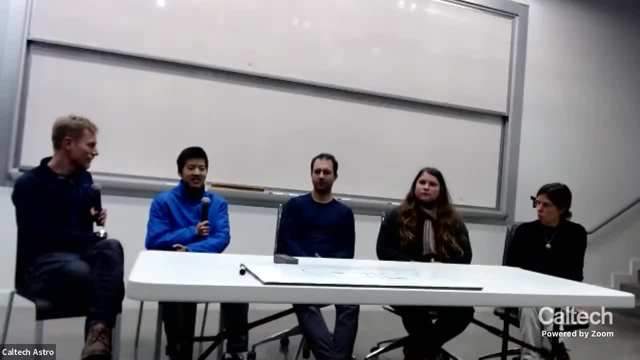 and the hopes were that it would stay intact on its passage around the sun and then it would get super bright in the weeks after thanksgiving, which it didn't because it was destroyed by the sun. and so in the past, if you look through the past few centuries of like bright comets, 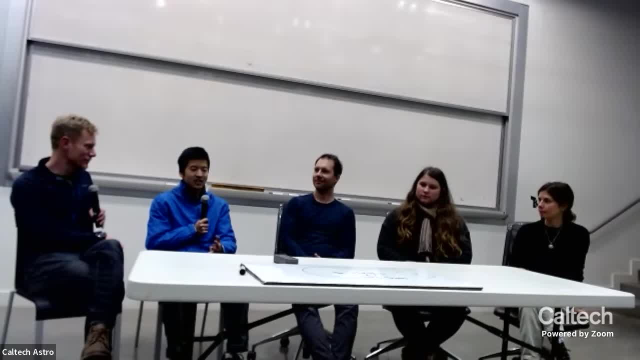 the vast majority of extremely bright comets that you see in historical records, the ones that, like, have tails stretching like 100 degrees in the sky that fuse by like why is there a random search light that's like shining into the sky? those, the vast majority of those, tend to be these so-called sun grazing comets, because comets that they're. not intrinsically that bright. i mean, they're just like a ball of rock and some ice that's, and they're like really small few kilometers in size. but they only get bright because they're heated by the sun and they get heated by the sun a lot if you put them really close to the sun. 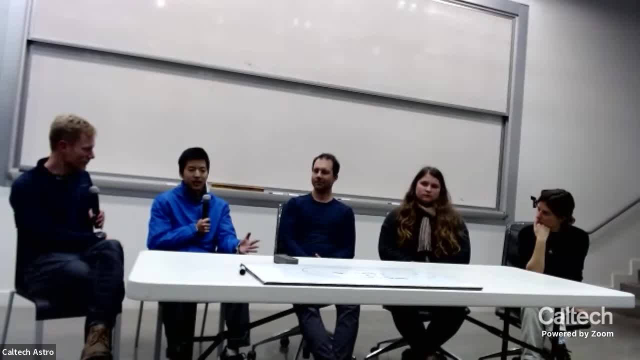 and so the brightest of these are these sun grazing comets that you basically put right up to maybe like one solar radius away from the sun or so, or less than that, and they can potentially get very bright because of all this stuff coming off of it, or at least, if they're big enough, more than like a couple kilometers in size or so. and so the last 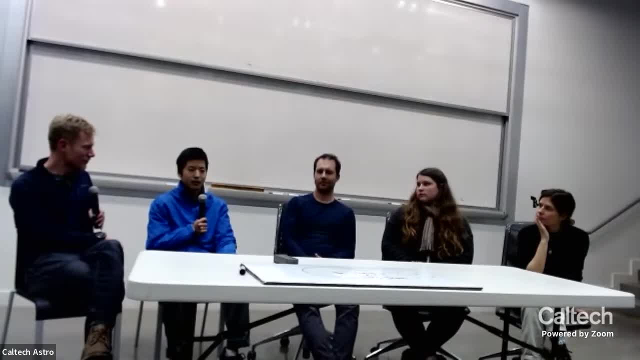 really bright. one of these was probably back in 1965, which is comet ikea seki, which got up to about magnitude minus 10 or so in the daytime sky. so it's visible. it's about as bright as the moon, wow, and you can. there's stories of people to basically just hold their hand right up to the sun block it. out and there's basically this just bright comet that's like right next to it. that's wild, and so there were some hopes that this comet- ice on would do that, and unfortunately this was not a multi-kilometer size comet. this was a probably around half kilometer to one kilometer size comet. 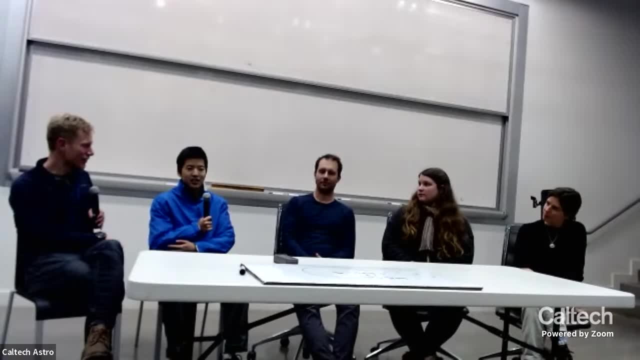 big enough to survive its way around and so, uh, it did not end up being a particularly bright comet, in the night sky at least, uh, but on in the anticipation that it might be extremely bright and interesting, there was a huge campaign launch to study it. and if you go and online and like, look up. 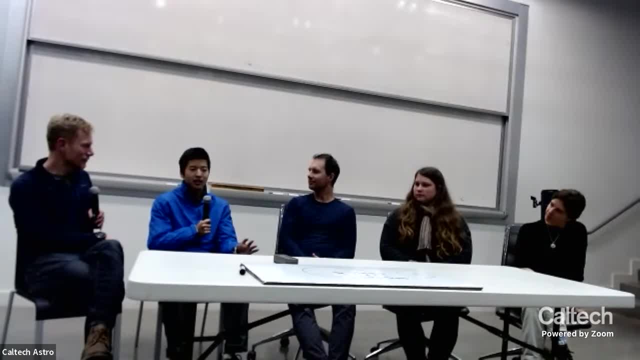 papers relating to like the comet ice on observing campaign. in fact, you'll find a large number of different papers, including many of them, and the other one is the comet ice on observing campaign. in fact, you'll find a large number of different papers, including many of the עםec 스데 brain use pieces- they get called as gyro enters, but which are 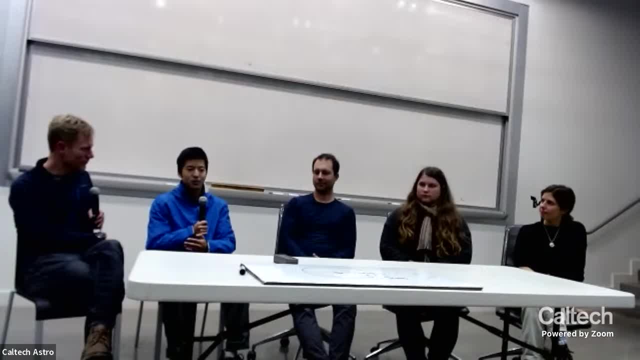 um, using that true aerial, using that compiled results from, like the amateur campaign where people- because like professional astronomers, we can't like monopolize all the observatories around the world to like, look at a single comet as much as we'd want, to as much as you'd want. 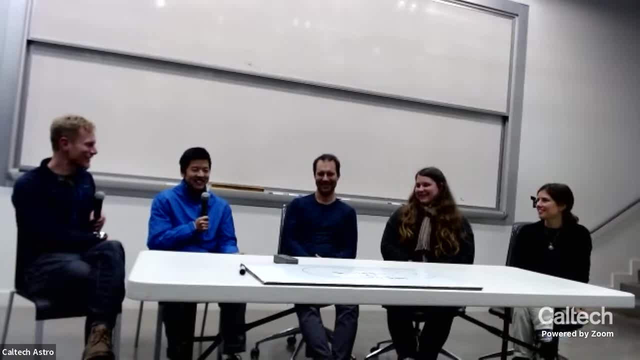 i mean, i dig comments, i like comments, but everybody, everybody, yeah, everybody wants to use it for their own science. yeah, and. and so we can't like all, 100% of it. all the observatories: time to like look at a comet, to see how it like rotates, and stuff. 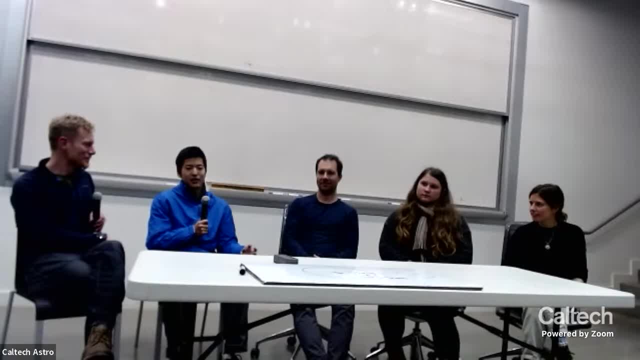 And so it's in times like that where contributions from amateurs are extremely useful, because they can help cover and fill in the gaps in what the comet looks like in between, And so we can see like the jets of gas and dust that are emitted by the comet as it rotates. 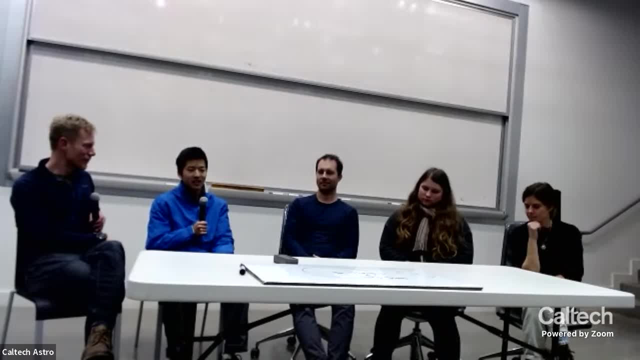 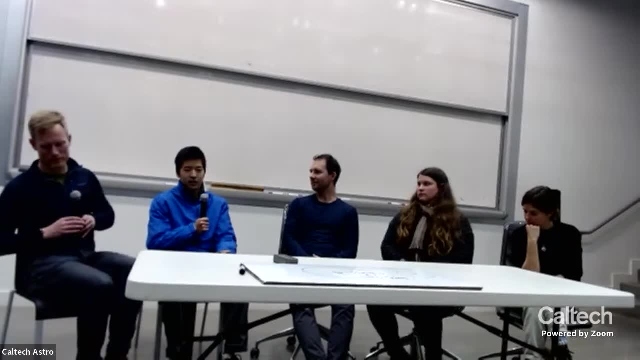 which helps us figure out things like what's its rotation rate and how big it is- yeah, exactly, And things of that nature that are just hard to find from single observations, And so there are campaigns like this, And so that was the big one. There were a few more more recently. There's the comet 4145 and 46P campaign, basically just set of three periodic comets that came by in like 2017 and 18 or so A lot fainter, but it's a lot more than that. 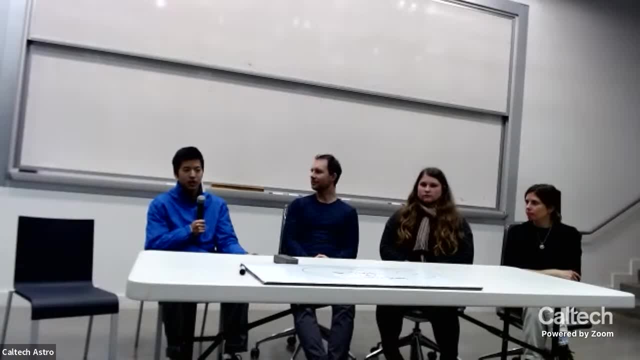 It's a lot more of a similar nature involving the amateur community And as more bright comets that are not of the Well. so there are basically if in the sky at any moment there's usually at least a dozen comets that are observable at any moment. 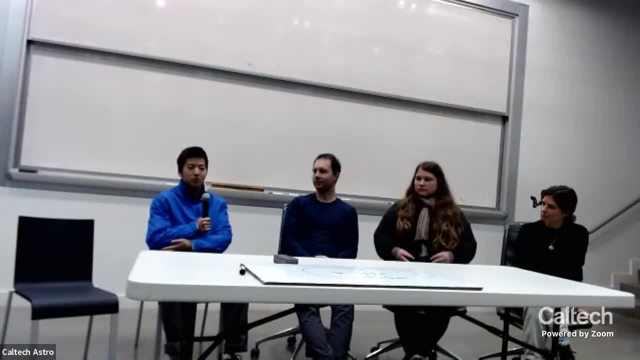 And so every now and then, there are ones that are brighter than others And as more, and those are found by future surveys- and most of these are just surveys- that are constantly scanning the sky Every clear night, looking for anything in the sky that moves. 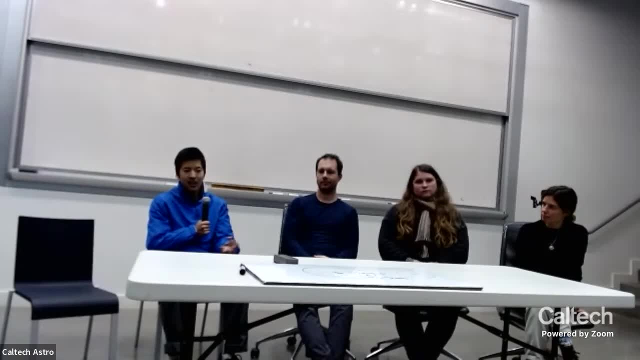 most of which are asteroids, which are not very icy for the most part, So do not emit gas and dust, but some of these moving objects do. Those are the comets, And every now and then one of those will have an interesting orbit of some sort. 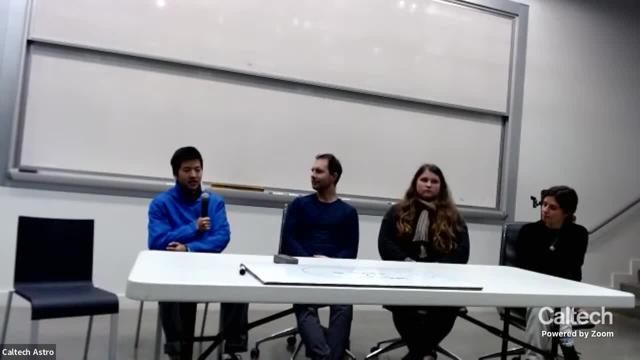 whether it's that it takes it very close to the sun or it takes it close to the earth, And when that happens, there will be campaigns of this sort that involve amateurs and professionals to generate better science. Cool, Thank you, that was great. 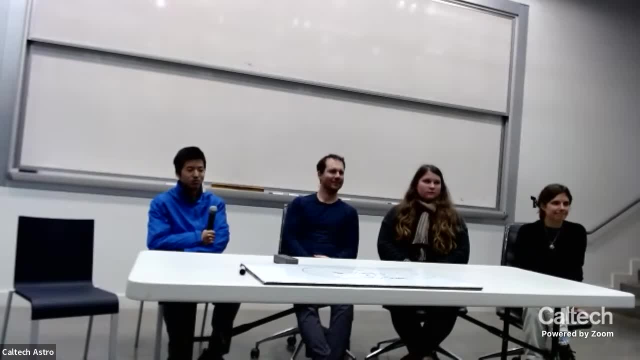 I love these things because I learned a bunch of stuff too. Thanks for coming, Andreas. this is for you. I saw a couple of days ago- I saw a story about that- the JWST- that someone observed with the JWST. 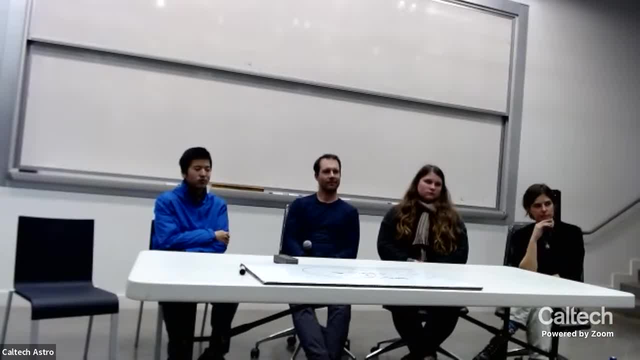 that there are galaxies that formed like, that appear to form like 600 million years after the big bang, much earlier than we previously thought. So I guess I'm just curious what you thought if you saw that, what you thought of it. 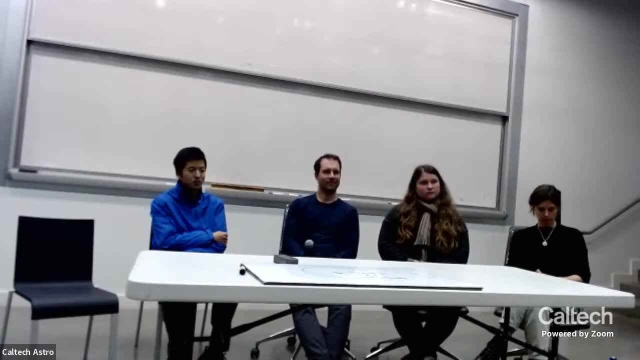 and then, if that is confirmed, how does that change our understanding of the timeline of the formation of the early universe? Yeah, I mean it's very interesting, right? I mean, before JWST we didn't even know that these things exist right. 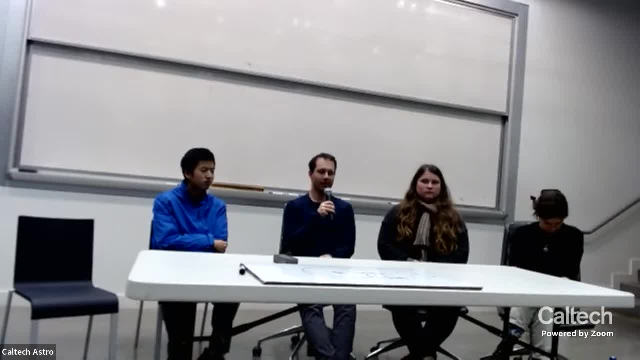 Because we were just limited in what we can see. So give it a bit of background. So how do you find those galaxies, right? So basically you have this. I think it came up when Cameron was answering question. there is this redshift, right? 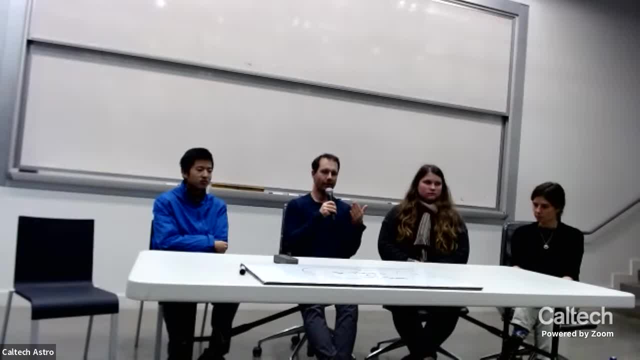 So basically, what happens is because of the expansion of the universe to galaxies that are far away, actually move away from us, And so that's basically like a Doppler shift that we can, you know, hear when a car passes by, right, so the sound changes depending on if the 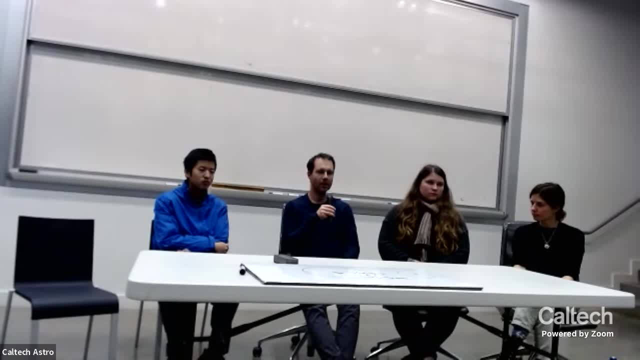 car is approaching or driving away from us, like the ambulance or so, um. so the same thing happens with light, right? so when you have something that's moving away from you, it's the light is red, shifted, so it appears red. so i always say, when you have a traffic light and you drive towards the traffic, 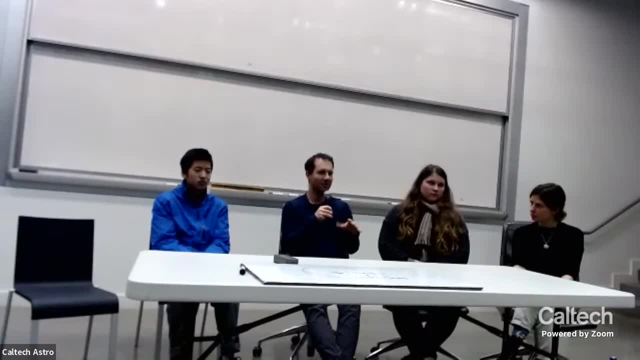 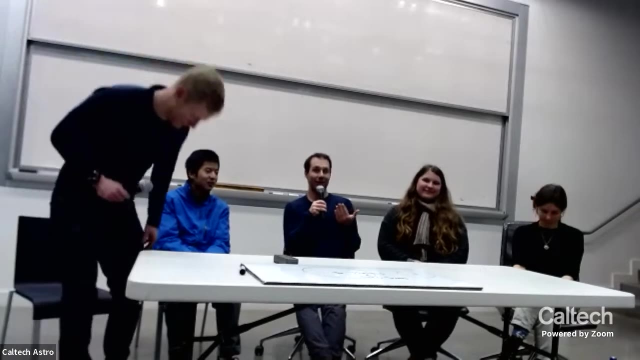 light very quickly. you know, roughly with the speed of light. um, your traffic light turns blue right and when you drive away from it it turns red right, so it's kind of funny. um, probably get a speeding ticket, um, and so so far. so, when you and and then, um, what we found is that when galaxies, 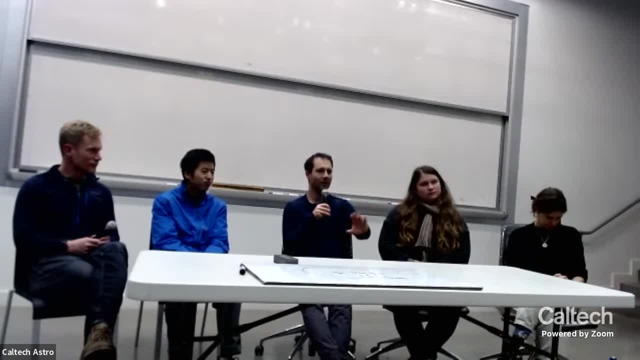 are farther and farther away. they move away from us more quickly than galaxies that are close right. so now what happens is, when you want to observe those 600 million year after the big bang galaxies, you need to look into the red right, because you, you wouldn't see them by eye, because they are so redshifted you, you can't see. 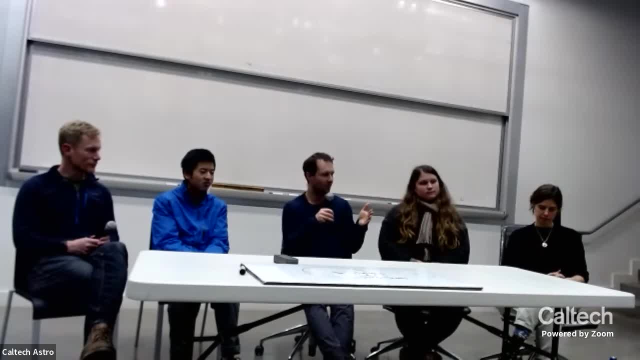 them. so they are the, the red part of the spectrum that um jessica showed before um, and so if the jwc, we're finally able to see them right. so we- there are different types, uh, challenges, how to measure them. so we can take a spectrum. so we look at some emission lines and just see how red 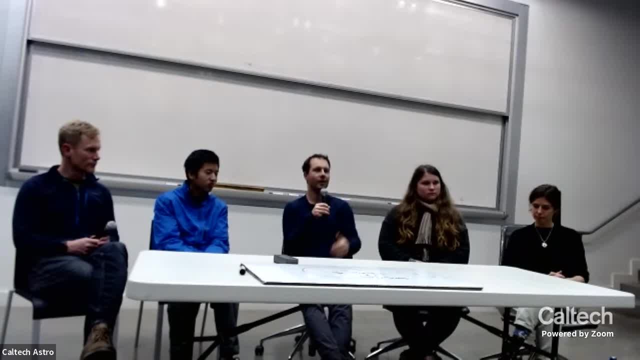 shift that they are and that's how we can get a red shift, and so we know a distance to those galaxies, um and um. and the other way is to just look at the color. so we take images and see, you know, there's a red dot. okay, that's might be a galaxy that's formed 13.1 billion years ago, which. 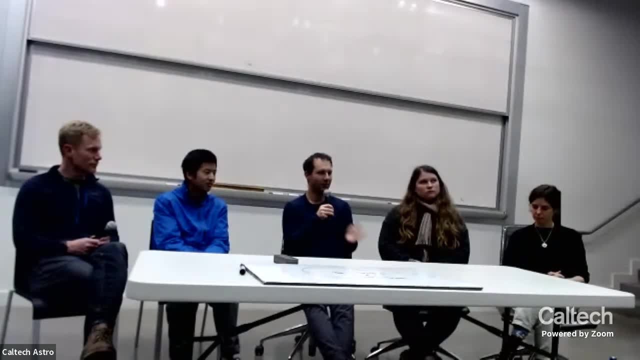 is 600 million years after the big bang. age of the universe is about 13.7 billion years. and so what? what was kind of amazing is that now we can actually not only confirm the distance to those objects and therefore the age, so in the, in the cosmic time, right. so 600 million years after big bang, we can also, with the spectrum, we 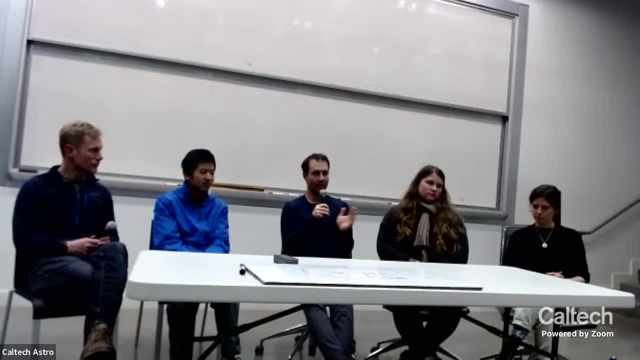 can see how many stars they are forming. what are the chemical compositions? i mean not like we don't see, like uh all those lines in as in the, in the exoplanets, right, so it's, it's much uh broader what we can learn about, so, but we can. 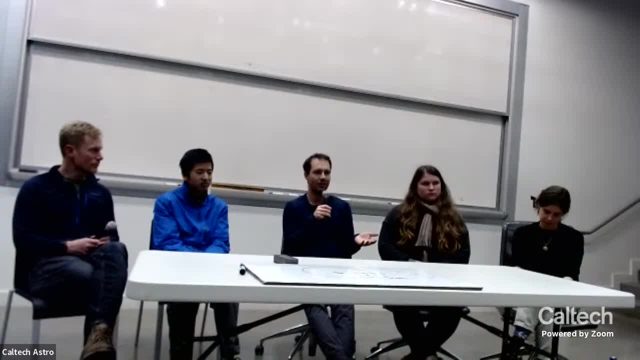 you know, learn how many metals are in those galaxies, right, how much dust in those is in those galaxies. and what's interesting is that some of those galaxies, they are very they have, they have a lot of metals already, right? so, and what does this mean? right, you know, in order to create metals, 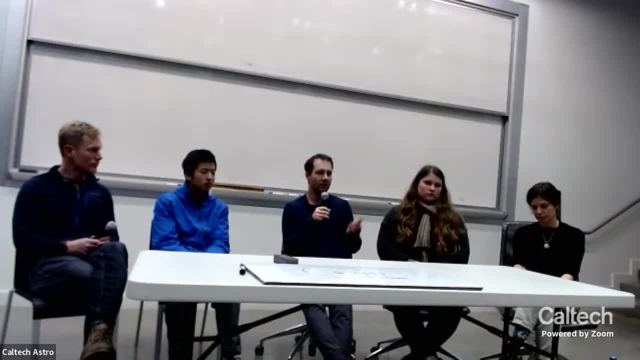 you have to form stars, and that takes a while, right? so you need a couple hundred million years to form enough stars to have a metallicity that's about the one that you know has our military way. um, and so so those detections. they basically allow us to constrain our models of how galaxies 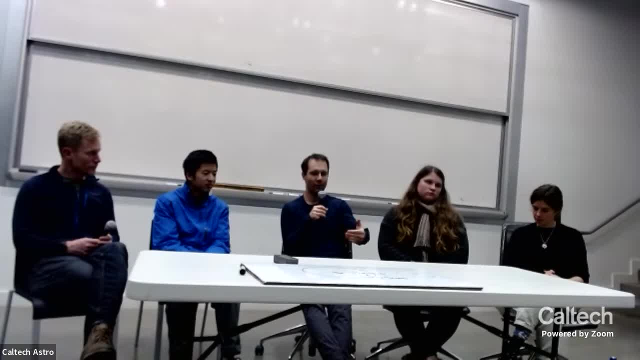 are forming right, and so the farther back you go in time, so the higher redshift, and you find those galaxies. it kind of pushes our models a little bit, and so what we have found is there are very massive galaxies, so 10 to the 11 solar masses, so 10 to 11 suns um, or 10 to the 10, which is very. 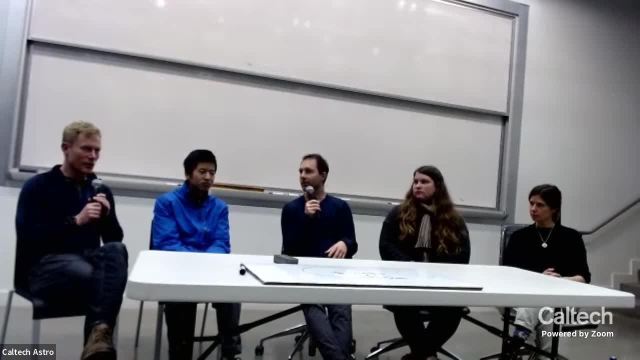 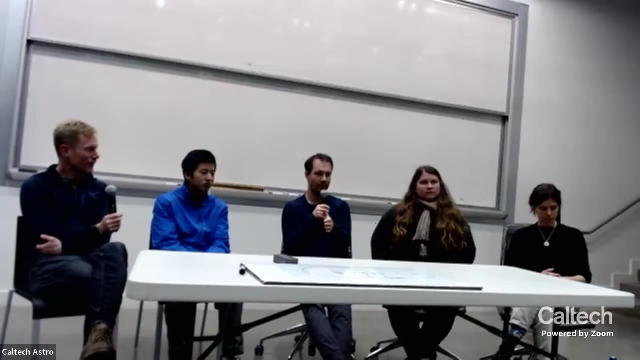 with our own milky way, which is 10 to the 12.. yeah, roughly, right so, almost as massive as our milky way, but formed 13 billion years in the past, right? so how do you make this thing? and much smaller, right so? galaxies, they don't only grow in in. 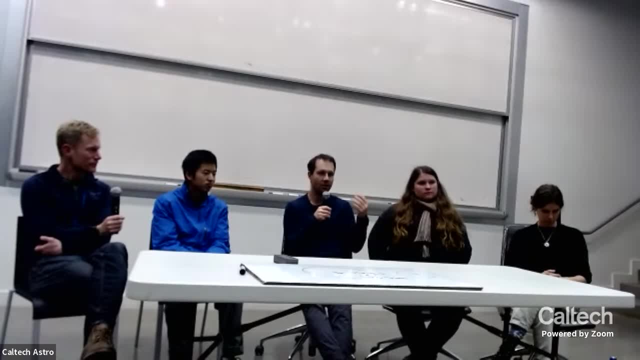 in mass, right, because they're forming stars, like our milky way forms about- i don't know- one or two stars per year. those galaxies, um, maybe form hundreds, right, when you go back in time, um, but they're also physically small, smaller, right, because they're also growing in size, right? so you have those very compact little things. 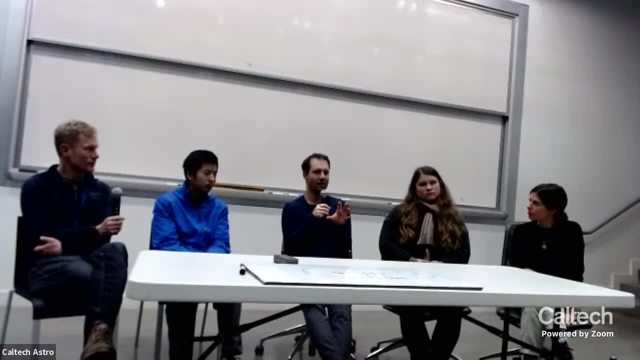 um, factors of 10, smaller than our milky way, um, and they're forming a lot of stars, and they already are that massive, right? so so, um, but again there is. so this can channel, challenge the whole understanding of our universe, right? so how mass forms, how galaxy clusters form, um, how you know? 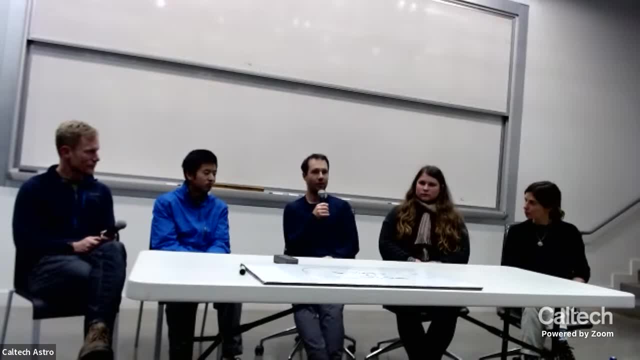 galaxies form, um, but, on the other hand, there are a lot of uncertainties in these models as well, right, um? so just give an example. so when you, when you have one of those star for me clouds- right that that you showed in your talk, um, and you form stars, we don't really know what's the distribution of. 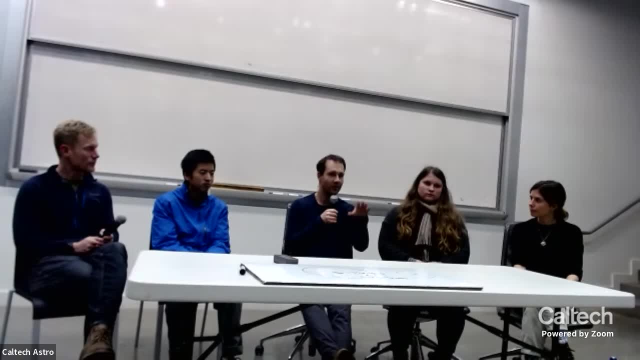 those stars are those mostly heavy stars that are being formed, or others mostly low mass stars are being formed right and so this what we call the initial mass function for star formation. that might change over time. so in the early universe maybe you form more massive stars, more, more massive. 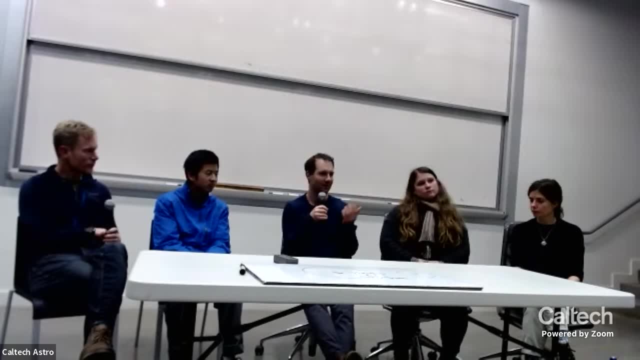 stars than you you form in in today's universe, like in our milky way, right? so these are model uncertainties and if you play with them, you can actually make this work, right. so it's a similar thing that cameron was saying before. you know, there are some knobs you can turn in your models. 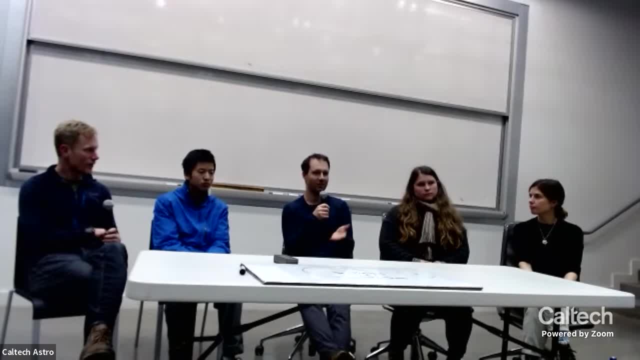 right, some simple explanations to to explain those massive galaxies in the universe, yeah, but but just from a, from a personal perspective it's. we were trying with hubble and with keck really hard, you know like 10 hour exposures, you know- to get like a single line of this galaxy. and now jbl, jwst, you. 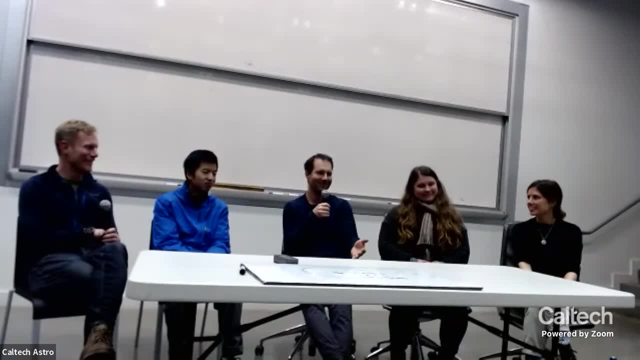 know an hour, you get the whole spectrum, you know. so it's it's really um, it's really amazing what we can do now and um, and these are only a couple right, so we will find a lot of more of them and we can actually, at some point, um get the statistics. 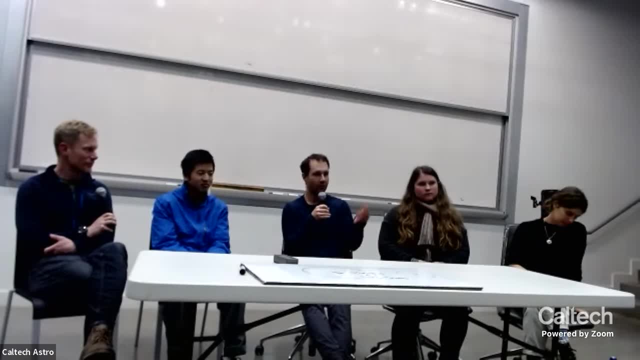 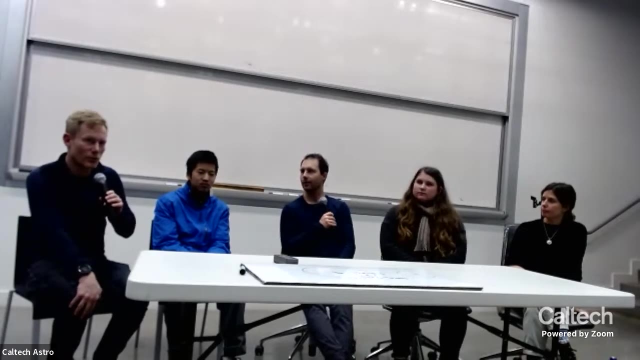 right of how many, uh you know, of metal, more metal rich galaxies are at this epoch in time and and that really constrains our model of galaxy formation. so it's very important. yeah, we're definitely, i'd say, at at this time, because of the launch of jwst, at a transition. 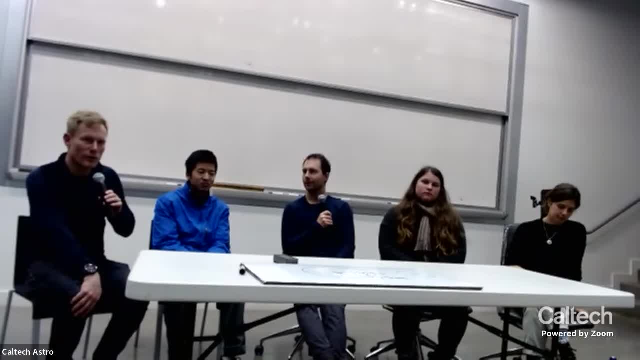 point in our understanding of of how things are evolving in the early, early universe, especially also what you're doing right with simulations, right so how you form those galaxies, yeah, if we can make theoretical models that are consistent with the observations that we have- and right now not all of them- we can't, like we can't, we can't create galaxies of that mass, that quickly. 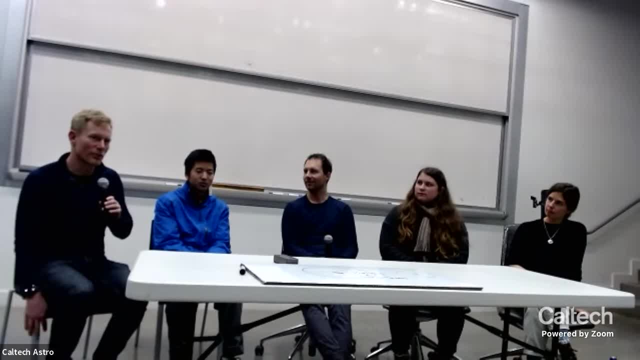 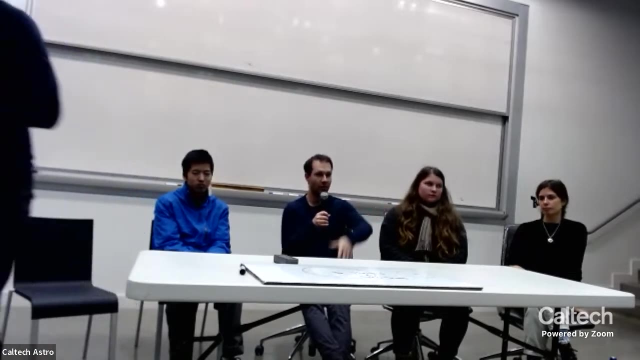 um, not at least with the observational characteristics that exist. but this is always an iterative thing, you, you work with what you have and then, yeah, one other thing is that they're also always selection biases, right. so we find the most extreme objects usually because they have strong emissions. 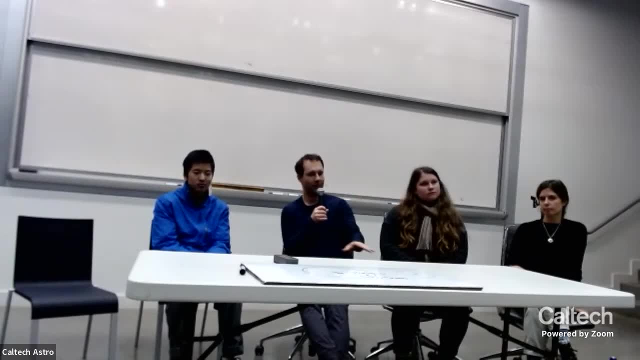 or they have high mass and they break free from organic matter and so they can't be separated really well, or i often imagine a myriad of 말고 but one kind of race in my Explorate Summary. so, uh, I do want to point out that you know, if you sound on video at least some of the suo rahat. 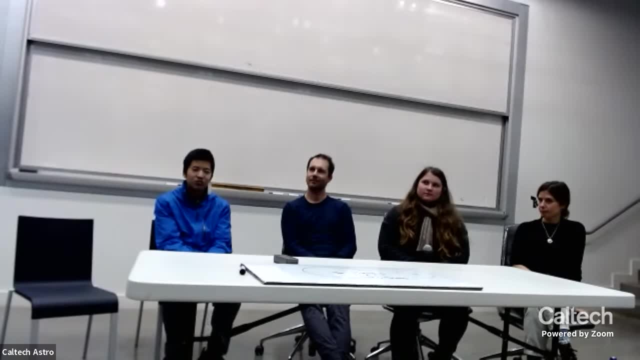 we see stars and they appear to be, at least from our perspective, just like kind of constants. so why do they? you know, what's the time scale over which they die and what? why do they die and what they leave? yeah, this is a great question, and it's something that i'm really interested in. 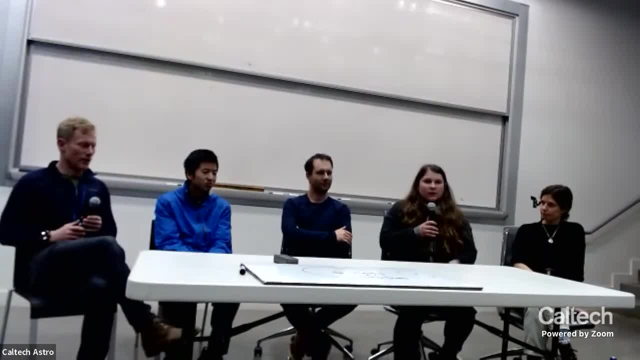 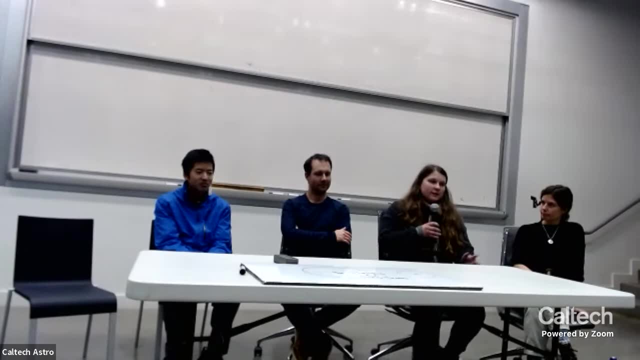 trying to understand the population, not just of stars that are going to die, but then the stars that explode, and we see those explosions and also the population of objects left behind from them, so black holes, neutron stars and white dwarfs. so basically, the basic picture of a star is it is. 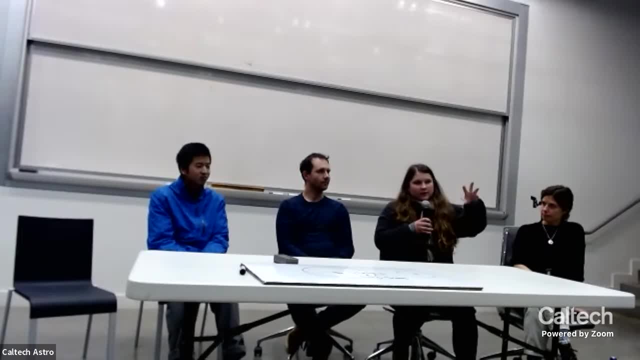 a ball of gas that's held together by gravity and it is held up by pressure, and that pressure you need to have very high temperatures to support that much mass. and the things that's providing your very high temperatures is your are fusing in your cores, so like a hydrogen bomb or 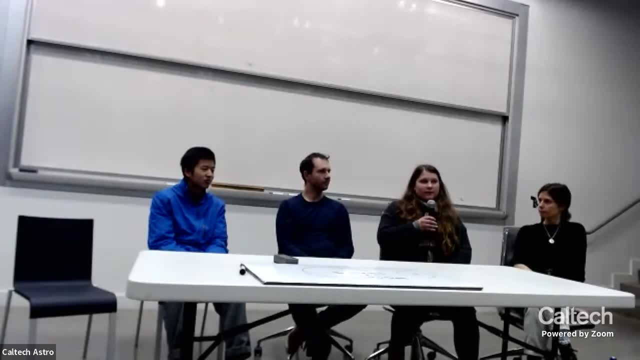 if you remember in the news, maybe a couple weeks ago, there was a hydrogen fusion where you got more energy out than you got in. that's the same thing. that's powering stars like the sun, more massive stars like that. but in order to fuse hydrogen you need to have hydrogen. so there comes a point in a star's lifetime where it's used all of its. hydrogen. it's fused all of its hydrogen into helium. it doesn't have any more that it can fuse and then it needs to do something else in order to support itself. so it's no longer fusing hydrogen. there's no longer the energy that sort of is. supporting the star and it starts to contract. so for a while you can just go on to fusing heavier elements. so you can fuse helium into heavier elements. you can fuse all the way up to on the periodic table, to iron. now when you get to iron you actually reach a peak in sort of the amount. of energy per nucleon. if you go to elements that are heavier, you can fuse helium into heavier elements, heavier than iron. instead of getting energy when you fuse, you actually lose energy. and if you go sort of to the other extreme, if you consider really heavy elements like uranium and sort of, 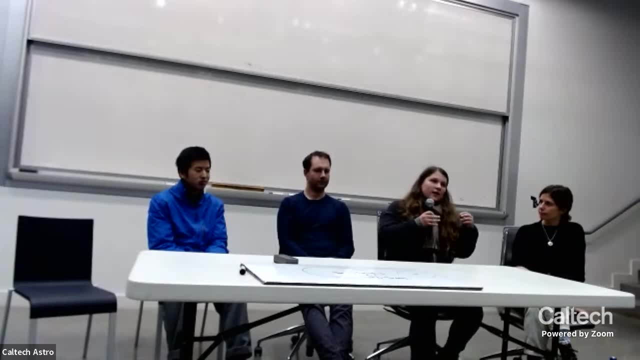 all the radioactive elements. they will fission instead and you get energy from fission. so that's how most nuclear power reactors here on earth operate. but the problem is with stars. okay, they're not. they're not fissioning things. they need to fuse in order to get that energy, and so 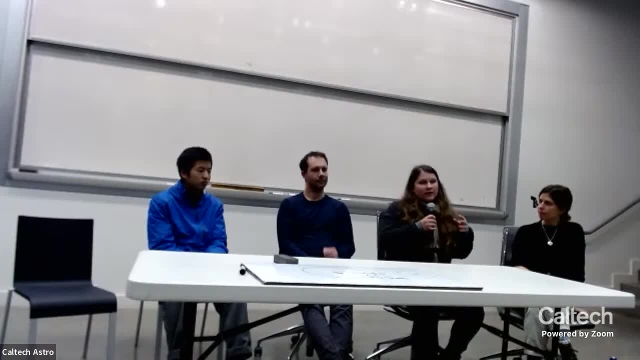 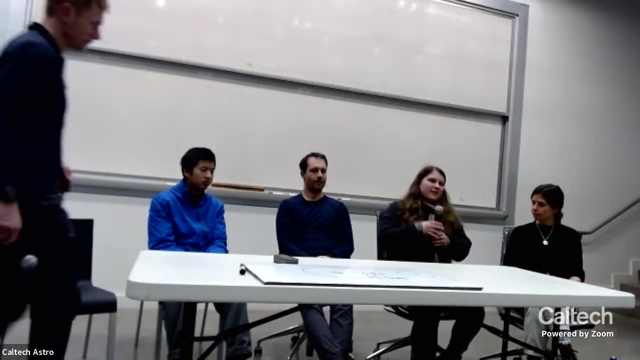 when they reach this iron bit, they have a problem. they no longer have any energy to create the pressure they need to support themselves and they collapse under gravity and from there a couple things can happen. so a star like the sun and stars that are, you know, comparable in mass and less massive, they tend to live longer because they're less bright and so they use up their energy more slowly and their cores sort of won't actually even get to to fusing things like iron. they sort of top out around carbon or oxygen, and they're sort of done at that point, and they sort of blow some of their mass off, and they're sort of done at that point. 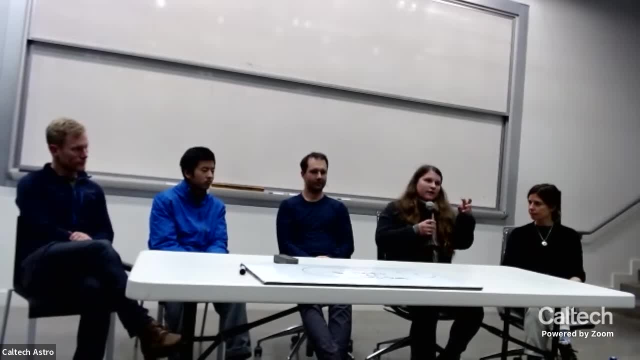 off and are sort of just left with the degenerate core. so the degenerate core is supported not by gas pressure, so by something that's like hot in temperature, but just by, like the rules of quantum mechanics, where you can't fit more things into a smaller thing, and so the degenerate thing. 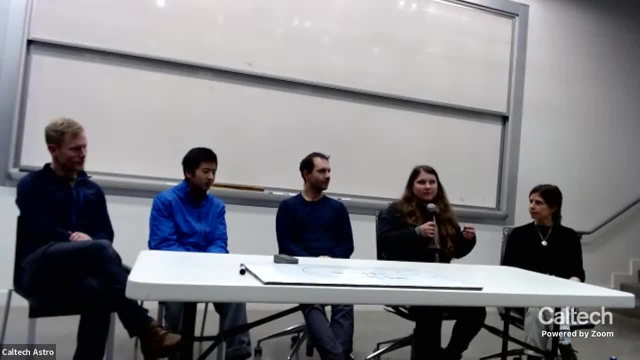 left over for low mass stars like our sun is a white dwarf. so in about seven billion years our sun will sort of reach the end of its ability to fuse hydrogen. it'll puff up in its thing, it sort of blow off its outer layers and it'll just be left with a white dwarf and we observe. 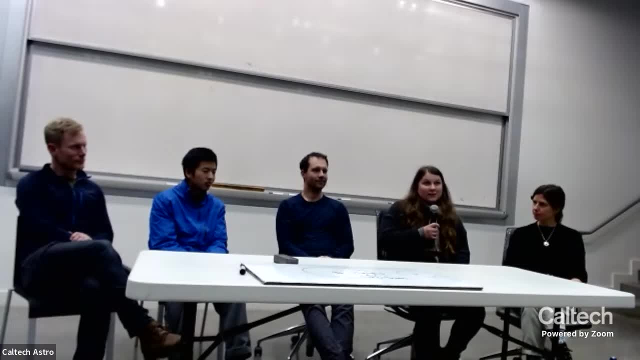 these white dwarfs in our galaxy. the stars that I'm really interested in are stars that are maybe more than eight times the mass of our sun, and when they, they can fuse almost all the way up to iron, and they do something much more exciting than sort of just blowing off their 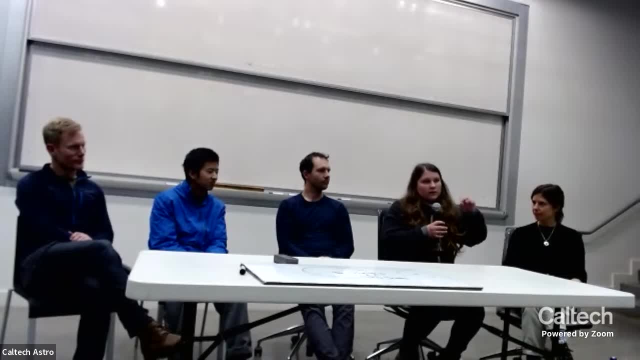 outer layers and being degenerate, they can actually explode. so once you sort of get that last little bit of pressure support lost, your outer layers will come down and they'll hit your hard iron core, that your hard core that can't, can't compress, and so when they hit back they'll bounce like a bouncing ball back out and we see that as an explosion. we. 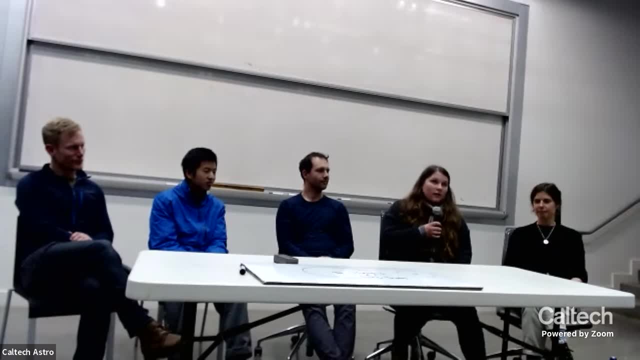 see that as a supernova explosion. interestingly, you could actually sort of have two paths for these massive stars. so either you sort of had this explosion and maybe you're left with something very dense in the center, supported by a different kind of degeneracy pressure. this would be a neutron. star, or maybe you hold on to your mass and instead of exploding back out, you actually have enough mass to collapse in the center, and then you're left with something very dense in the center and anything that can actually collapse in this world entirely to a black hole. you collapse down. 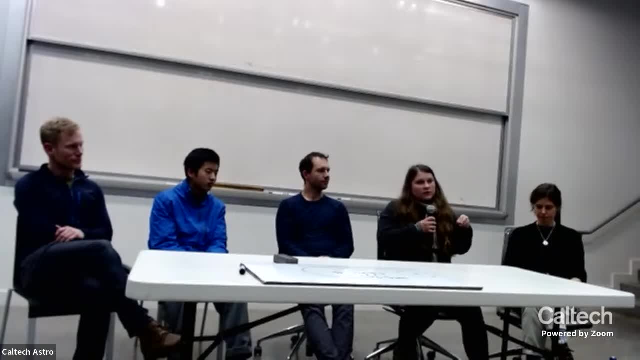 to a single point, um, and i think one of the most interesting questions in astronomy right now, at least for me, is what determines whether a massive star will explode and become a neutron star or implode and become a black hole. would i know that? no, i thought, i thought it. 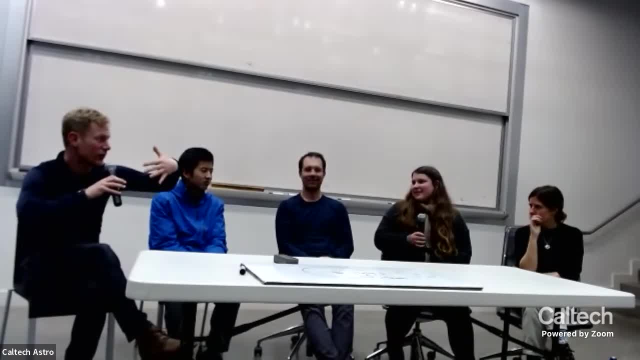 was mostly just determined by the, the mass of the star that's undergoing that explosion. if it's massive enough, oh so it's not. so now I'm in a dive where i hit a cold water美国. i've been to the ocean for 11 weeks making delicious light cruiser intra golg ou. i've made eight of those sinka darkقة. 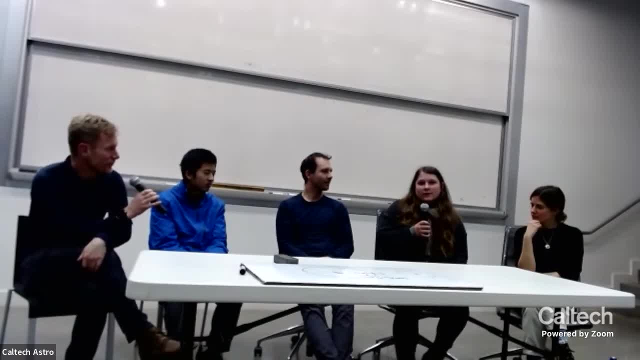 oh, so it's not so. so yeah, you would think, okay, if your star is beyond a certain point, um, then you have enough mass to clap down to a black hole. it actually turns out that your internal structure is much more important, the idea of whether you're going to pull, push back out and get rid of a lot. 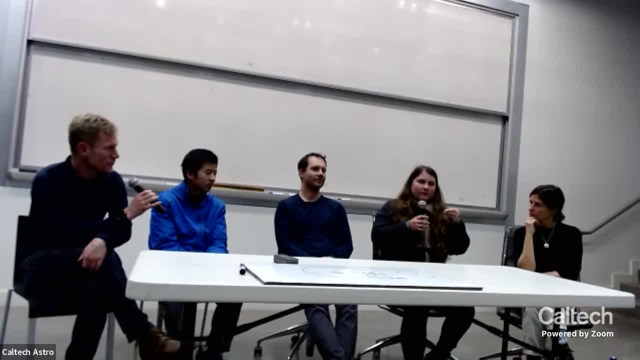 of your material or collapse back down to a black hole. i i feel confident in saying that we don't have a clear answer, um, and it really depends on our understanding. so, uh, people sort of you can come out at this from two perspectives. you can watch explosions happen and try to understand. 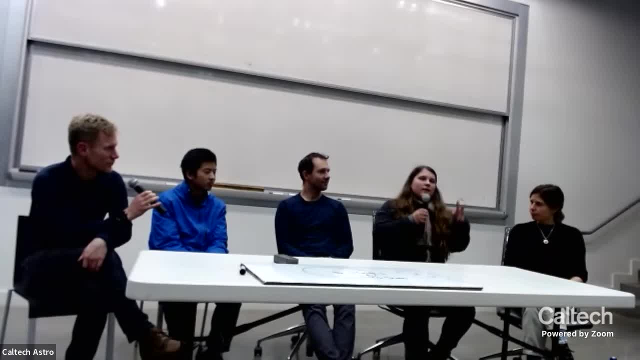 them. the problem is this with this is you mostly see the environment around the star when you see the explosions. you can learn stuff about the energy, you can learn stuff about that, but you don't really sort of know the internal structure of your, of your thing that exploded right before. 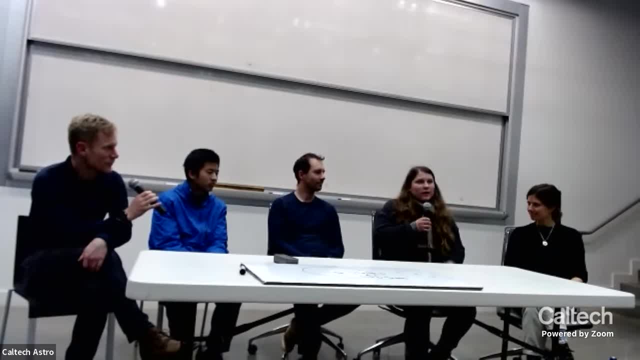 it exploded because you don't. you don't see it, um, you actually just see it right- or it's too far away usually. so most of the explosions we observe aren't in our own galaxy, they are in other galaxies. they're far away. i think supernova 1987a was the brightest supernova in the last 200 years. yeah, less like, yeah, 200 years. 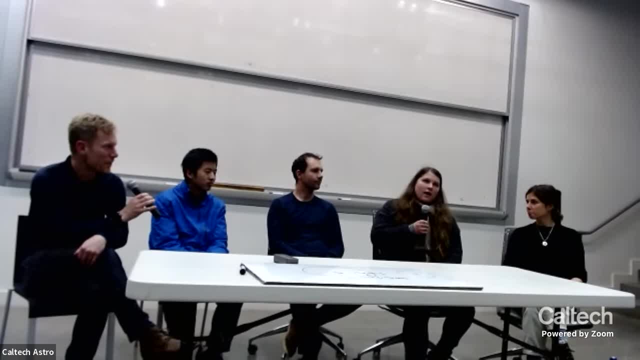 or so, and that was in one of the satellite galaxies, the milky way, uh. but most of the supernova we observe, most of the supernova we see, are all in other galaxies very, very far away. so you can't actually see what exploded. you can just say you look at the galaxy and you say, okay, now there is. 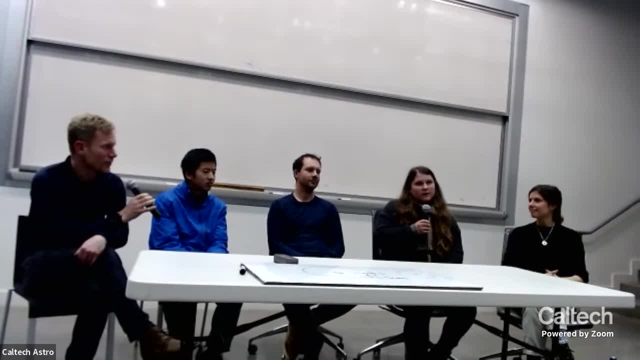 something there that wasn't before. you don't actually see the thing that exploded. so i know there's a lot of talk, especially in the last few years, about the star beetlejuice that's very bright in the sky. it's a red supergiant. it's in the constellation of orion. you've probably seen it if you've looked. 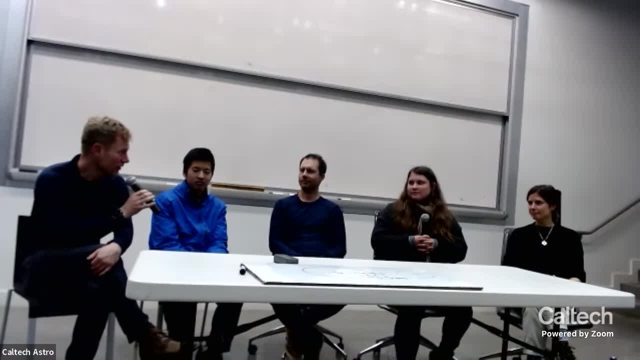 up in the sky, um, and we think it's going to turn into a supernova at some point in the next either days or thousands of years. but if it were to go and undergo supernova, explosion, would, because we have so many observations of it, because it's so close and so bright, would we be able to? 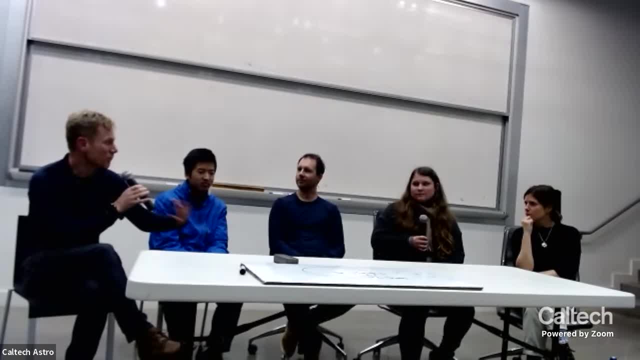 kind of constrain, this mechanism by which a star either turns into a black hole or it turns into a neutron star based on its, the mechanics of its explosion. yeah, so beetlejuice exploding would be really exciting for people who study supernova. we would love a supernova in our own milky way and we're overdue. 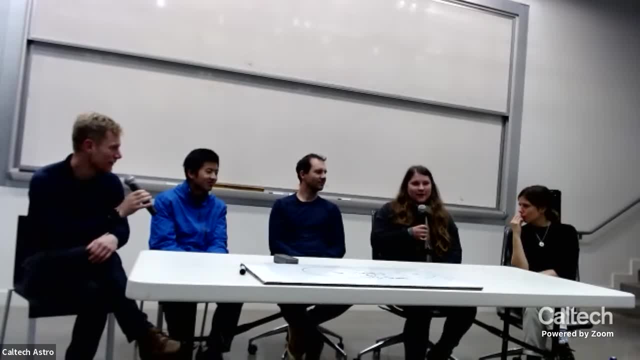 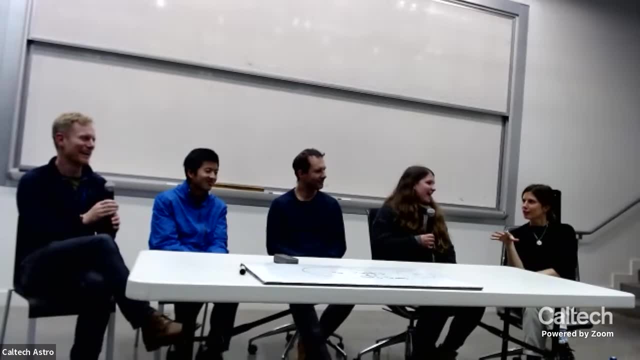 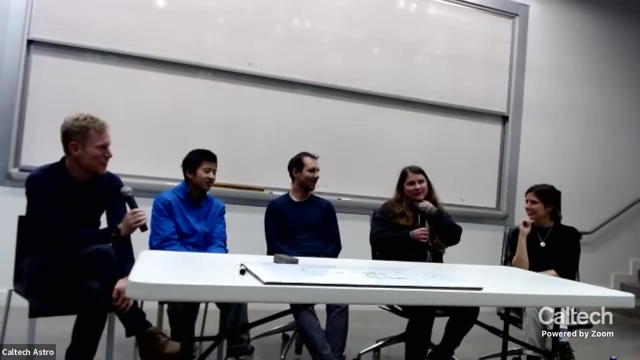 for one actually, so hopefully in the next 10 years we'll actually get to see one in our own galaxy. oh yeah, not too close. um, i'm a little. yeah, beetlejuice is pretty close. maybe i don't want beetlejuice to explode, i want one that's a little bit further than beetlejuice. to explode. i don't want to suffer any ill effects, but i would love to watch the explosion. i don't think so. from what i remember reading, it's not necessarily so close that it's a danger to like blowing off our atmosphere or radiating everyone on the solar system. 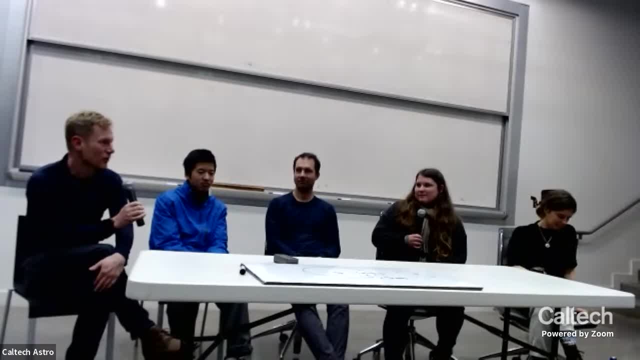 but it would be a spectacle in the sky. it would be much like some of the supernovae that exploded in the last thousand years that were in our galaxy, such that it's so bright that it's as bright as like the full moon in the sky, kind of like key chang was talking about with this comet. 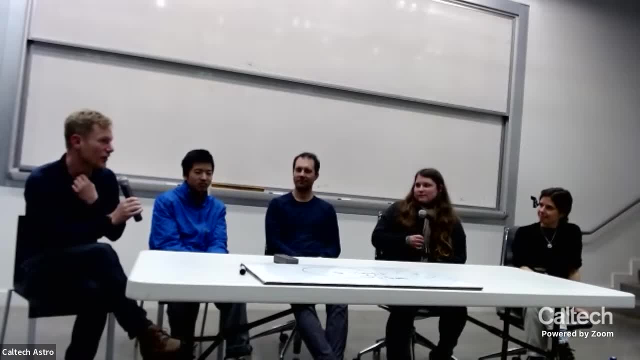 but this is a star exploding and it would be as bright as that for a period of weeks as it slowly fades and that sort of thing. but yeah, i don't think it's. i don't think it's a danger. hopefully it might mess with satellites and stuff, but i think we're in more, i think. 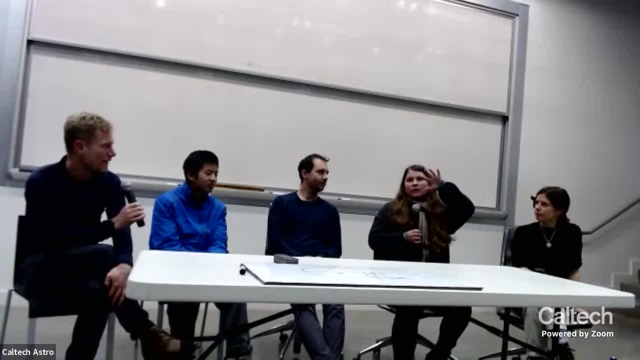 i don't know if it's entirely clear how much the the solar wind will prevent stuff from getting in. i think i think most people think beetlejuice will be will be fairly safe. i think you have to be a little bit closer. it's a few hundred. yeah, i don't. i don't remember exactly. is it eight? 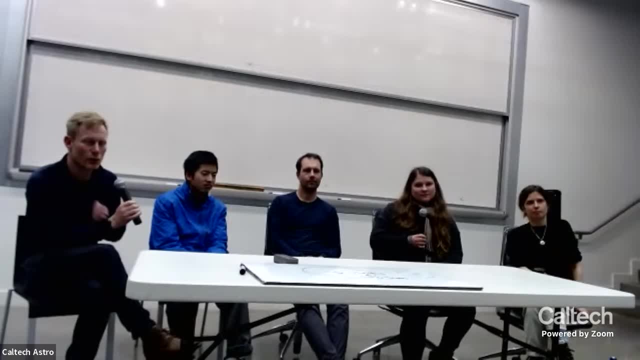 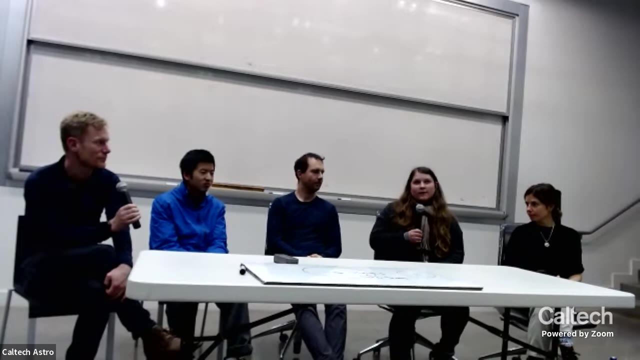 yeah, it's a few hundred. yeah, it's pretty far. it's not like alpha centauri or something. yeah, yeah, yeah. but again we would have a similar problem where, with beetlejuice exploding or any other star in our own or in our own galaxy, a you can't see. 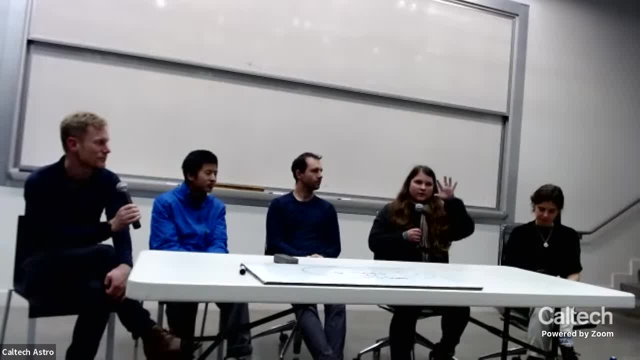 into the interior of a star. just by looking at it, you sort of just see the photosphere. it's like trying to look through at the bottom of the ocean. um, just by like looking at the surface. it's really really challenging. um, you can do. uh, there's a technique called astro seismology where 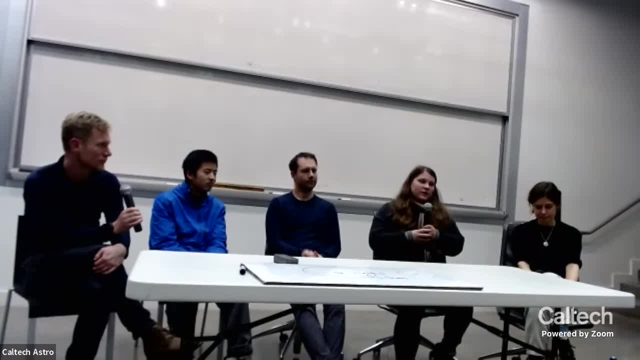 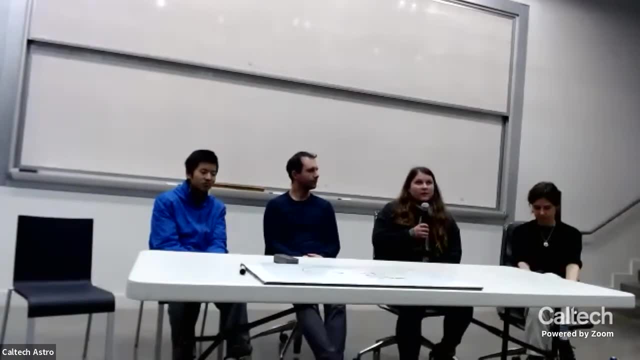 you sort of just look and see how the surface of a star uh is changing and that can tell you a little bit about its internal structure and that's something that would be really helpful for us to really interesting uh for red super giants, i think one of the most interesting um probes of the 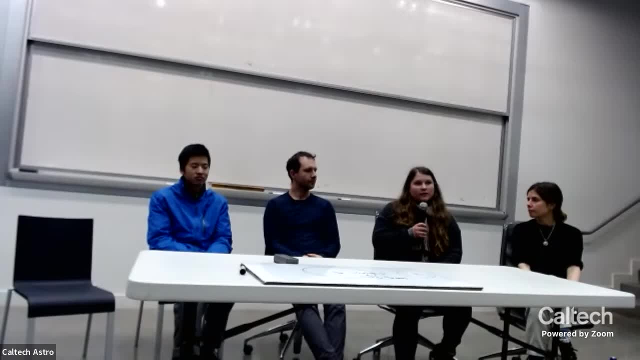 interiors of massive stars, especially in our own milky way, will actually be neutrino emission. so neutrinos aren't like um, like photons, which will get stuck in matter right. neutrinos will mostly free stream out um and then we'll be able to see those. so you actually should detect a whole bunch. 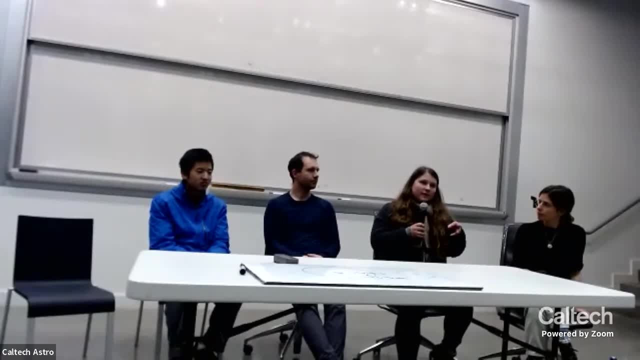 of neutrinos before the actual explosion happens and i think i think those neutrino detections will tell us something extremely interesting about um, about the supernova explosion itself, because it's going to be probing that structure at a at a very early time in the explosion that you just don't 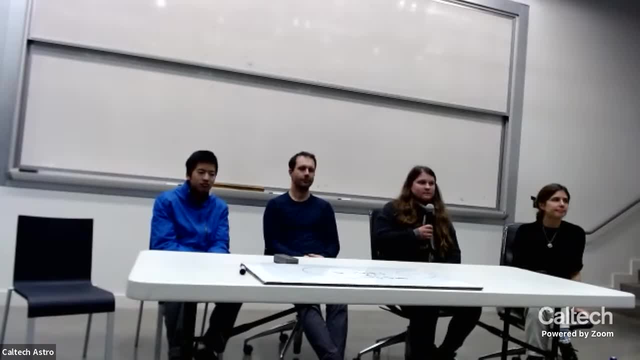 get with with photons. if beta juice explode, would that affect any of the telescope or any of the equipment we have here on earth? that would affect how we view space. so you would want to adjust your exposure times based on how bright something is. just because something is bright in the sky doesn't mean it's going to like damage the telescopes. 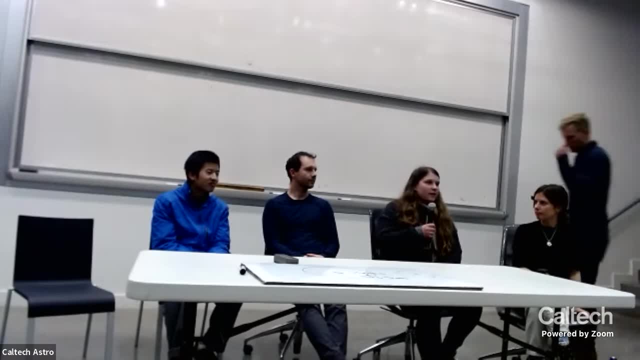 right, the sun is in the sky all the time and it's very bright, um, and you choose where you point things, um, appropriately. so, with something really bright, you just don't have to, uh, collect as many photons. you don't have to collect photons for as long to get the same number of photons as you do. when you're looking at something that's really dim, but it wouldn't like damage our telescopes or anything, if that's what you're asking, yeah, yeah, so there are already, depending on your telescope and sort of uh, your tolerance for light pollution and sort of what you're observing is like how close you can be to the moon or how close. 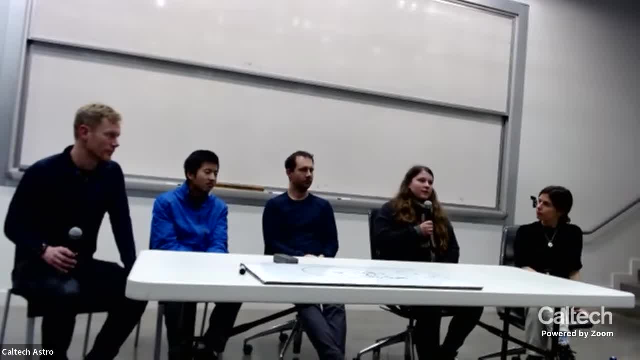 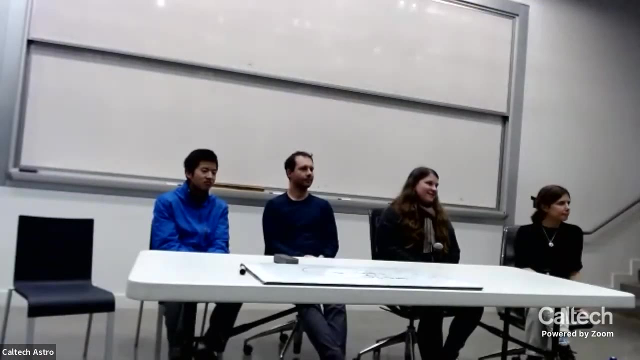 you can be to twilight and stuff, so it definitely would be sort of important to keep that in mind, something for astronomers to think about. of course, beetlejuice itself is already still quite bright in the sky. all right, uh, last question, i think for the night. um, this goes back to what you said about the redshift galaxies, but you said how? 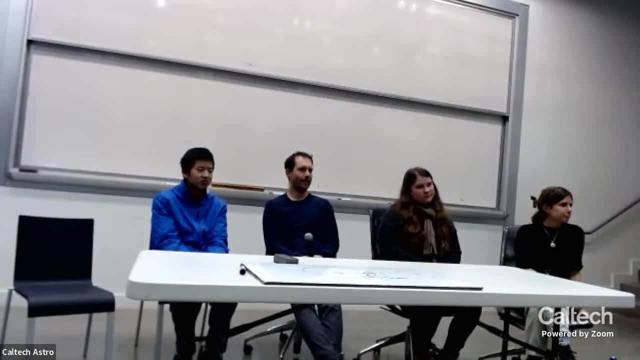 we could tell the age of the galaxy because of, like, the redshift and how far it is and everything, but i'm wondering what are the other methods to measuring the age of a galaxy that are closer to us, like how do we not know? or how do we know that a galaxy that's close to us isn't the same age as? 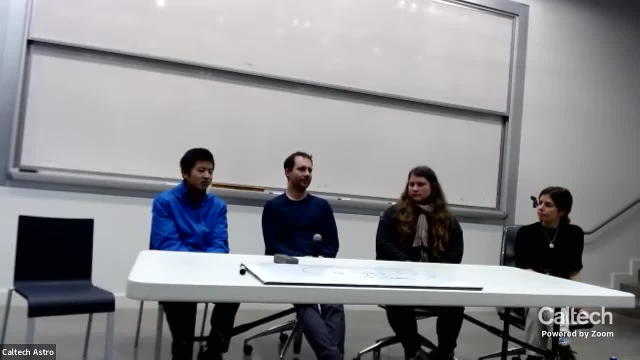 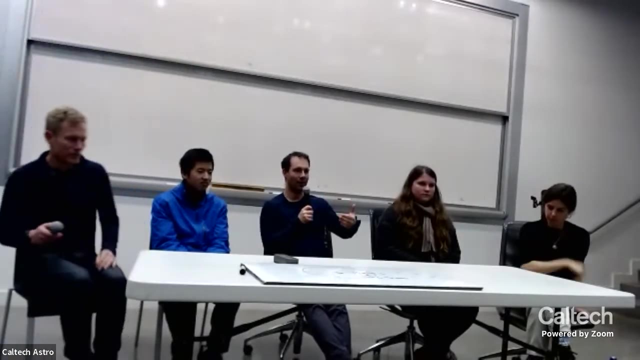 one that's that far and just because of, like, the distance close to us, you know, right. so that's so there. so there's the. it's basically there are two different things, right. so there's the, the redshift of a galaxy which tells you how far away it is, and therefore, how long the light has traveled right. so if it's 10 billion years, it's 10 billion light years. so you basically look 10 billion years into the past, right and, and then there's the maximal age. so, and then you know at what time, you know what the age of the universe was. so 13.7 minus 10 billion is. 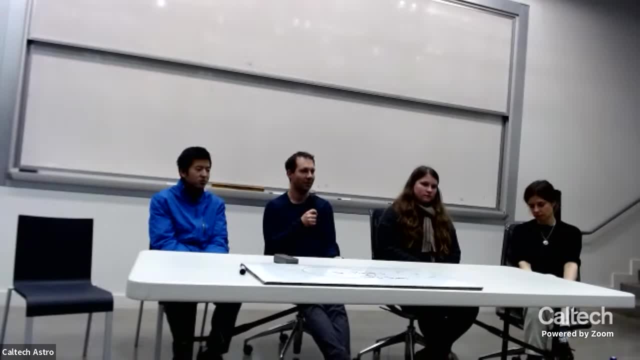 like, uh well, 3.7 billion years, right, and that's the maximum age, because you can't form a galaxy before the universe, right, and then there is the, the actual age of the galaxy, right, so how long it has been forming stars, or when it did start forming stars, right, so galaxies, um, so how they actually form is, is basically you, you. 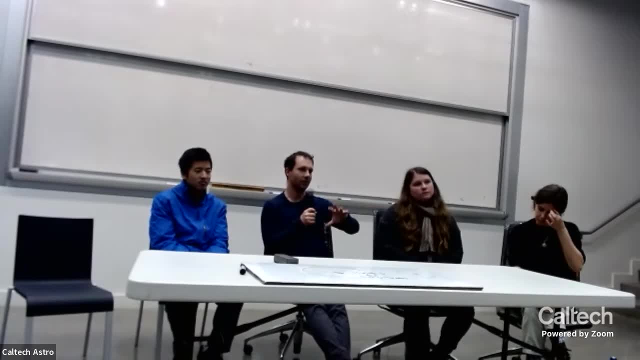 have a structure of dark matter in the universe right and um and and that builds areas where you have more dark matter and dark matter is basically has no interaction except through gravity. right, so you can flow through you, you will notice right. but if you have a lot of dark matter, you you have a 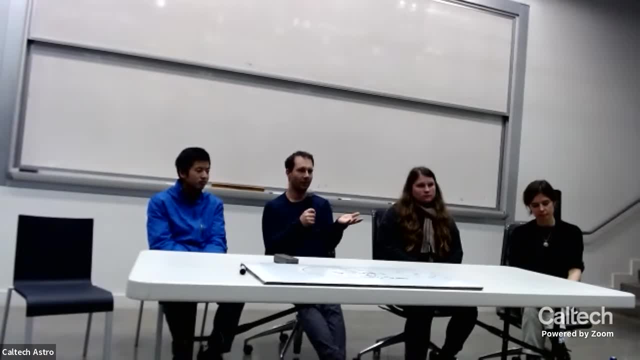 gravitational attraction, right, and so that's what happens in the early universe, right? so you have this, this web of- it looks like a spider web, right. um, of dark matter that forms um, and, and then you have gas in the universe, and so this over densities of dark matter. they attract the gas and it flows. 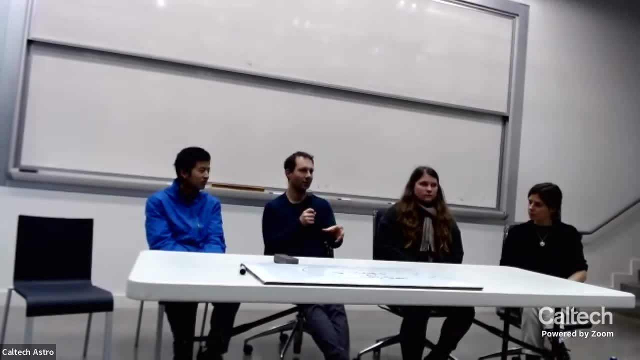 into those dark matter, over densities, and then the stars are being formed, um, as we heard before, by basically construction, contraction of the gas, heating up, and then you have- uh, you basically have to ignition, and you, you have stars, and then you build many stars and then you have a galaxy, right? so? so when this, this process, form uh starts, that's. 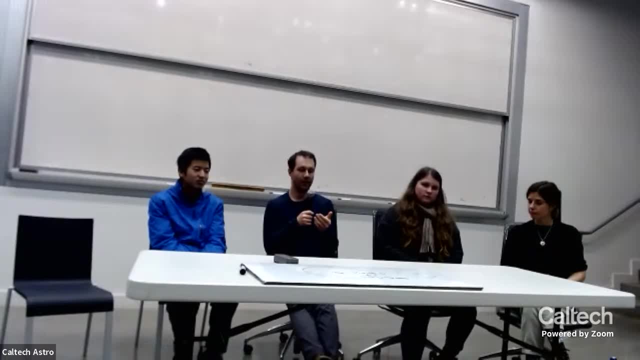 basically the age, what we call the age of a galaxy, um, and it's not easy to measure it. there's a there's a gigantic uncertainty on that right factor of two to ten, right, um, but basically what we are doing is we observe the light of the galaxy. 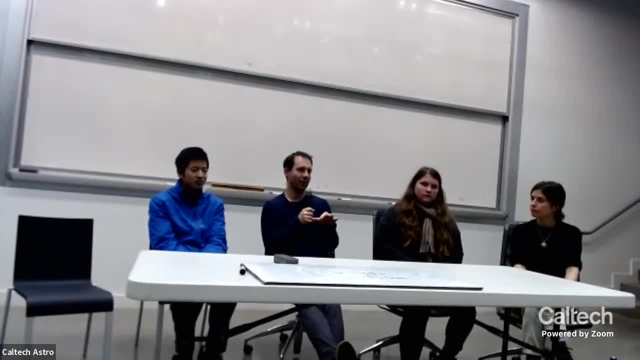 um, and depending on what kind of stars you're forming or you have formed, you either have more red light or more blue light right. so if you have stars that have been formed in the past 100 million years, you will have a lot of light in the UV right, and so when you look at the spectrum or 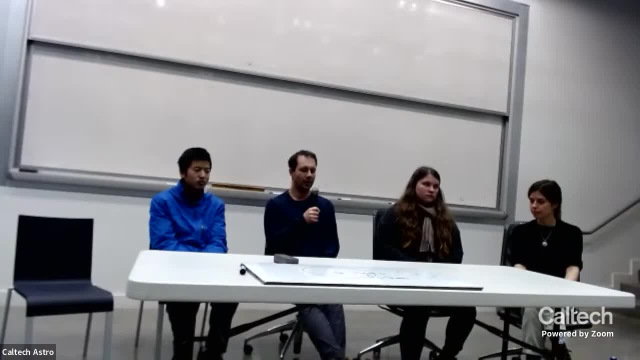 at the, the color of the Galaxy. it will be blue, right, um and um and then uh, um. if you have an older Galaxy, you have more the old and massive stars that still remain. right, because, as we have heard, the more uh, uh, sorry- the the less massive stars, because the more massive. 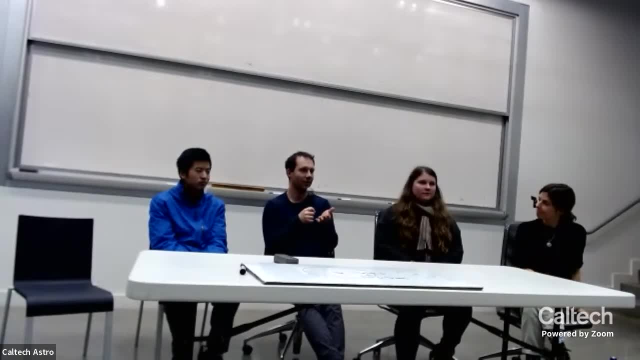 stars. they die early, right. so what do you have ending up in the end after five, six, seven million billion years? is the Loma stars right? and so you change your kind of distribution of energy from the blue to the red right. um, and now it's funny- um, so you have the redshift right. 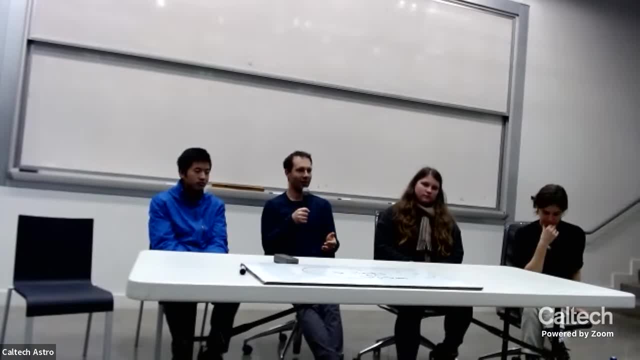 which tells you the distance to a Galaxy. you have old Galaxies that are also red and in addition to that you can have dust in your Galaxy. that's also making a Galaxy red right, so great you can go home right. so this is basically the problem, right, and so the redshift. you can really just look at the. 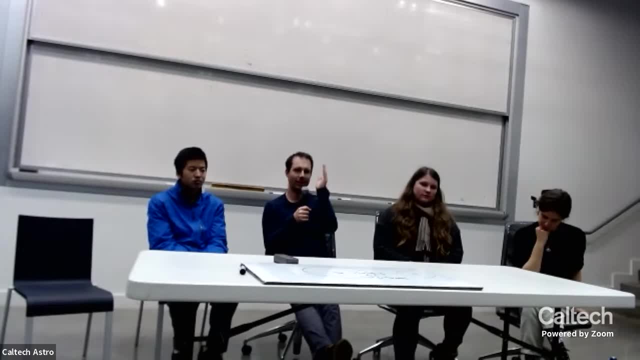 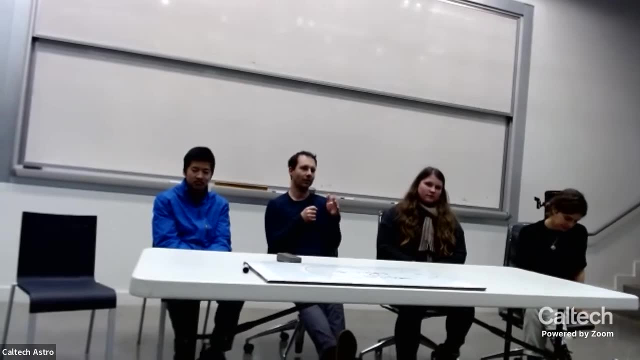 emission lines, how they are shifted to the red right. so that's, that's basically 100. you get this um and then the what how usually look at or how, how does your Galaxy is? you do this also from the continuum right, so if the Galaxy is more red, 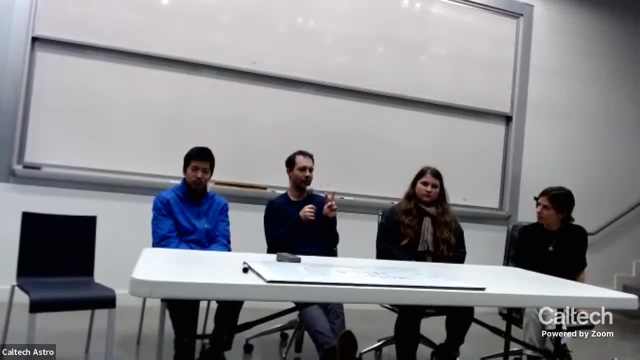 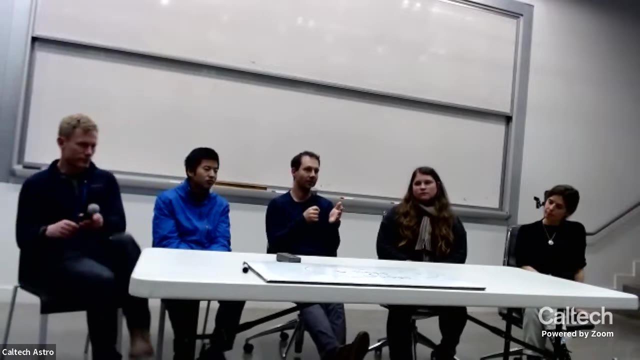 um, then you have, you know, more dust, but you can also use ratios of two emission lines. so, for example, there's the hydrogen line, H Alpha, at 650 nanometers, and then there is H Beta- it's 480 nanometers. and so the ratio of those, those two lines, is fixed by quantum physics. right, it's a. 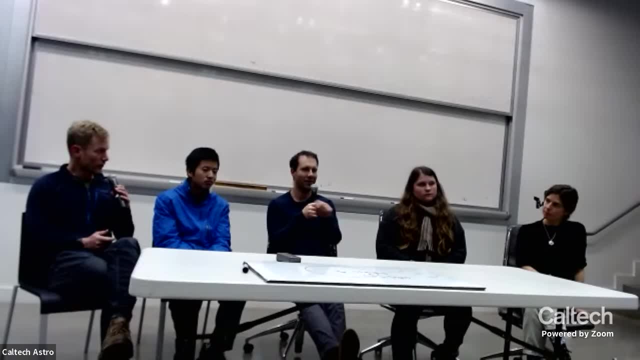 factor of 2.86, the brightness of those two lines. the brightness of the two lines, yes, right, so, and? and H Alpha is usually brighter by two point, by a factor of 2.86, right, but if you have dust, you attenuate the bluer. 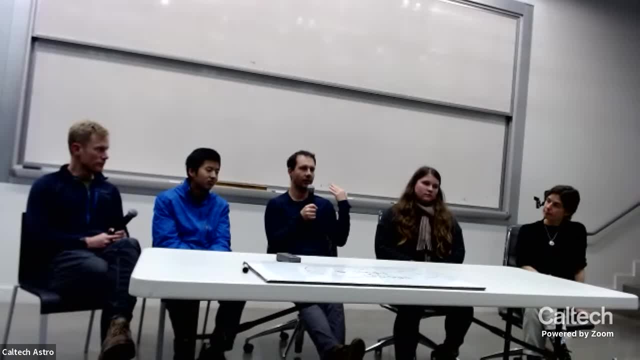 line, because what does basically does? it's like when you look at the sunset, it basically scatters the blue light and that's through the red light, right, so it's a reddening, and so your, your H Alpha line might be brighter by a factor of three instead of 2.86, right, and from that you can actually measure. 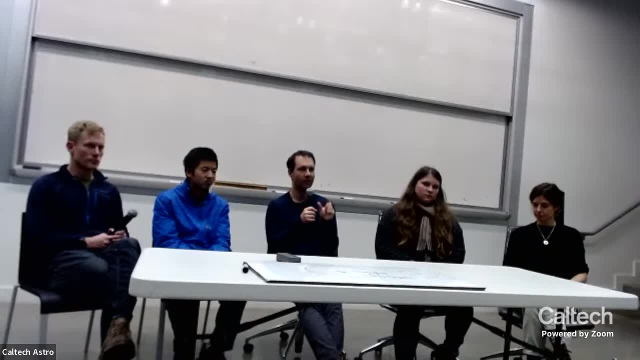 pretty precisely. what is that? dust content? or the dust attenuation of the Galaxy, right? so now you have registered and dust, right and now. the only thing you have now to do has to fit the whole thing with a model. so you have different models of different ages, right, you fit it to to each of the photometric. 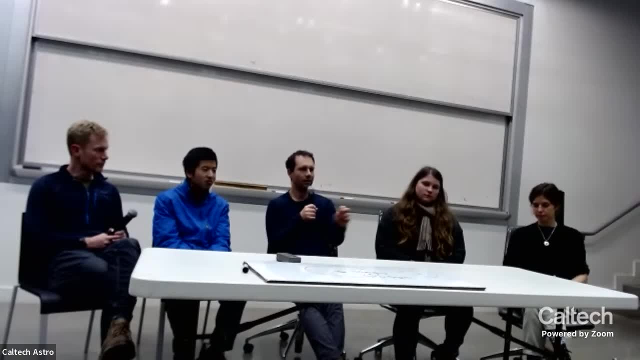 point from the low blue wavelength to the red wavelengths and you basically have prior, because you already know the dust and the redshift and that way you can figure out the age. um, so hopefully I confused you totally, but basically what I want to say it's, it's a, it's, there are degeneracies all over right, so it's really hard to get the age of a Galaxy, um, yeah,